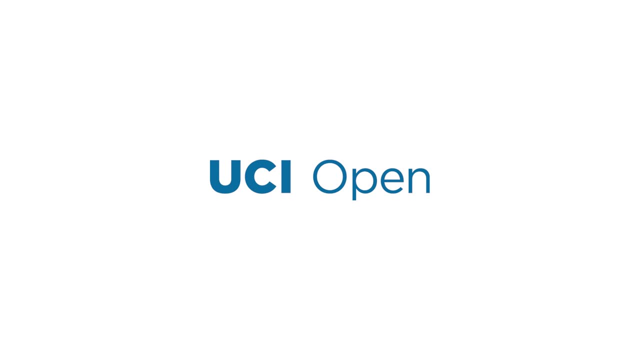 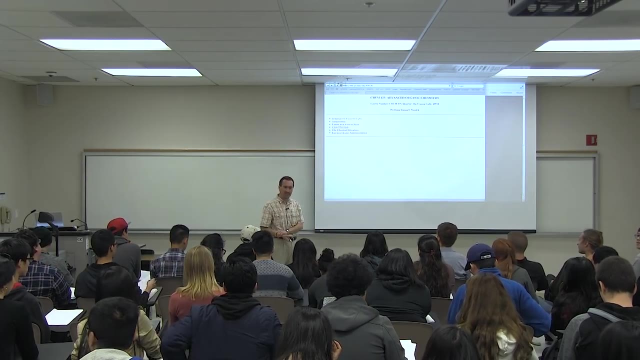 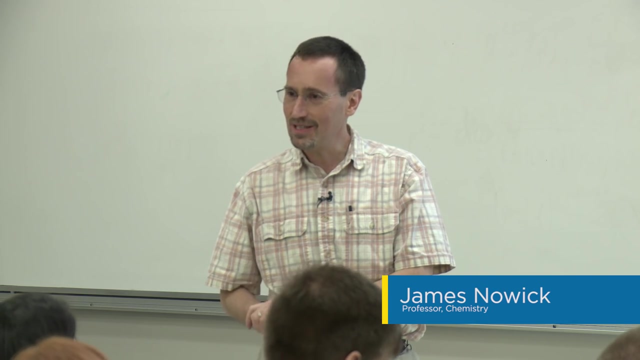 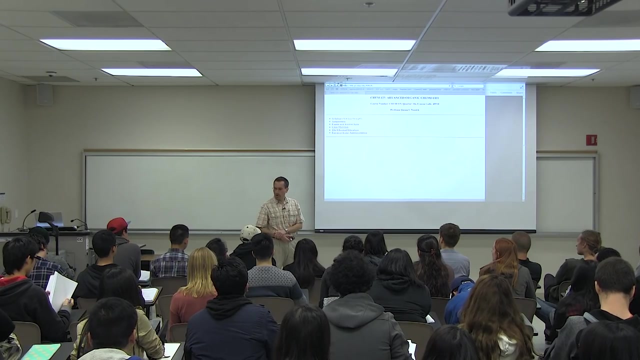 Welcome, welcome, welcome to CHEM 125, Advanced Organic Chemistry. So I am really excited to be here this quarter. This is a fun course to teach and it is a fun course to learn. I want to start today by going over the syllabus and a little bit about my expectations for the class. 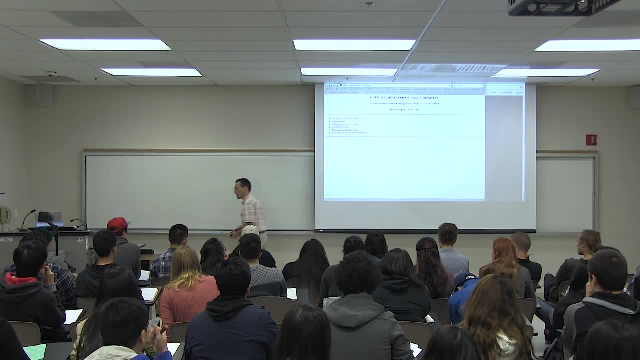 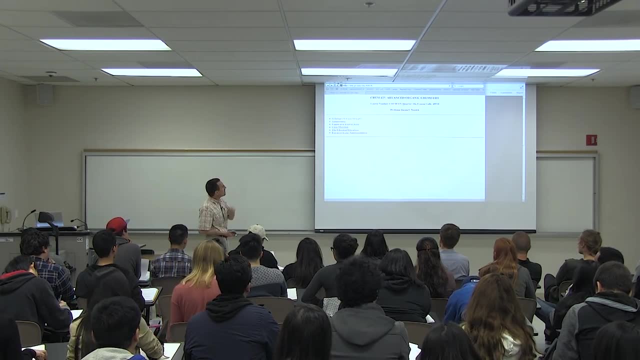 And then we're going to dive right in with chapter one of the textbook. So this is the website for the class. I presume all or most of you have already checked this out. We're going to have all of our homework assignments here. You'll get your exams and answer keys. 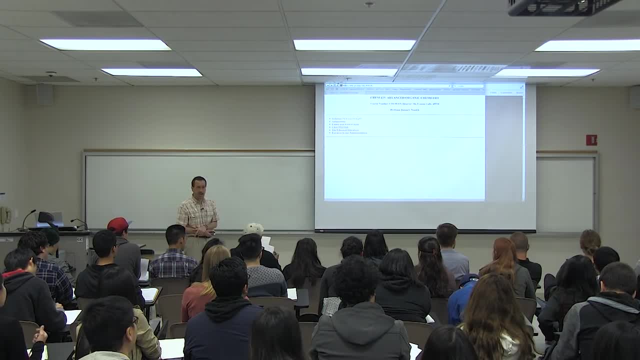 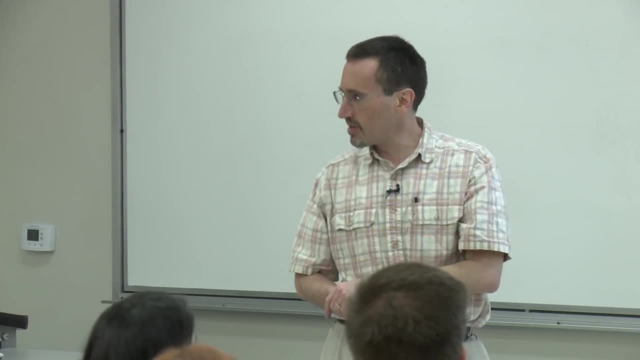 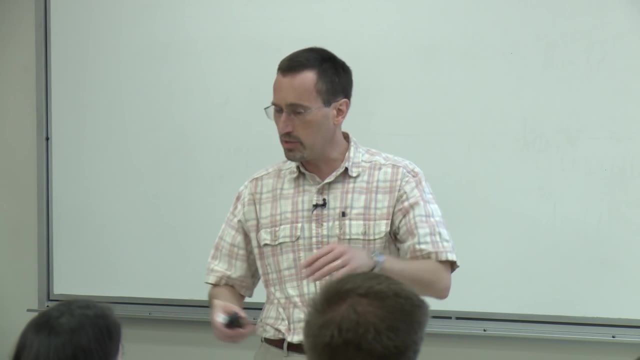 I'll post various materials for the class, like those handouts I directed you. We also have some links here. You may have noticed the video camera is in the back of the room. One of the things that I've been doing is putting my classes on available on YouTube and, I think, iTunes U. 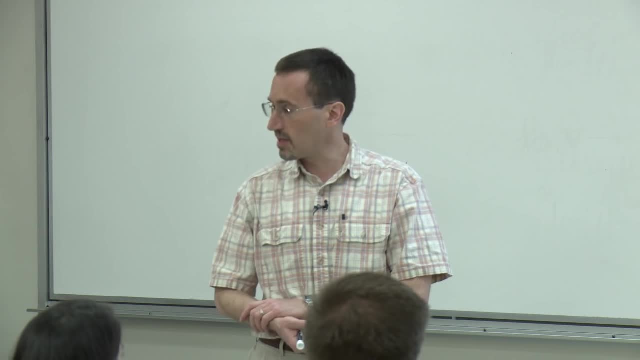 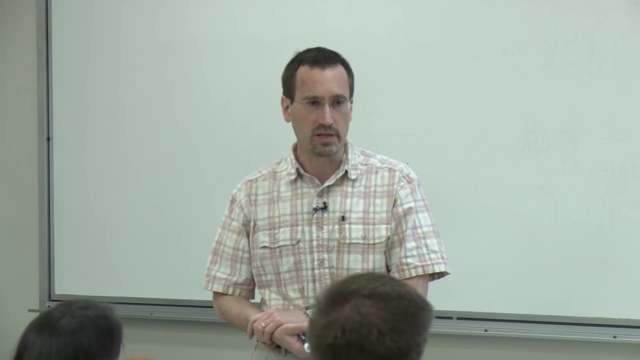 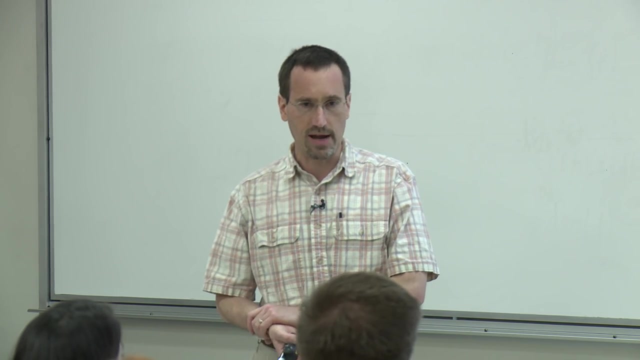 And basically not only to us but to the whole world, which has been really, really fun, Because I get to hear from people all around the world and they benefit from it. But mostly it's a chance for you to go back in time. It's a chance to go back if you miss a class, if you're out sick and you don't want to share your flu with us or whatever. 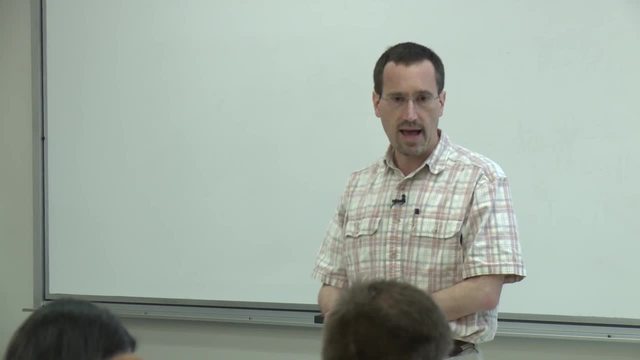 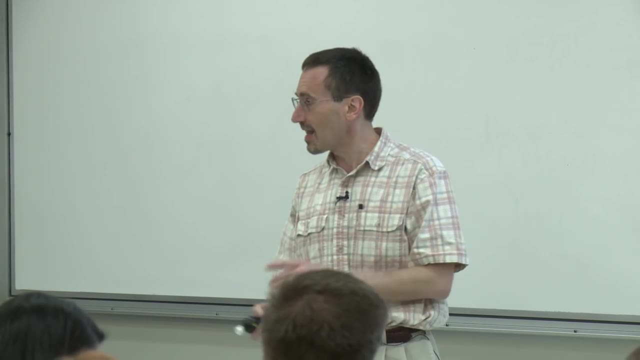 Or you simply didn't pick up something. It's a chance to go back. The videos will probably be about a week after the class, So a little bit later than you know. don't miss class. I mean, you know, come here. Seriously, it's a good place to be. 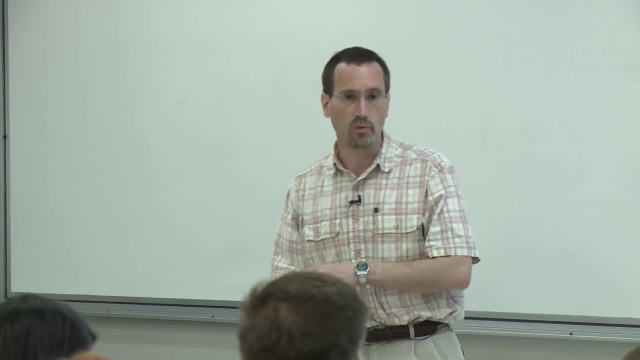 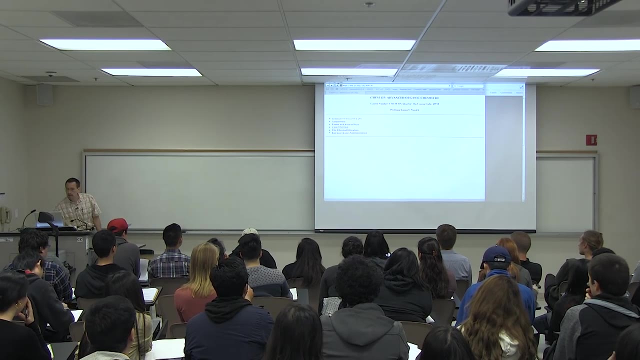 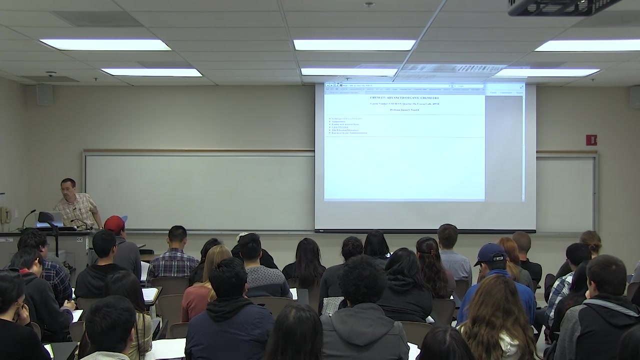 But it's a good chance to catch up or, if you want a way of enhancing your notes, to do that, All right. I want to start by going over the syllabus here And, oh yeah, and I'll put a link to the videos, probably right above class materials or right below class materials. 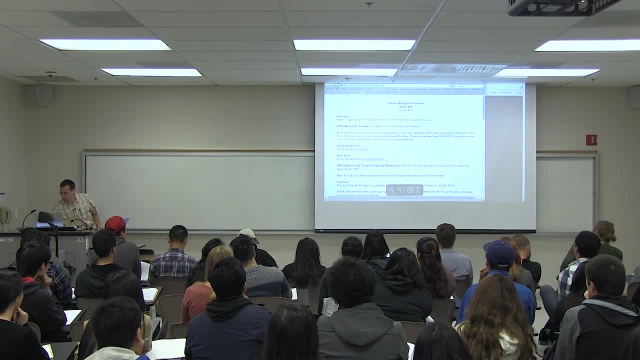 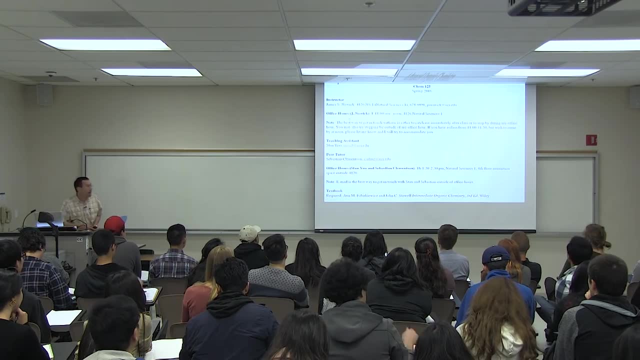 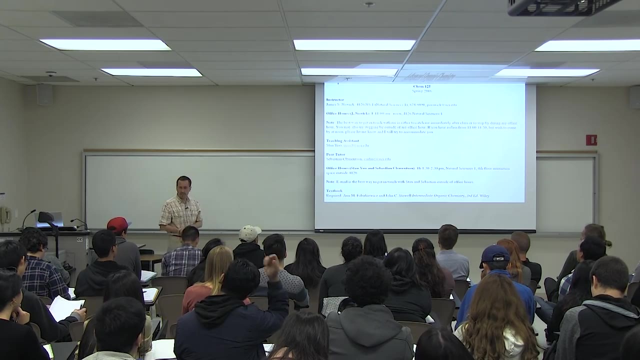 Somewhere on the page. Anyway, I want to start by going over the syllabus here And let's see All right. So here I am, Professor James Nowick. I set some office hours And I mean honestly, you can come by and catch me at other times. 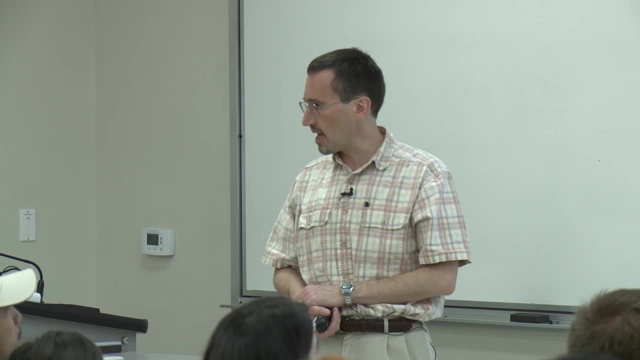 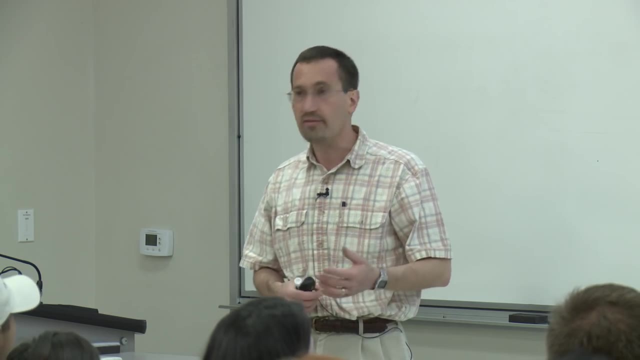 I'll make myself available then You can catch me after class. If you're really desperate, you can phone up to my office and say: hey, are you in your office? Can I come by? I've got a burning question. A bunch of ways to get in touch with me. 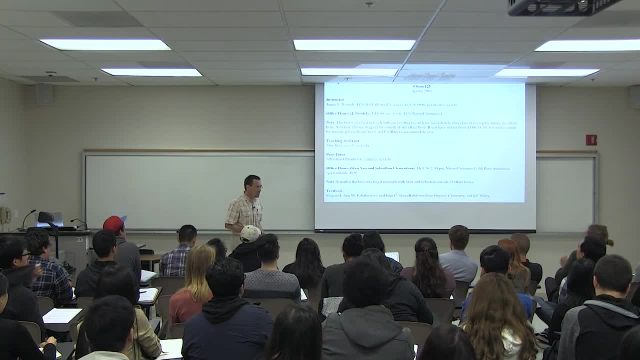 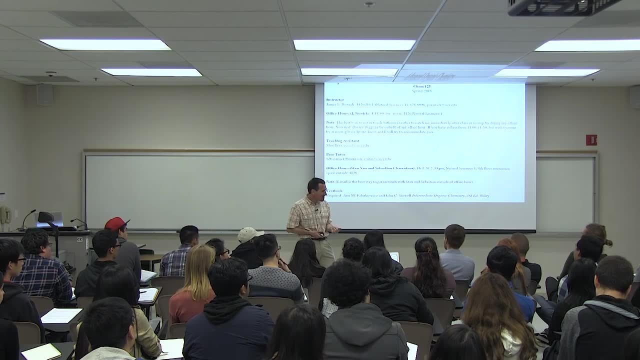 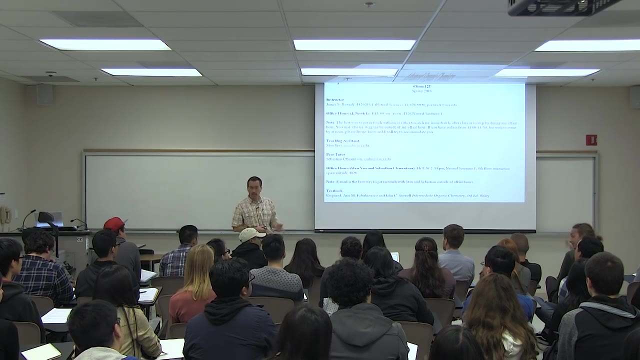 We have a teaching assistant, Stan Yu, who I have personally selected. Stan has been asking me- He has been asking me for the past what year- whether you can teach with me in this class- And also a peer tutor, Sebastian, is spending a year in my laboratory. 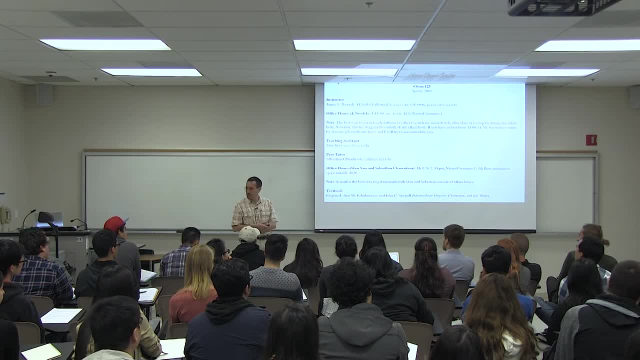 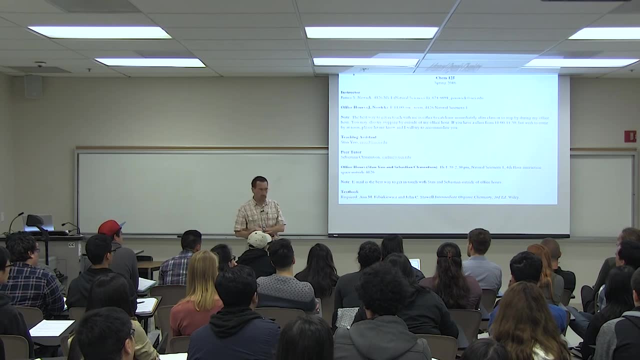 Meanwhile acing our graduate courses and putting our graduate students to shame. And Stan and Sebastian are going to work as a team as teaching assistants, with the discussion sections and having their own office hours and so forth. All right, So we've got a few things here. 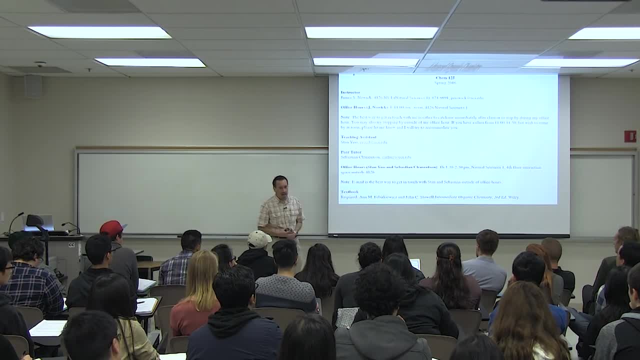 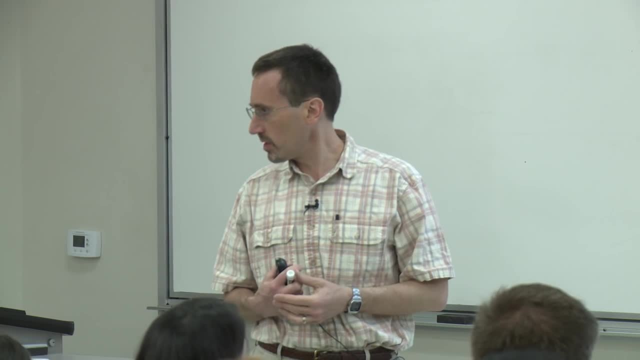 So we have a few things here, So I'm going to go over the textbook for the class. I have loved this textbook for a long time. I taught Chem 125 a bunch of years ago And the textbook was the second edition by Stoehl. 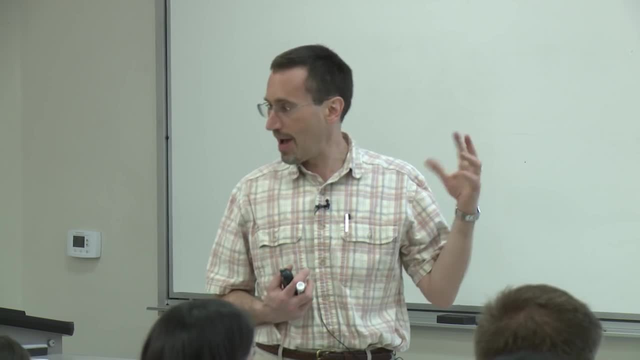 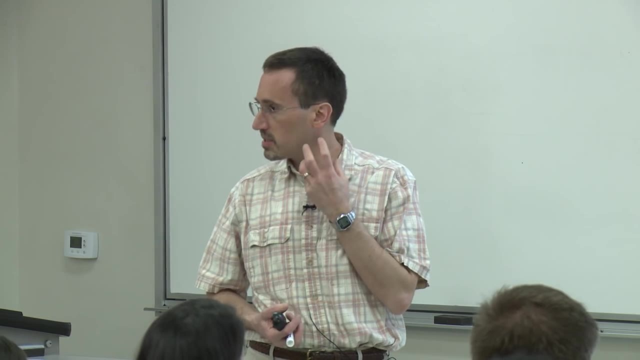 And it was already getting old, back maybe a decade or 15 years ago, And I was really sad because it was just a great book. I mean, this book is concise, It's readable in a quarter. At the same time, At the same time, it's terse. 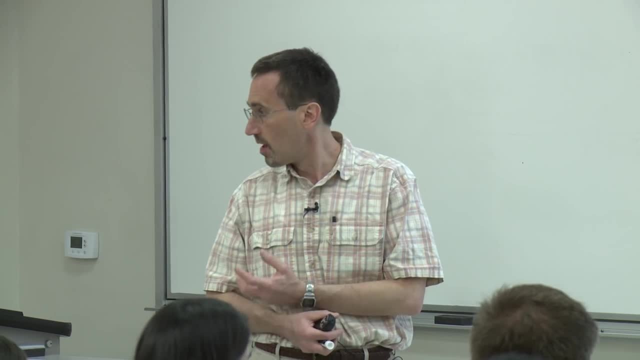 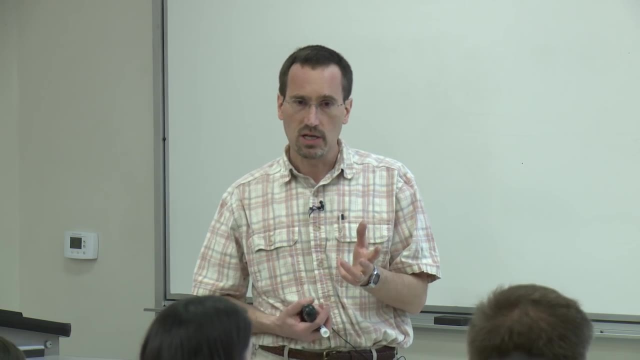 I mean, it doesn't waste your time with stuff you should know already. And it's just a lovely book, Fits in your hand, everything else, And it was getting old, And so when I found out that in 2015,, in the spring of 2015,, 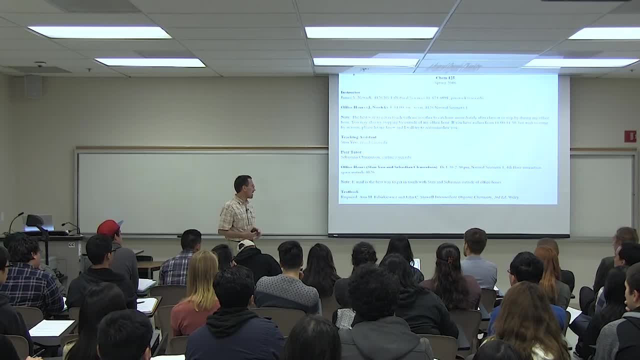 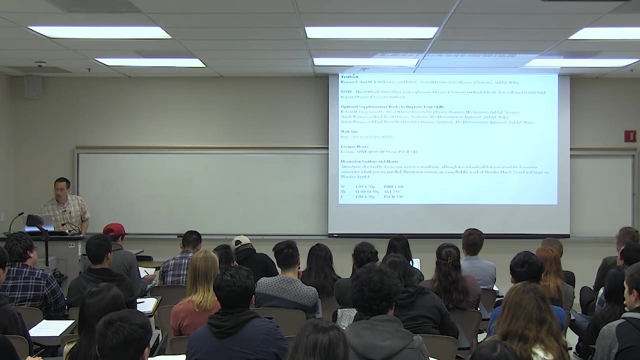 a new edition was coming out where a new professor, Anne Faberkowitz, had come to revitalize the book. I was so excited And I was really glad. I kept pestering the publisher to get a copy to me And I have not been disappointed. 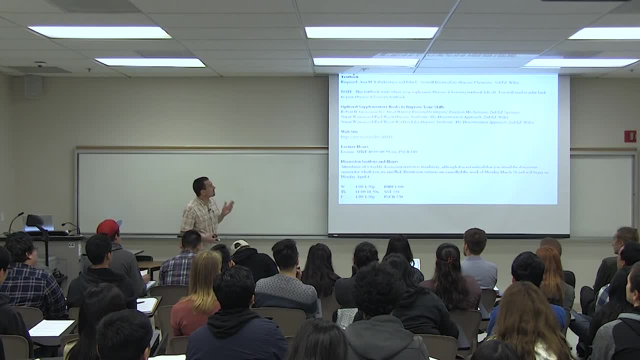 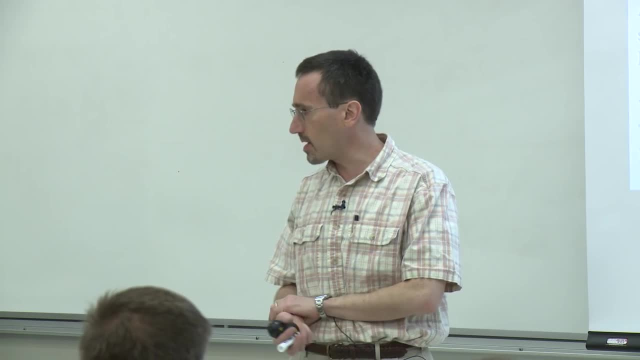 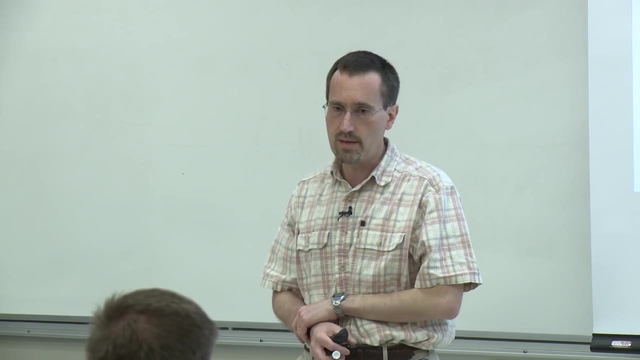 So, as I say in the syllabus, this textbook really starts where your sophomore OCHEM textbook left off, And I think if you've already read chapter 1, you'll see that basically everything it's talked about with nomenclature basically goes way beyond. 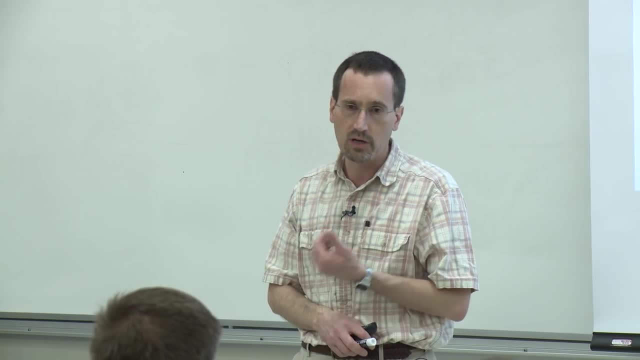 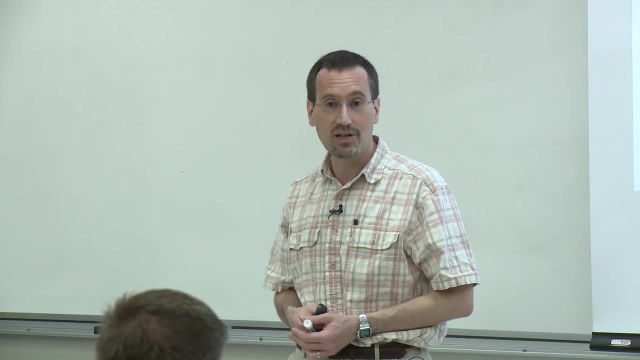 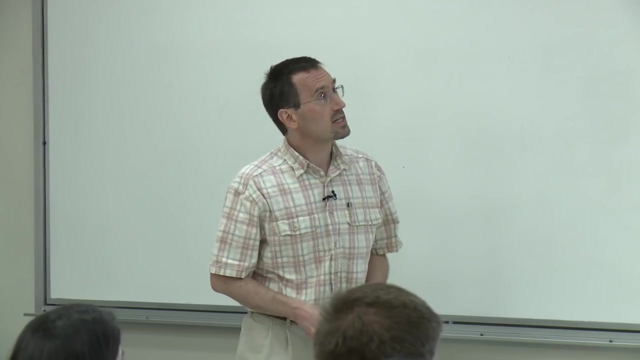 And we're going to see this in all the different topics we cover- Synthesis, reaction mechanisms and so forth, which means your sophomore organic chemistry textbook is your friend to refer back to on all sorts of topics you might be a little bit rusty on. 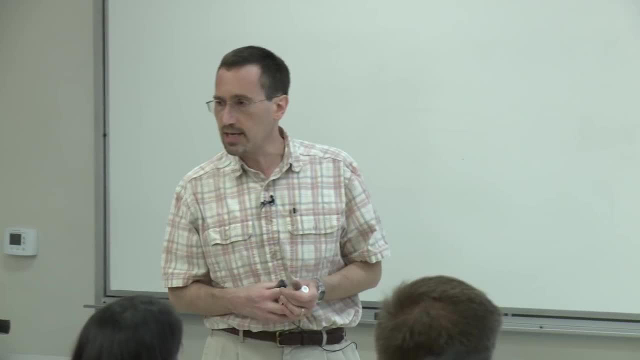 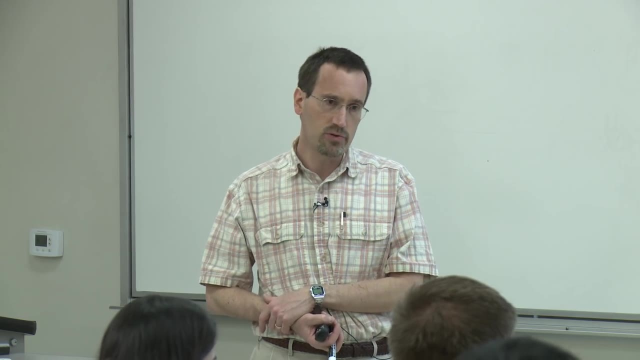 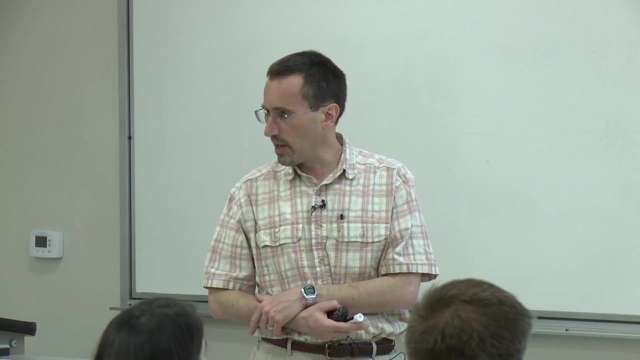 Honestly, I think the textbook and the problems are going to keep you pretty busy this quarter. But I know some textbooks, some supplementary books that I've used, that graduate students in my laboratory have used, that undergraduates have used, and they really love them. 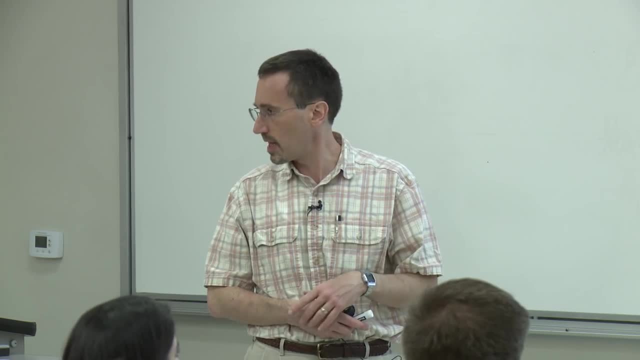 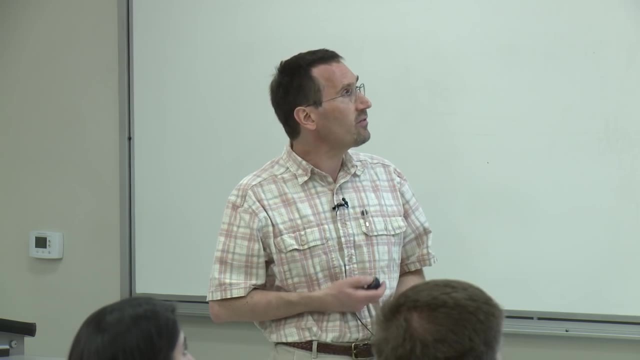 These are textbooks. They're not remedial. I've got textbooks to help. Well, the first one can help you out if you're a little fuzzy, But these are books to help really cement concepts if you're going on organic chemistry or if you just want more. 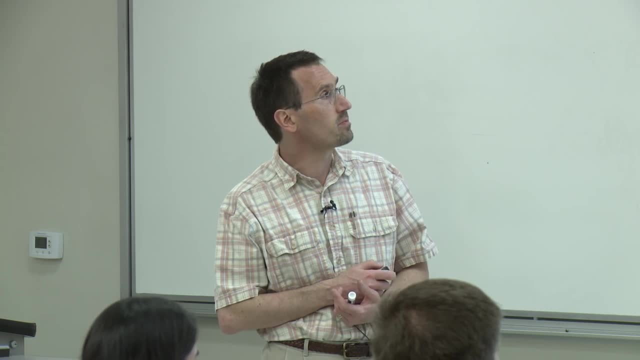 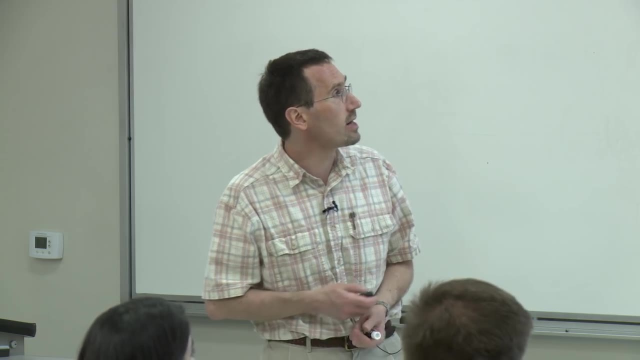 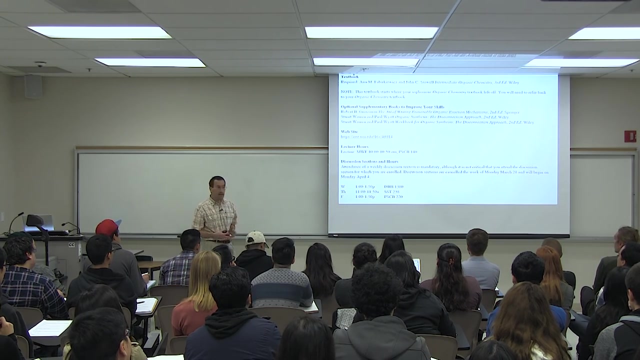 Every graduate student I know has loved Bob Grossman's book The Art of Writing Reasonable Reaction Mechanisms- Great for Curved Arrow Mechanisms and Paracyclic Reactions. There are two synthesis books, a textbook and a workbook- that are a lot of fun too. 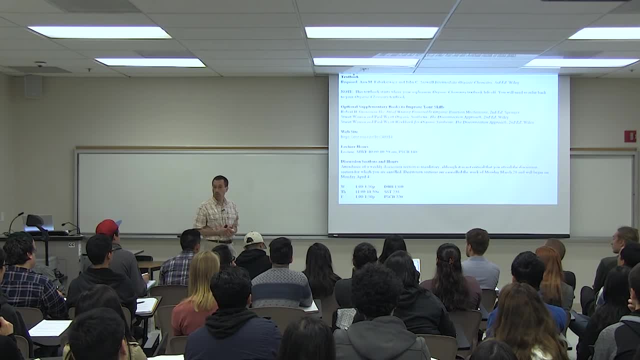 And I'm hoping that all of the problems- I mean I hope you like working puzzle problems, because these really are making you think and getting you to think about how reactions occur and how you build molecules. And that's the same for the problems in this book. 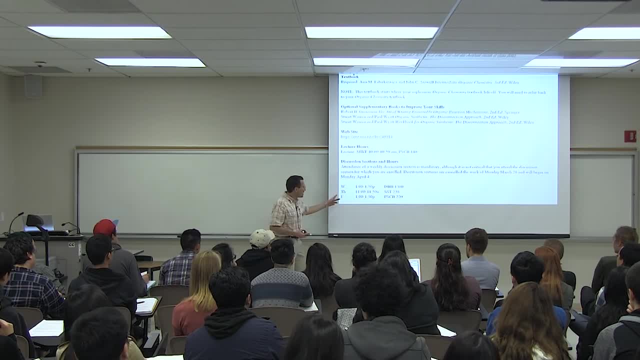 OK, we've got the website, the lecture hours. There are three discussion sections. They should all be pretty similar, so it doesn't matter. It doesn't matter which one you come to, but you need to come to one, And we're going to go over things like homework. 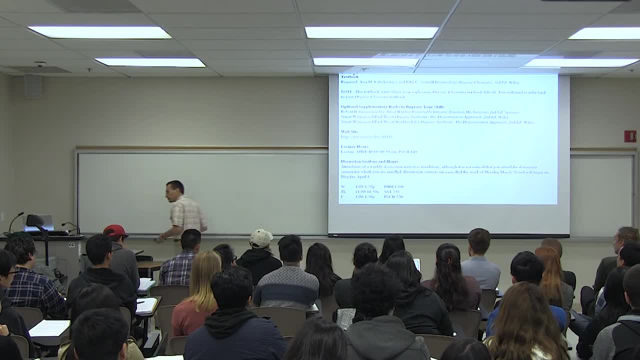 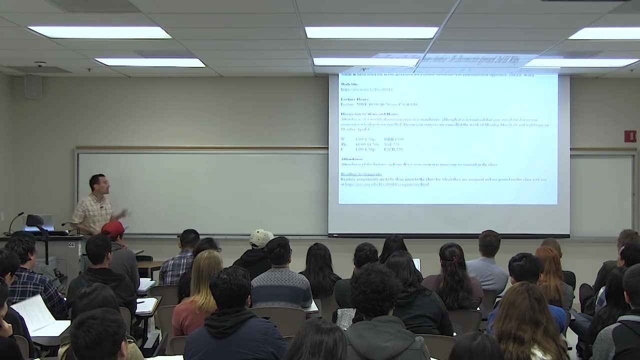 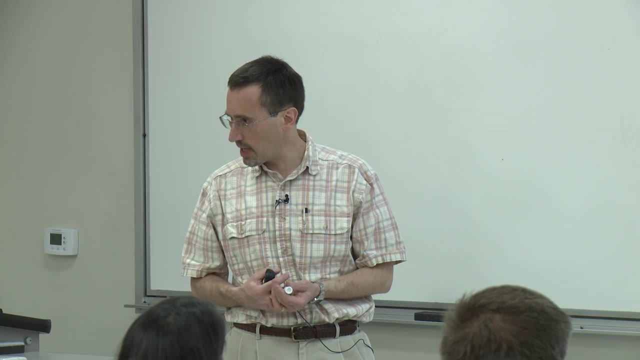 and maybe get some extra problems in there. All right, basically, as I say here, coming to class really is necessary. The textbook is dense, The textbook is challenging, And what I'm going to try to do is make sense of it. 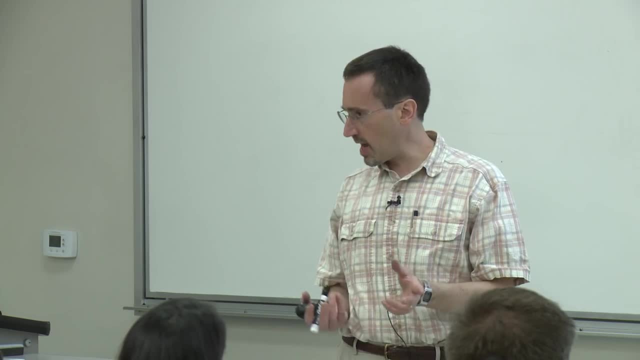 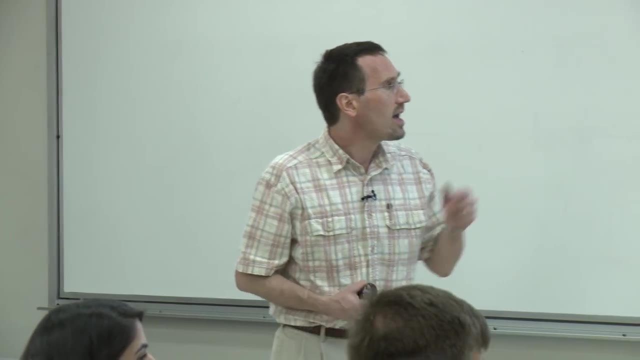 I like this text very much. This textbook is 10 chapters. We're going to do 10 chapters in 10 weeks. First two chapters are really short. We'll do them in one week And I think you're going to get my spin from the class. 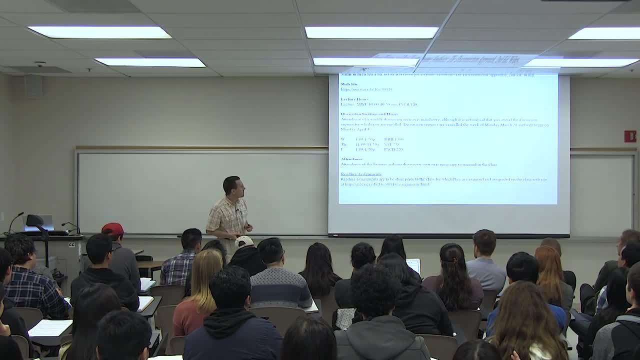 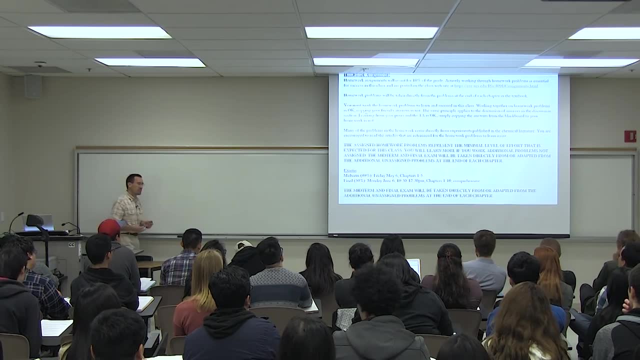 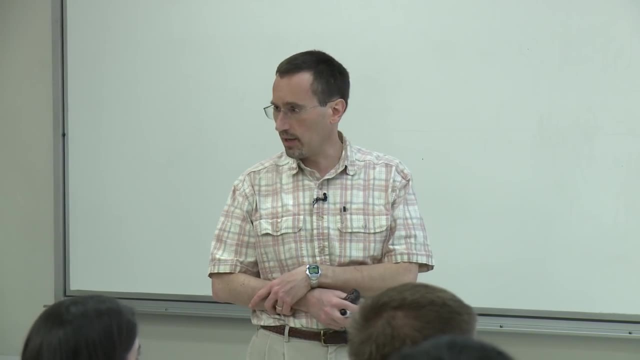 I'll be listing reading assignments as we go along. I may already have listed all of them, and I will then list homework assignments from the chapter. All right, this particular organic chemistry in general, but in particular this class, is something that you learn by working problems. 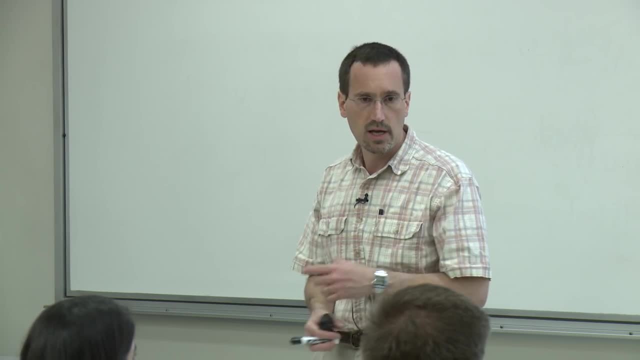 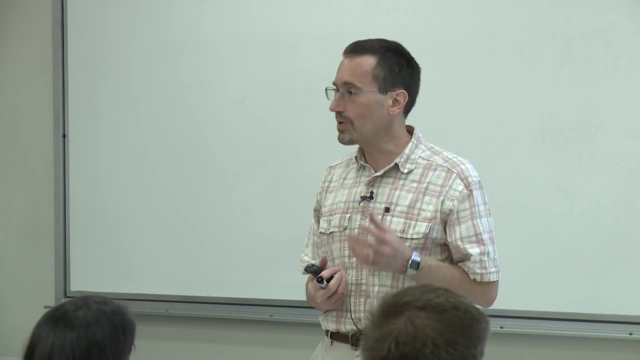 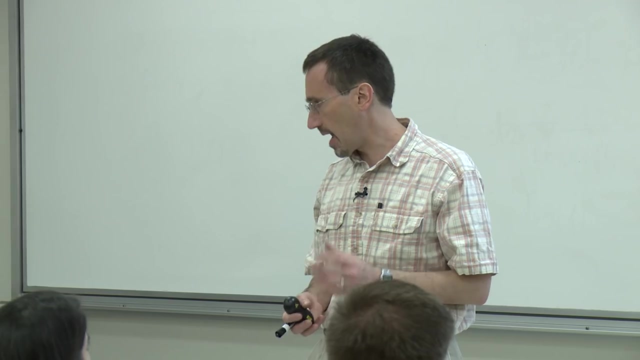 And you also get to see the level of expectation that comes from working problems, And that is the most important thing for learning. In other words, you cannot master organic chemistry, and certainly not at this level, without actually working problems. So I've worked it first. 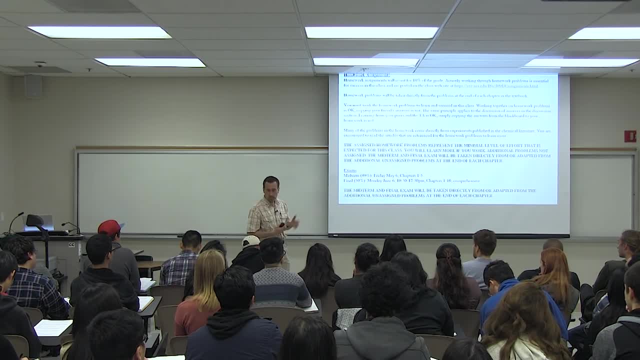 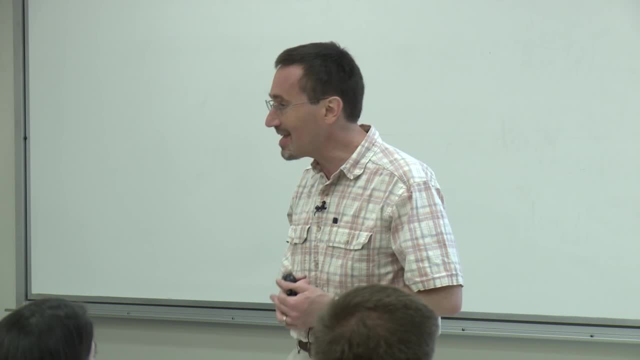 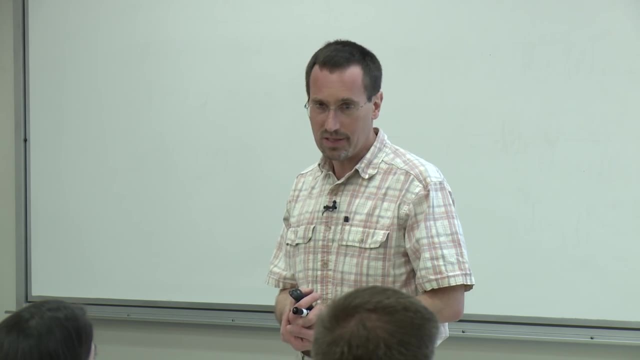 Homework set. I will be working all of them. I have worked in the older edition. These are fun. These are actually fun: tickling, challenging, engaging problems. It should take you some hours to work these problem sets, And they should be, I'll say, for chapter one. 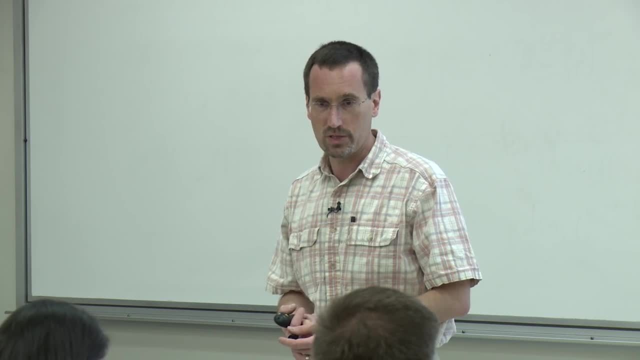 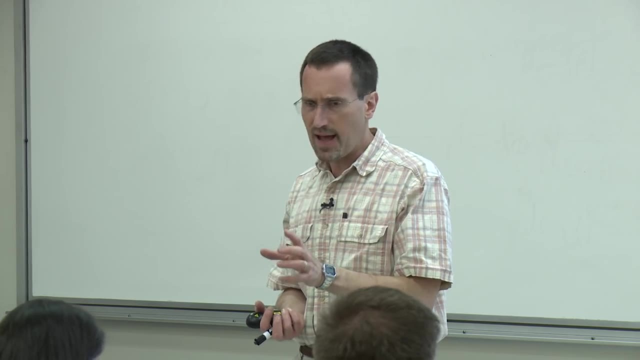 I look it's basically go back to the chapter and reinforce things. I read chapter one and every line I read. where I saw a structure on nomenclature, I went back And it's like, OK, the answer was how they got it. 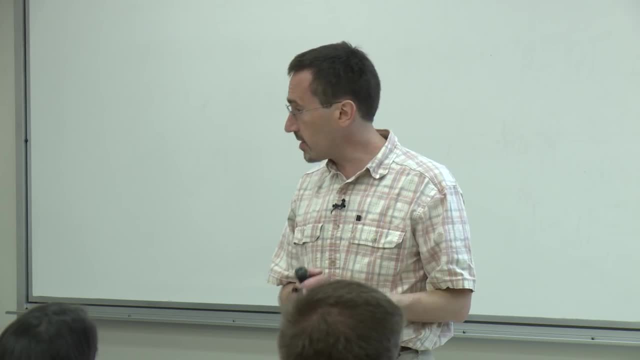 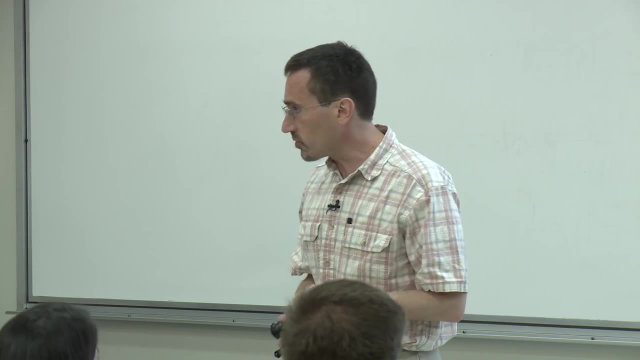 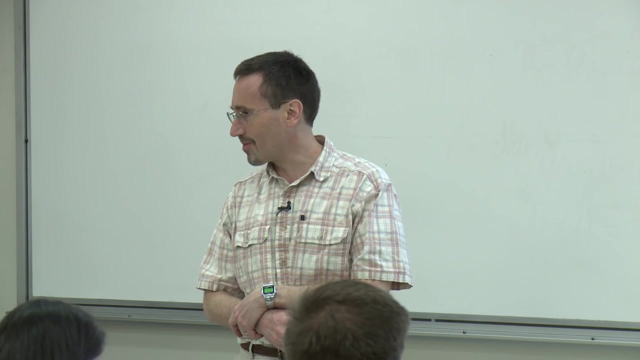 was right here And I sort of actively engaged with it. And then the homework problems. it's the same thing with that. You basically go back and you actively engage. Chapter two: I've already worked most of the problems there. It is like a scavenger hunt in terms of finding information. 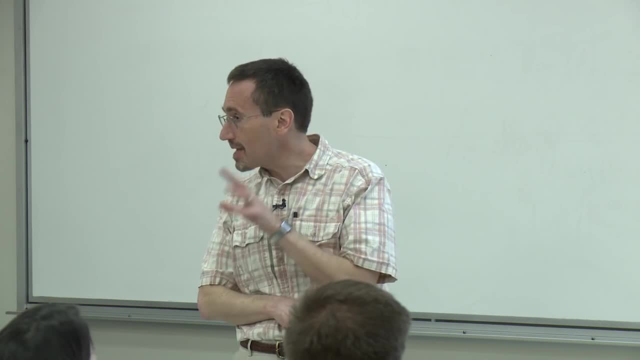 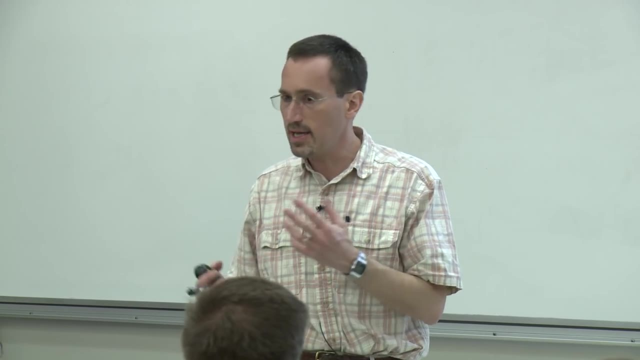 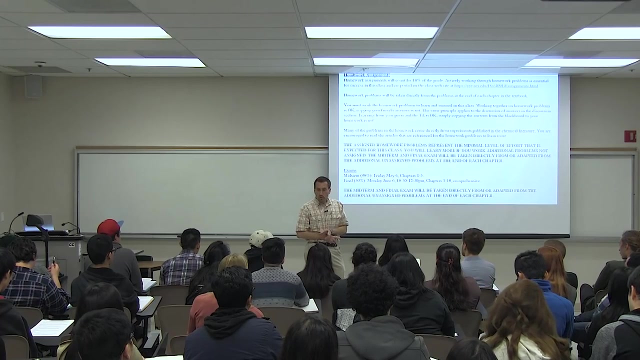 and learning the chemical literature And, as I said, this is taking us beyond where we started in sophomore: organic chemistry. This is making us realize that chemistry is a living, breathing field actively under development. Most of the remaining chapters are going to have not an answer key but references. 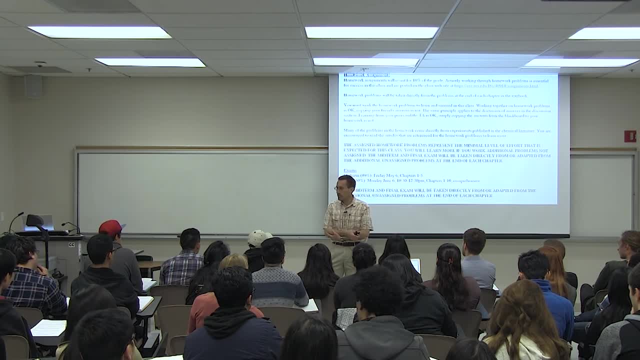 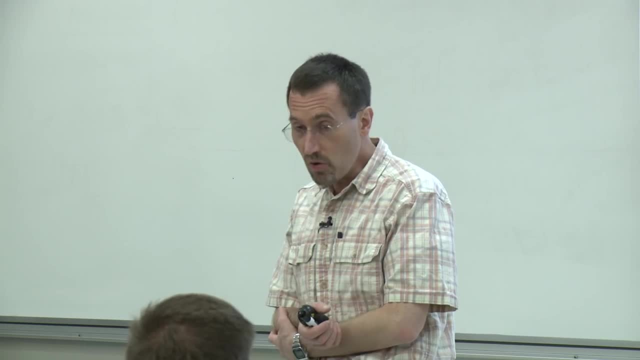 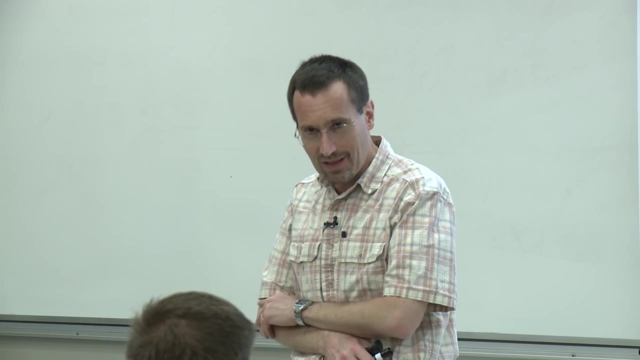 to the primary literature, references to articles in Journal of Organic Chemistry and Journal of the American Chemical Society and tetrahedron letters and so forth. Most of those papers don't have a quote answer. But if you read those papers along with work, the problem. 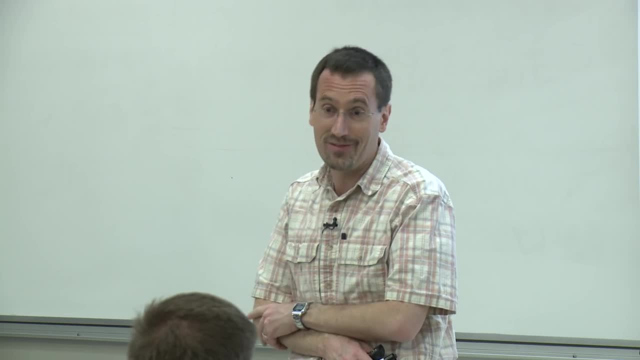 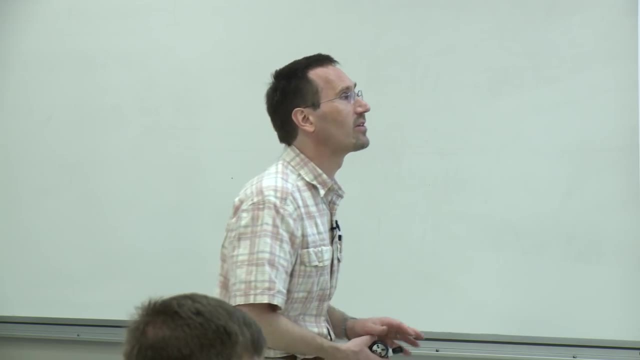 and read or skim those papers, you will learn a hell of a lot And I've done that in the course of my education And this has been fun and engaging, a completely different experience from sophomore organic chemistry. The textbook is going to the course. 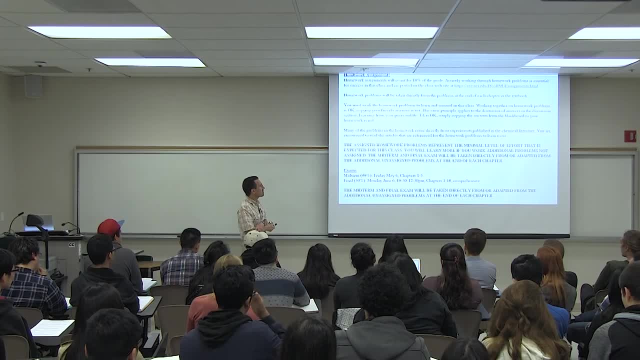 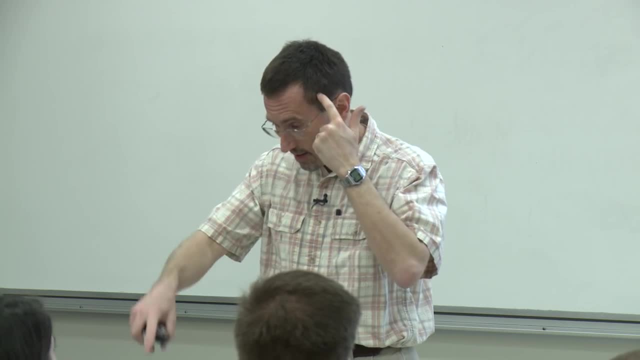 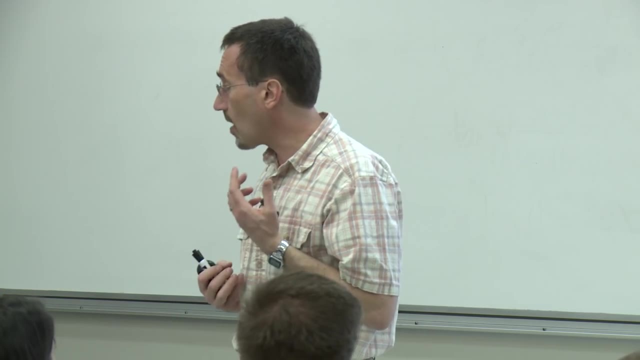 is going to be very problem focused, And what that means is things have to get from here into here, onto your paper, And that means actually working the problems At the same time working together. comparing answers can be a good thing. I approve of that. 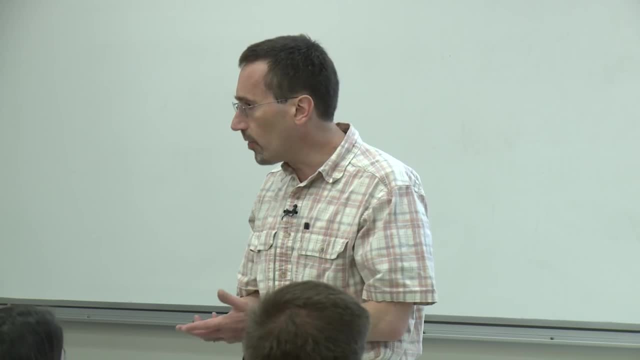 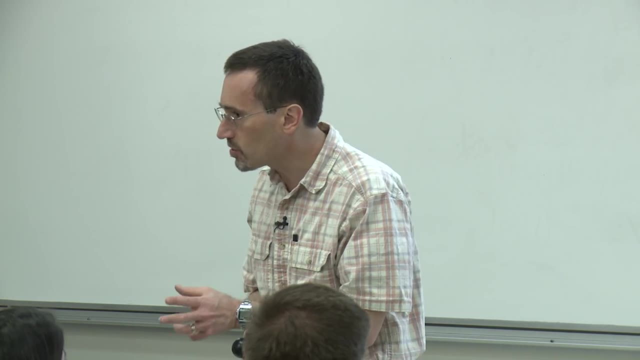 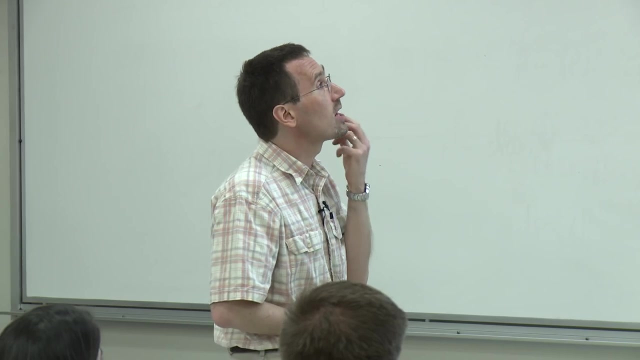 Talking to the teaching assistants can be a good thing, But ultimately the homework isn't about getting the right answer. It is about that process of transforming your thinking and your understanding so that you can actually really generate this knowledge and master it. So let's see. 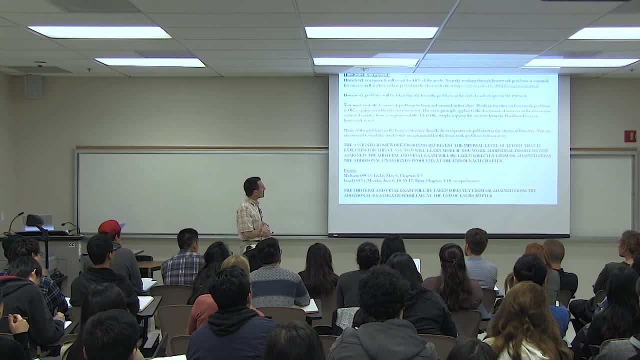 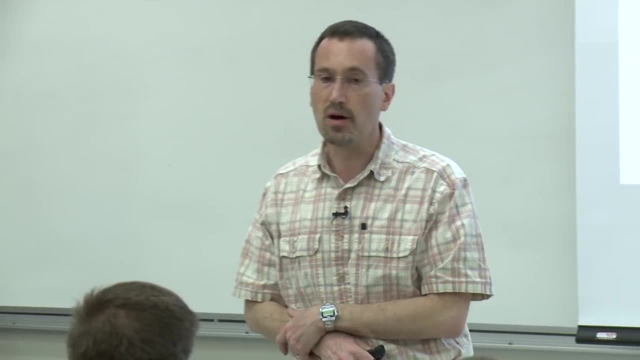 One of the things that I thought about this is, as I say, I like this textbook. I really do, And the homework problems I've assigned are sort of the minimal minimum for mastering things. It's sort of the baseline. 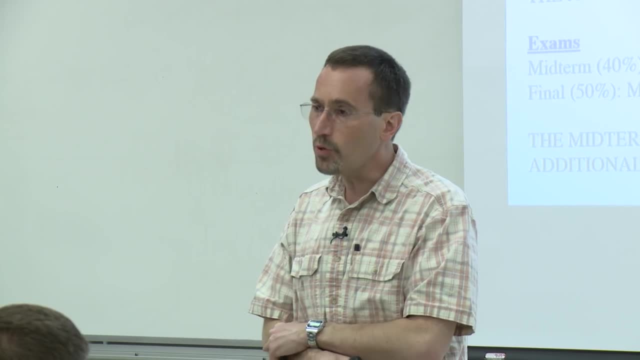 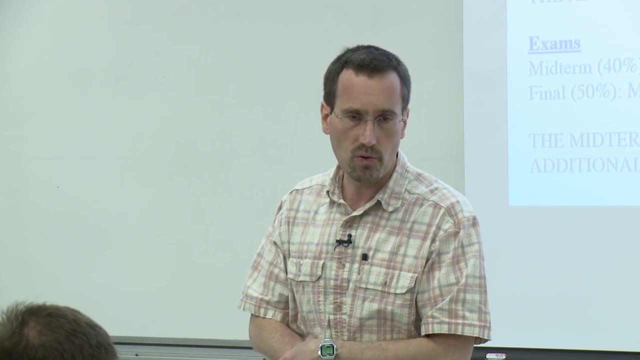 There is so much more to learn. The textbook is, For the most part, pretty sane in its number of problems, pretty non-repetitive in them, which I think is good. In other words, they don't get boring. And so what I'm going to do? and again this: 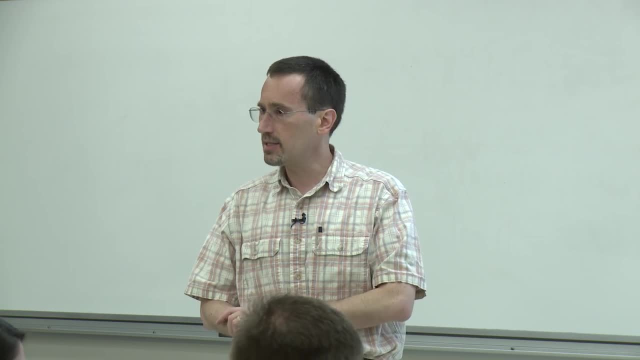 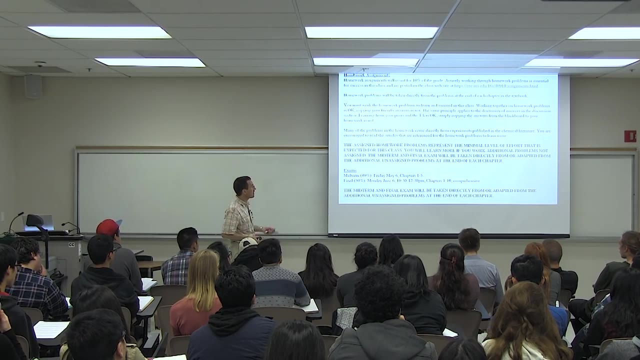 comes right back to the way I learned a lot of chemistry is the more problems you work, the more you're going to learn, And I'm going to reward you for that. Right now, my plan is basically all of the exams and problems. 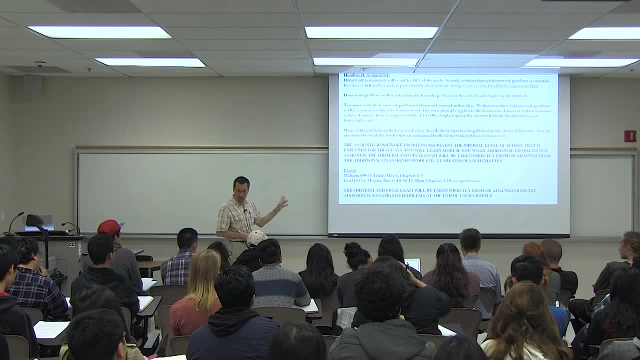 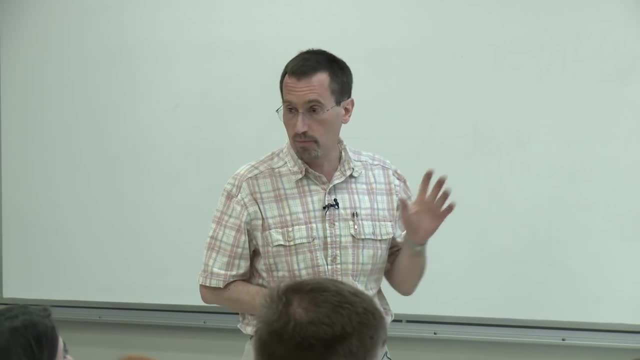 are going to be taken directly from the homework or adapted from it, meaning made in a more suitable format for an exam. I'll let you know if that changes, But right now I'm pretty gung-ho on that, which means you have the potential. 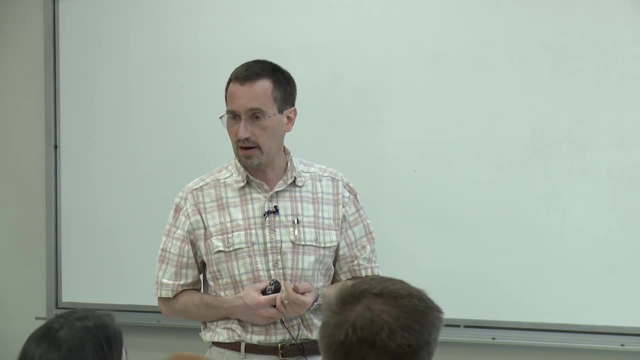 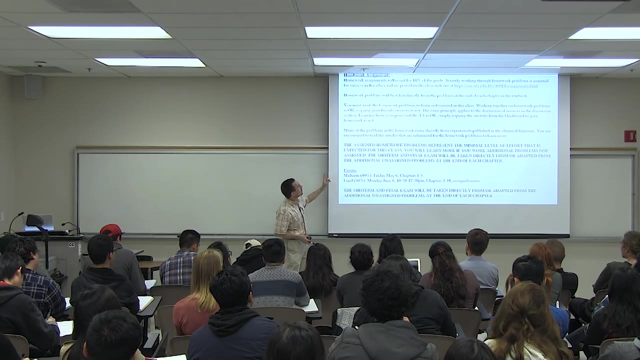 to go into an exam having worked every problem there, and for you it to be super easy. We're going to have two exams, so we're going to have homework. You've got to hand in the homework And I think I'm collecting the homework at the end of class. 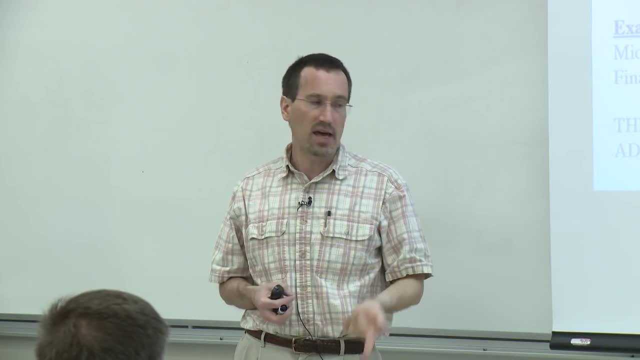 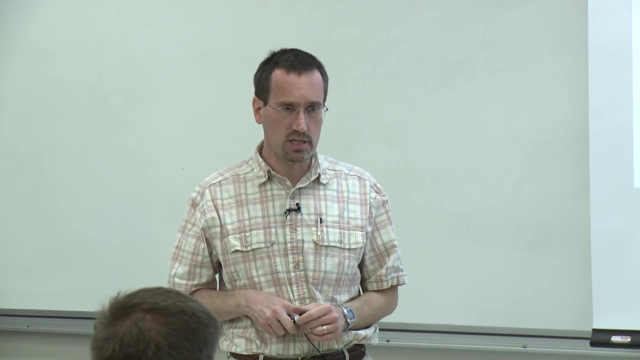 We're going to work on days that I've noted. I think I'll. We'll probably do it with a box or something in class For getting the homework back. I'm still thinking about the logistics. My inclination is to basically have them go back. 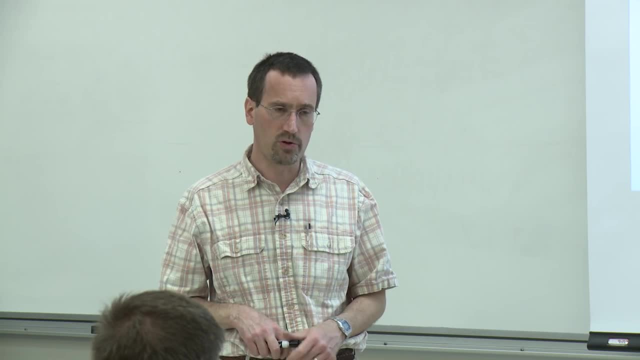 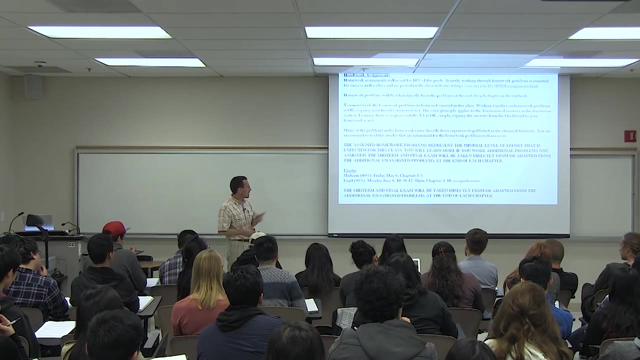 in discussion sections. maybe if we can set up some folders and alphabetize, It may get too chaotic, in which case we'll figure something else out. OK, so that's 10% of the class. The midterm is 40%. We're going to run midterm. number one is chapters 1. 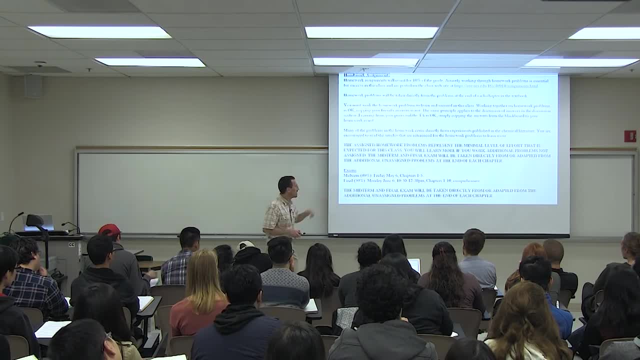 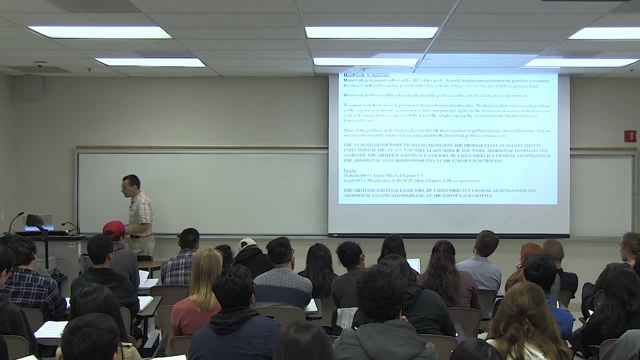 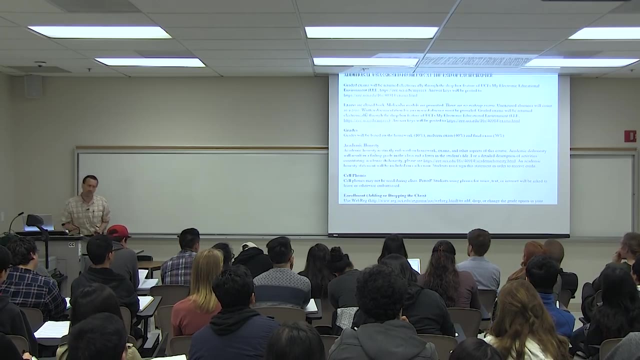 through 5 on Friday May 6.. And then the final is Monday, June 6.. And it's going to be 1 through 10 comprehensive, All right exams. I'm a little more clear about the mechanics And we may end up doing. 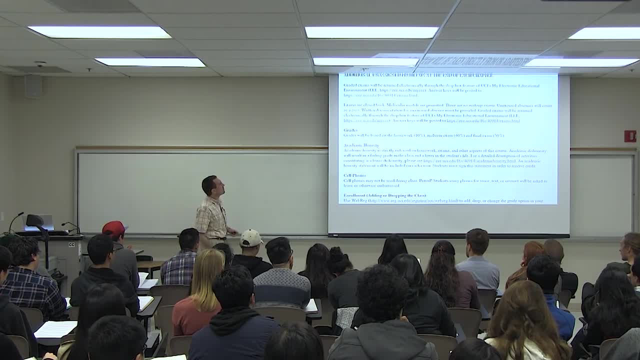 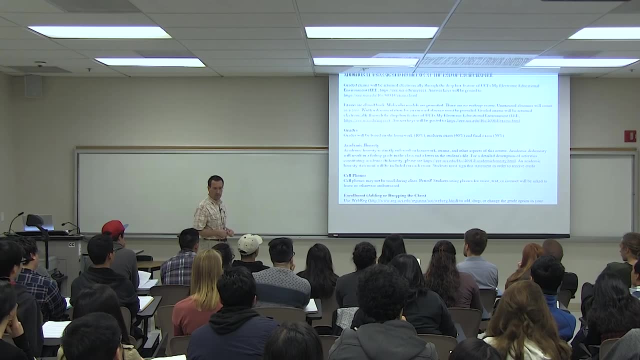 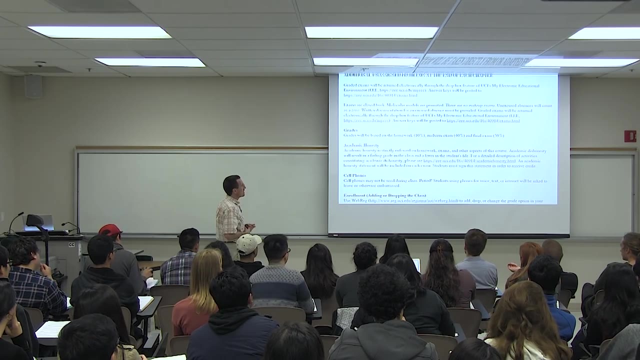 I probably won't be able to do rapid return for the homework, so we'll figure that out. Anyway, the exams will be through the same electronic exam return feature that you're already familiar with. We're going to have answer keys up closed book exams. 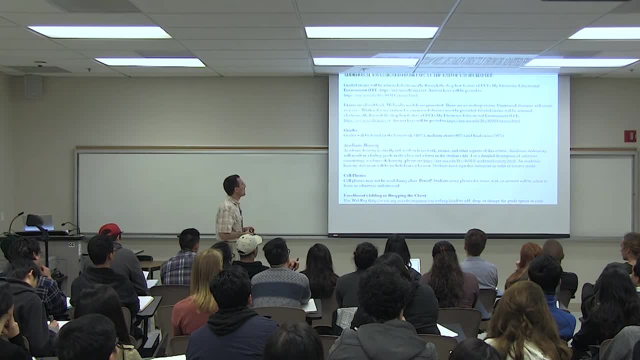 no make-up exam, unexcused absences counting as a zero. if you're going to miss an exam, like if you're sick, I need a note from the doctor. basically, Let's see what else. OK, don't cheat in that class. 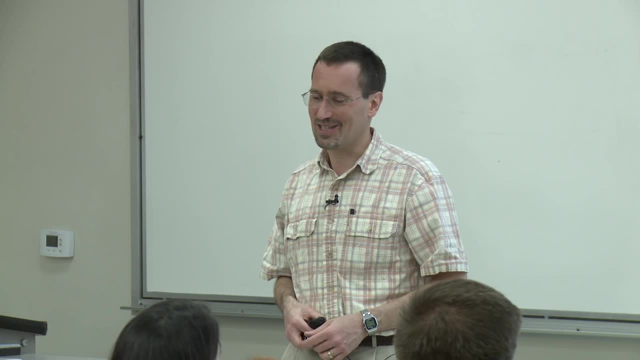 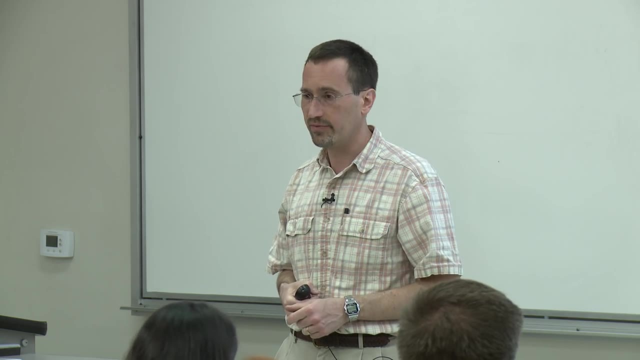 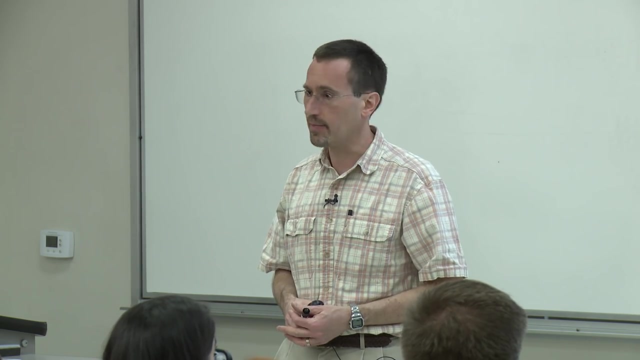 That just screws up the whole class, for I mean it just sours it unbelievably And unfortunately, at least in the sophomore class I have. I have failed a number of students. There is a policy here of basically any academic dishonesty results in a failing grade in the class period. 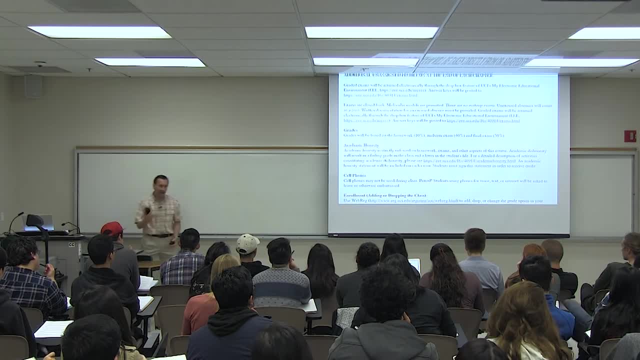 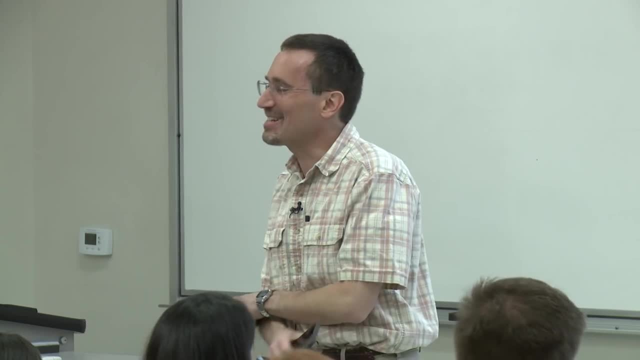 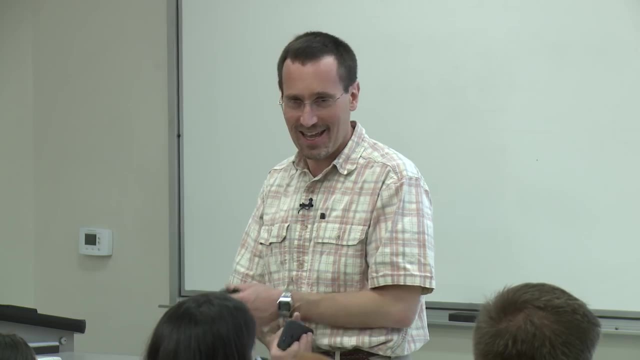 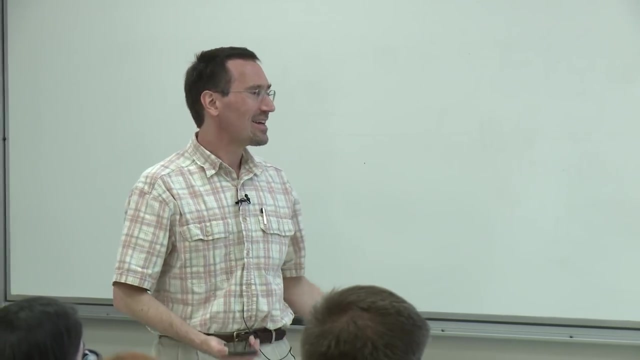 All right, cell phones. I love my iPhone, But I absolutely cannot talk intelligently with beeps, chirps, rings, Texting, Turn it off, put it to sleep. If it beeps, I'll send you out, or otherwise embarrass you. 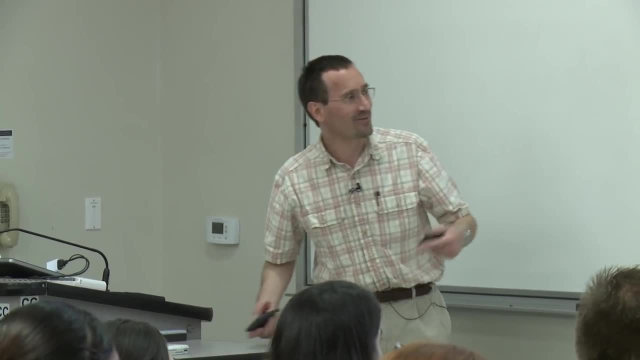 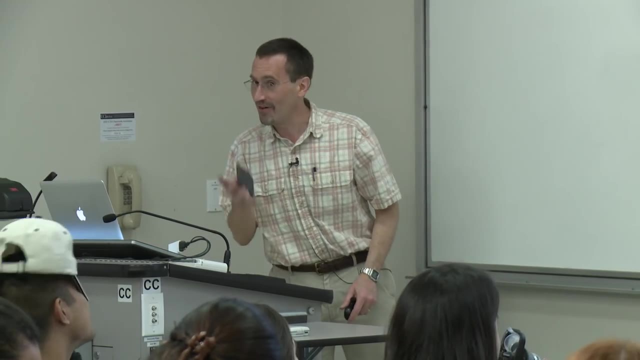 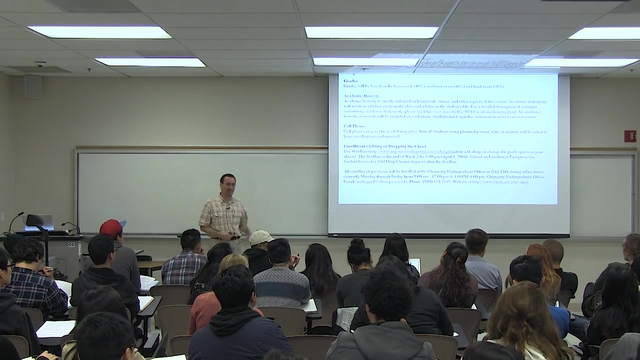 or we'll focus the camera on you and put you on the internet of live embarrassing things, or send a picture to your mother or something, Or I'll get out my phone and post you on the website. All right, all the enrollment stuff is handled by the. 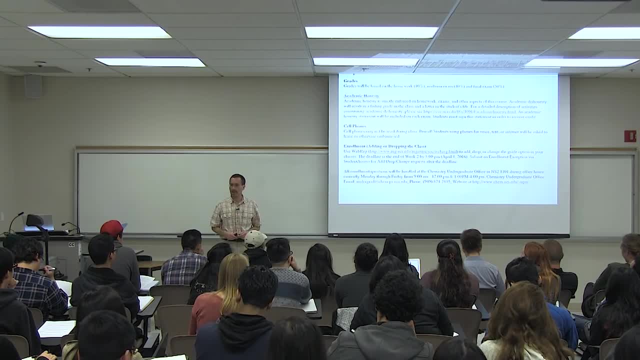 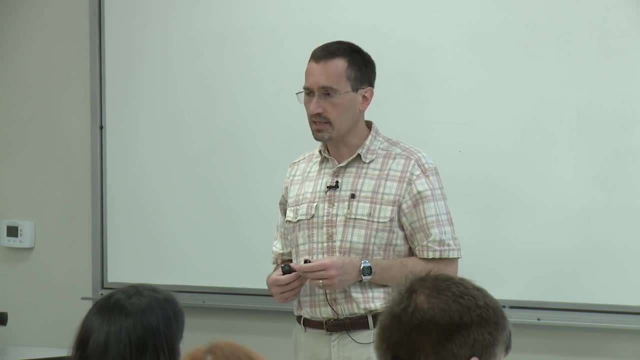 the undergrad office And I think they have two weeks to drop the class And it is going to be a hard class And if you look at the first homework and the first couple of weeks and you say, oh my god, I'm just in over my head, 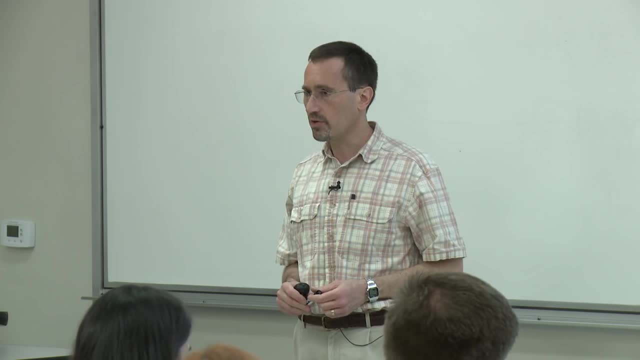 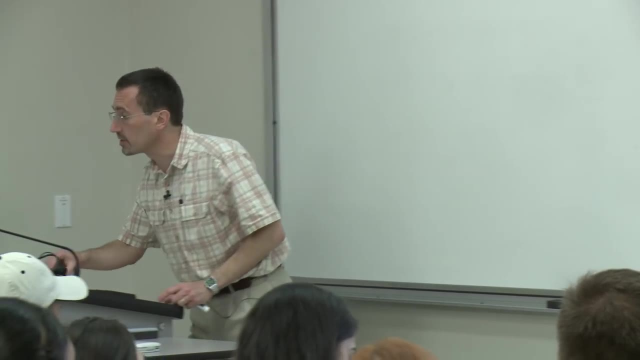 Come and talk to me if you're concerned, if it's to see if it's right for you. You know it's OK, You can figure things out. Anyway, I think it's going to be a good class. I think we're going to work really well together. 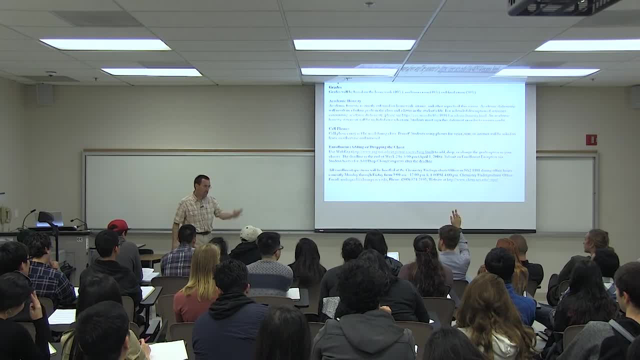 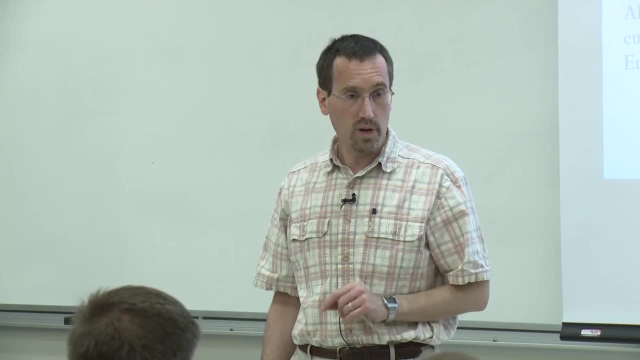 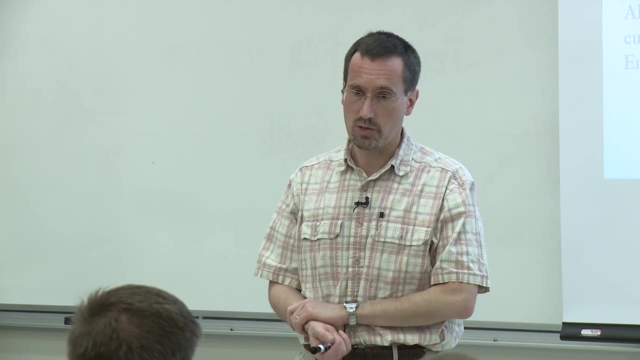 Questions or thoughts On the syllabus. Yeah, For homework assignments, will there be a key posted after? No, we are. we will basically mark answers on the homework, basically a little correction or a little guidance on there. So no, there won't, won't be keys present. 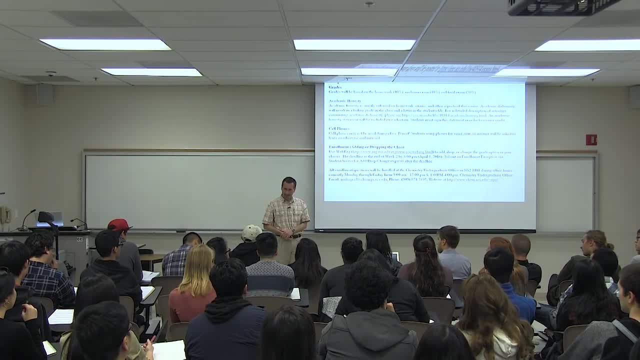 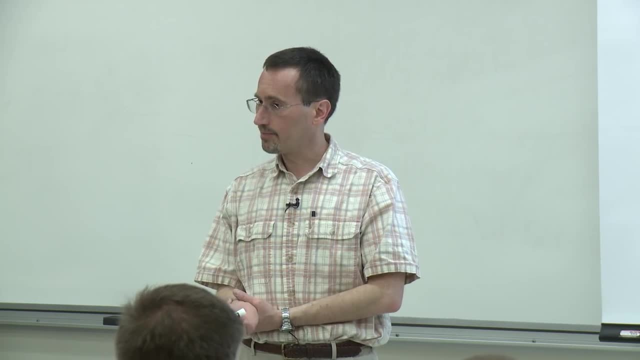 Yeah, If we're unable to make the office hours after 11 or noon on the, Just send me easiest thing. Scheduling is a little tricky because it has the back and forth. I mean if you say, are you available at this time? 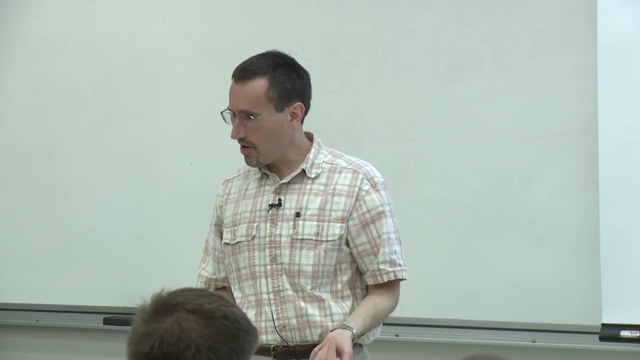 that's easy, Easy thing. pick up your cell phone, give me a call, say: are you in your office, can I come by? That's that's probably the most expedient. or catch me. catch me right after class. 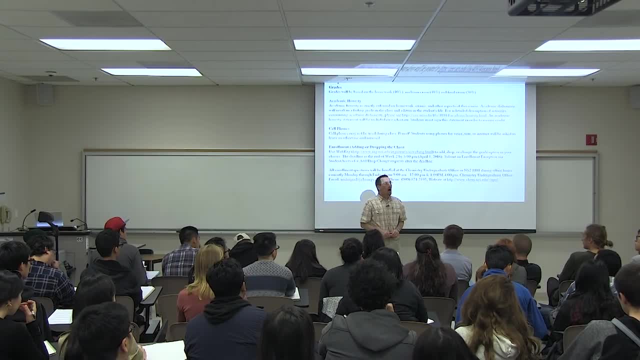 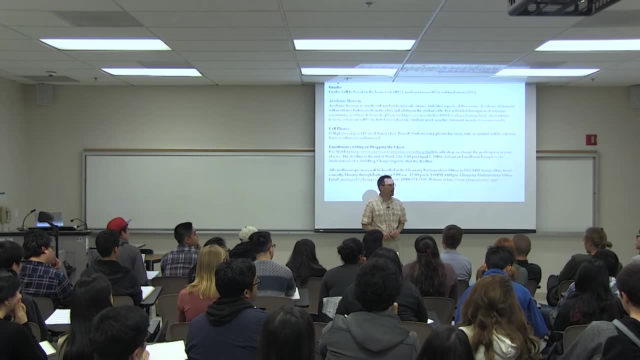 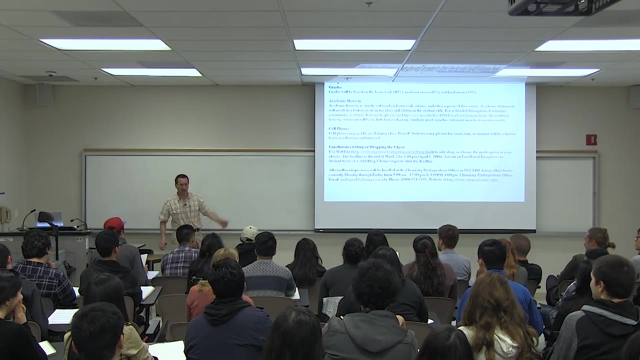 Will any of the supplementary text be available at the bookstore? Art of writing. reasonable reaction mechanism: no, No, OK, OK. OK. Amazon, OK, All right. How many people got the textbook at the bookstore and how many? how many bookstore? 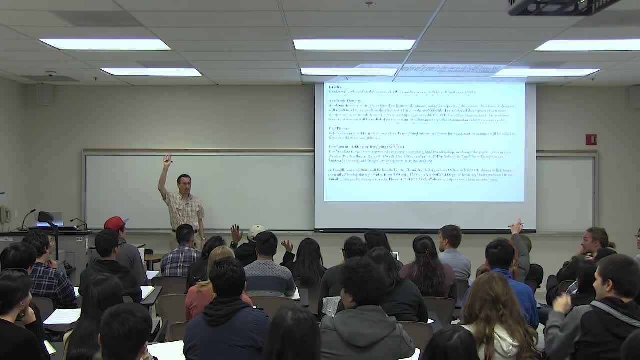 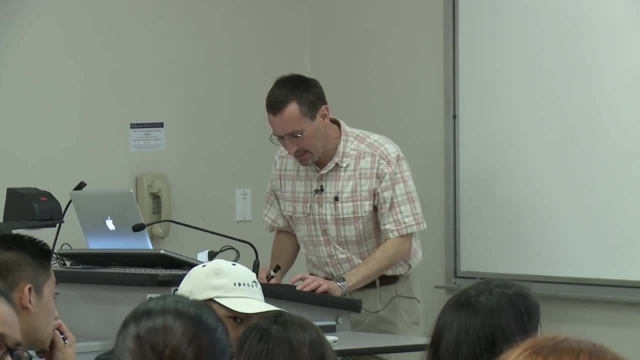 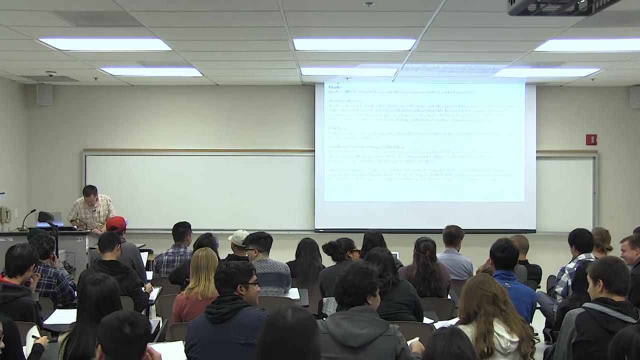 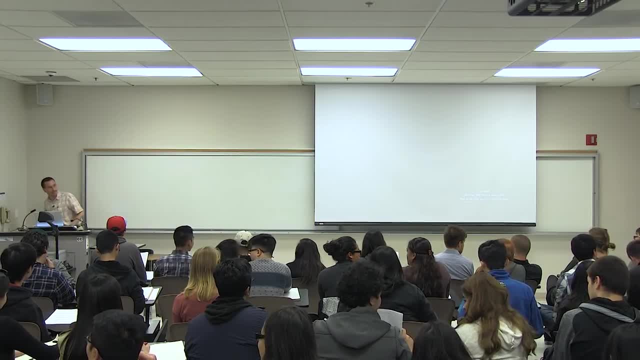 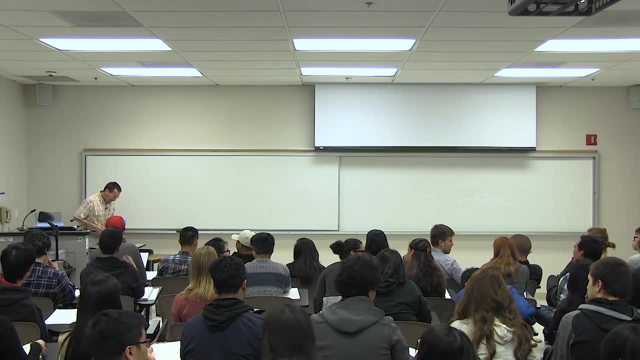 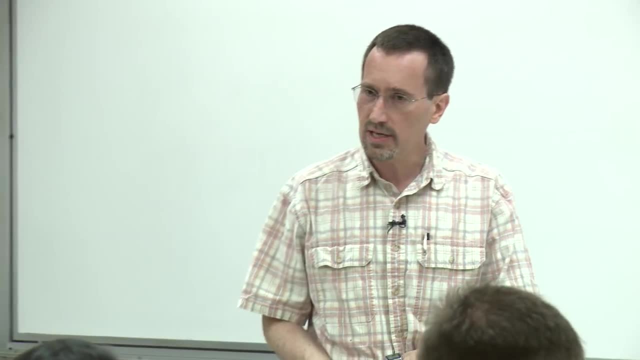 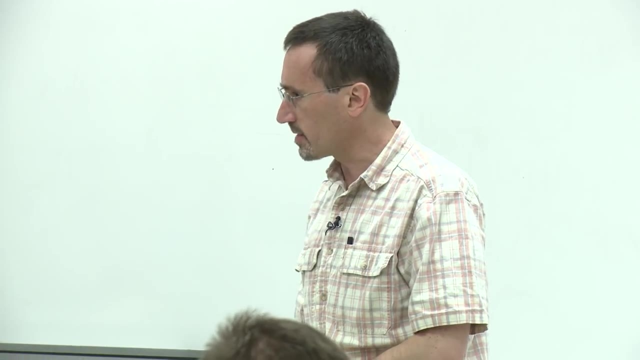 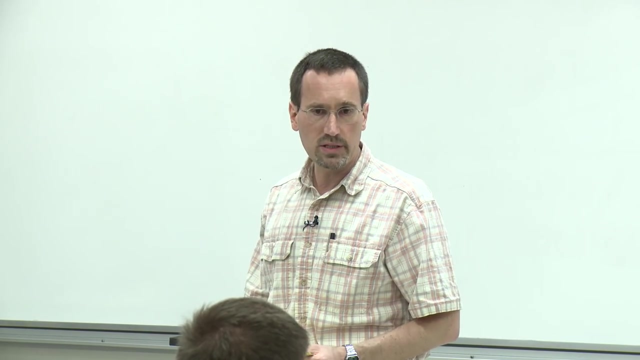 So the way I teach this course is basically as a survey of advanced topics, the same types of topics that the graduate students get in their classes. In other words, we go into things that I think are important and fundamental to organic chemistry. Now, the first thing we're seeing in chapter one: 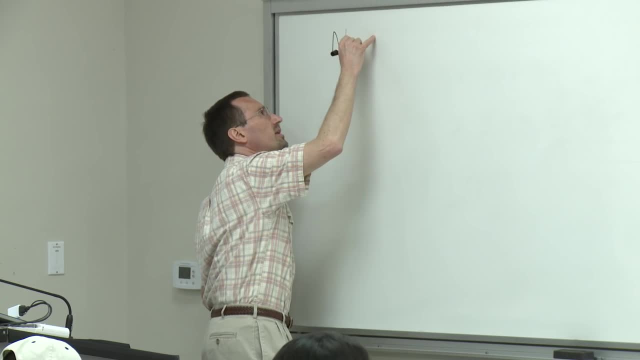 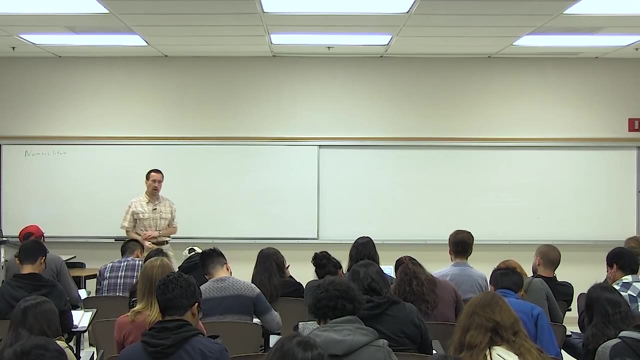 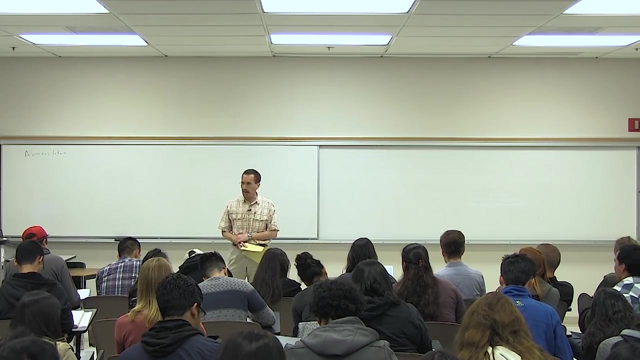 although it's ostensibly on nomenclature, in other words, how you name molecules, what you're seeing in chapter one is it really is about molecules. In other words, the molecules that you got in your sophomore class were simple, simple representations, for the most part. 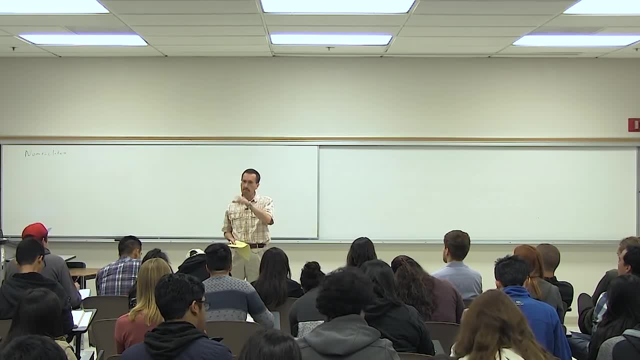 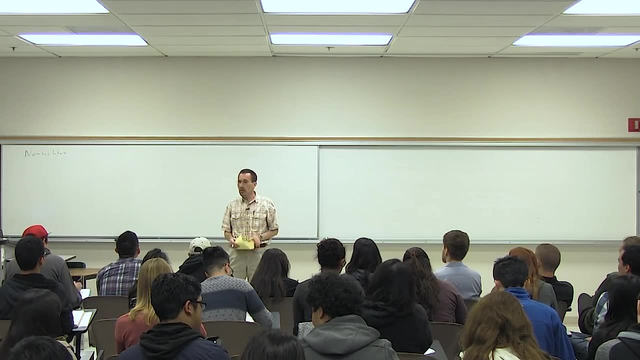 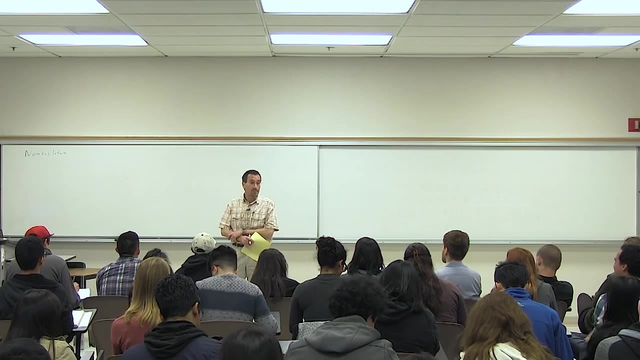 of organic molecules containing the minimum amount of sort of extra material and the minimum number of functional groups, and we almost lose the beauty of it. We almost lose the beauty of the millions, millions upon millions of ways, infinite ways. but right now we've got, you know, 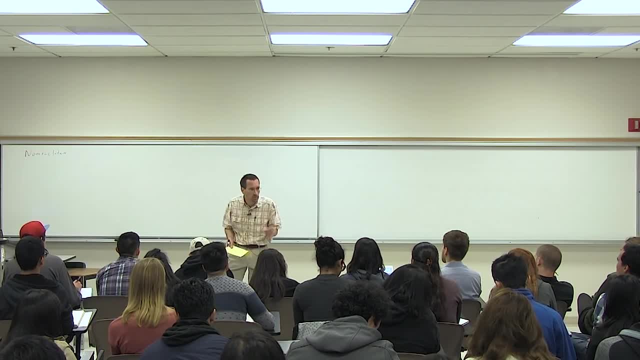 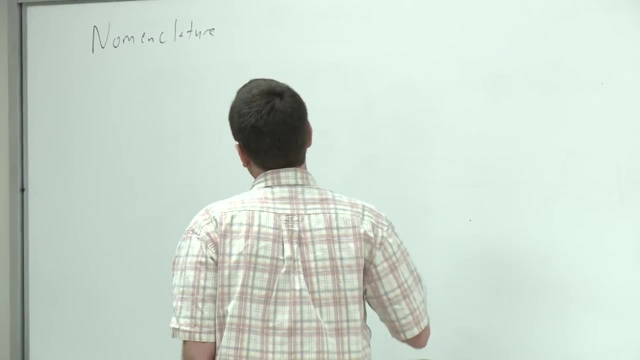 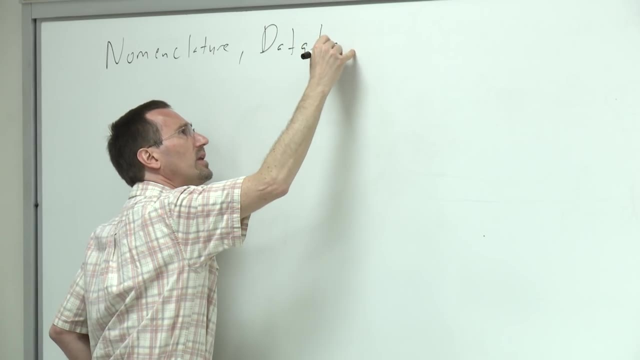 tens, hundreds of millions of known organic compounds and we almost lose the beauty of that. Chapter one, while it's on nomenclature, really is about the anatomy of organic molecules and we're going to segue from chapter one into databases, which is basically how we learn. 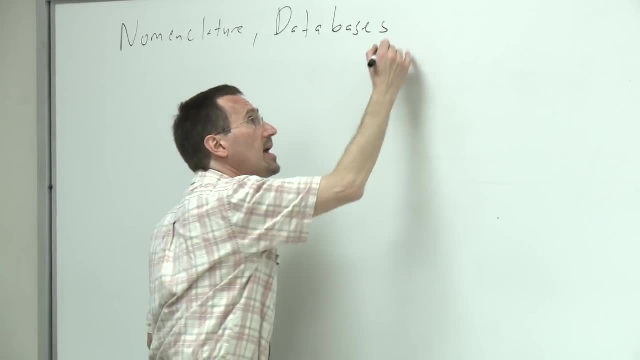 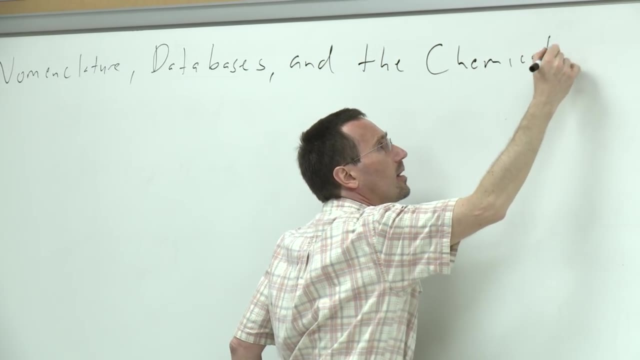 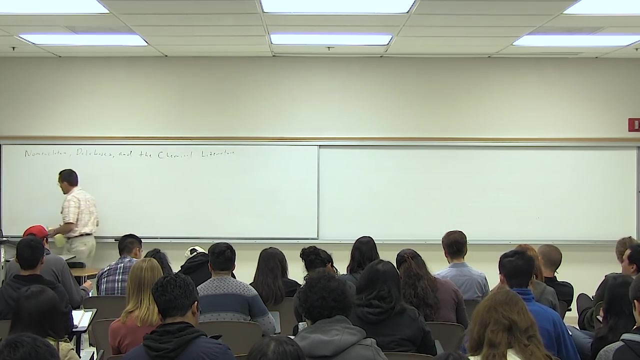 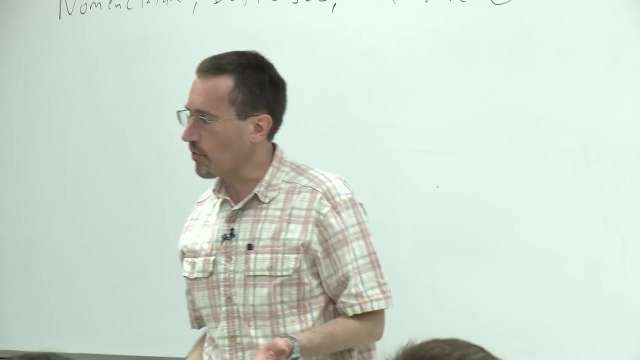 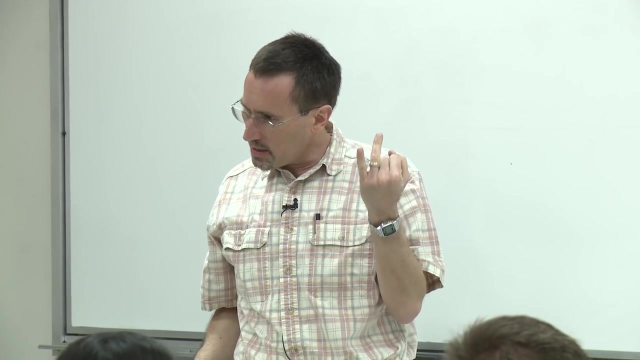 about real organic molecules and we're going to go to the chemical literature. So that sort of is our introduction. That really is, That really is just our first week Now in terms of big ideas, the big ideas of organic chemistry basically become functional groups. 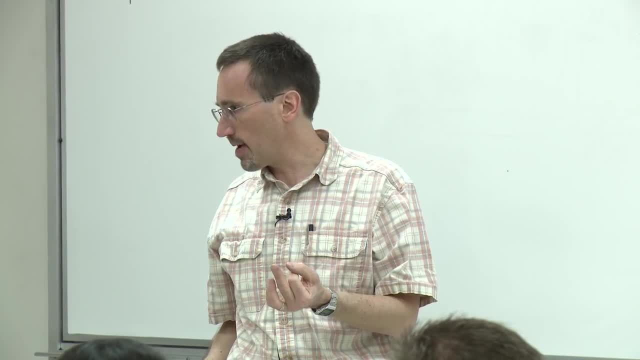 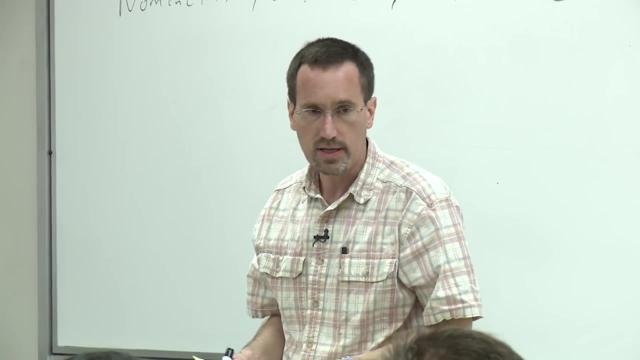 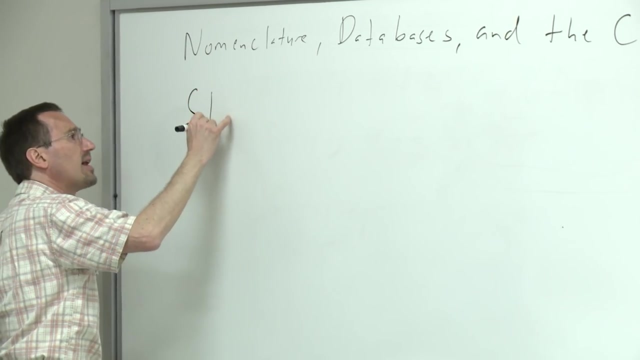 stereochemistry and reaction mechanisms. That is the overarching theme that ran across your sophomore organic chemistry class and we're going to go into more depth and it's going. we're going to move fast and assume that you've got sort of the basics of stereochemistry, but we're going to move. 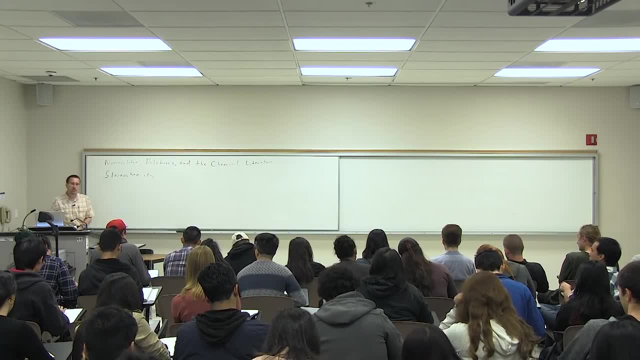 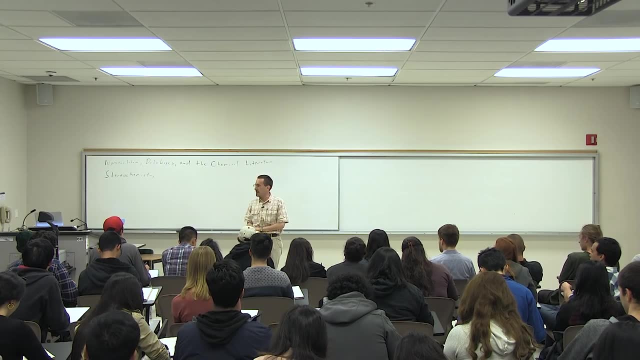 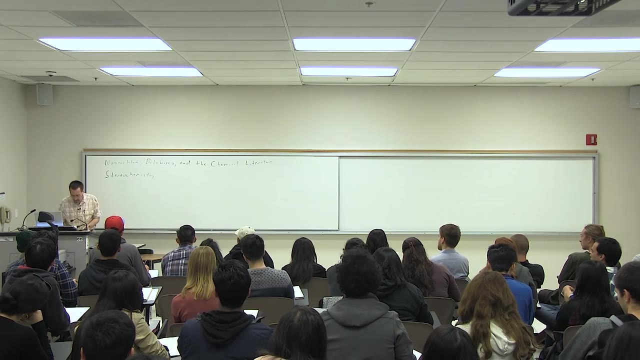 into stereochemistry, which basically goes in and shows us the beauty of the three-dimensional structures of carbon-containing molecules and nuances like atrobisomers and other factors, other features that you probably didn't get in the introduction. It's going to be fun. 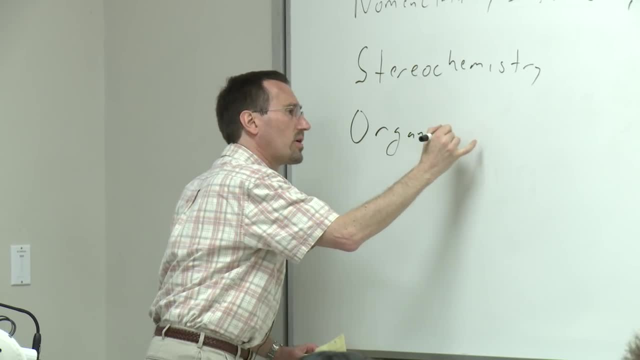 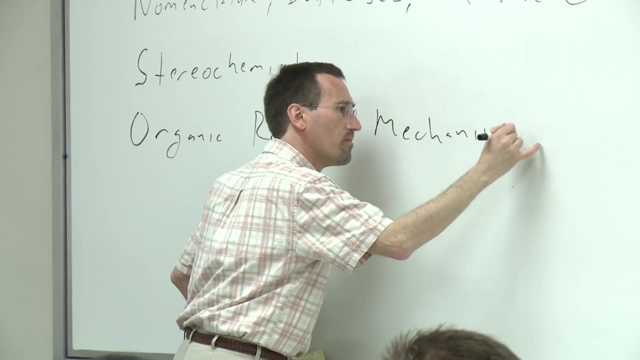 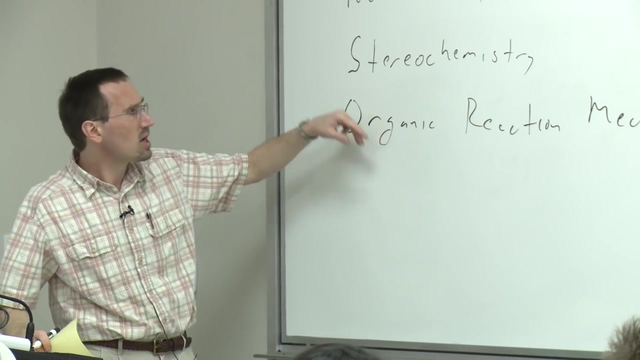 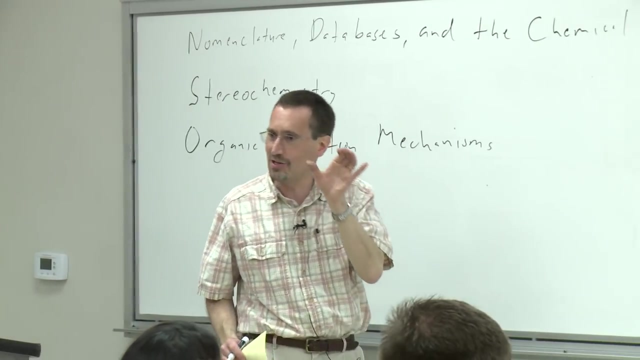 We're then going to have a couple of chapters on organic reaction mechanisms- One of the big concepts. in fact, we have two graduate level courses on reaction mechanisms, Although we don't have a graduate course on stereochemistry. I have a 1,400 page master work. 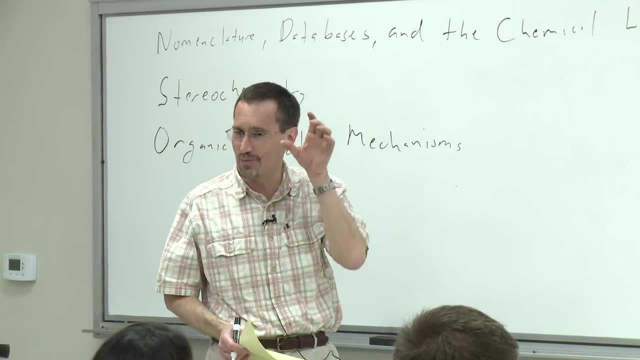 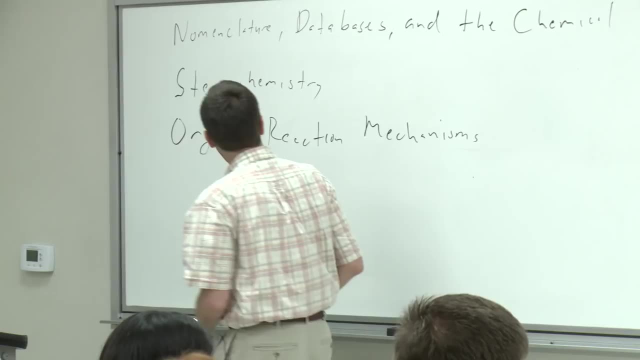 by Ernest Elial, as well as a smaller 500 or 600 page, but we're going to have a lot of work by him on stereochemistry, So it's a big and beautiful topic. As I said, we're just going to get a taste. 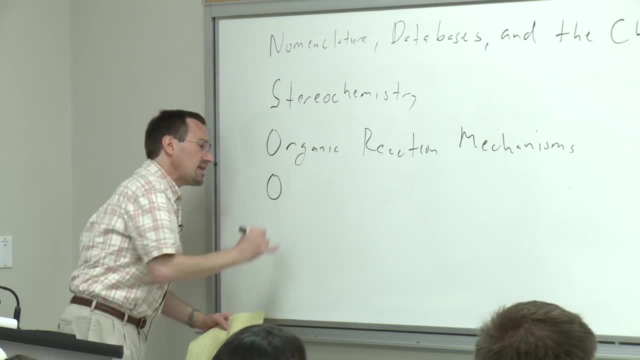 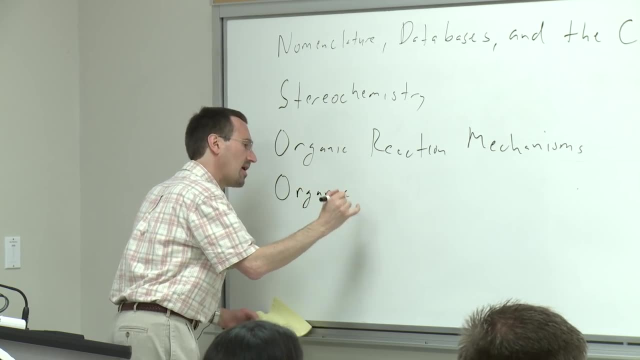 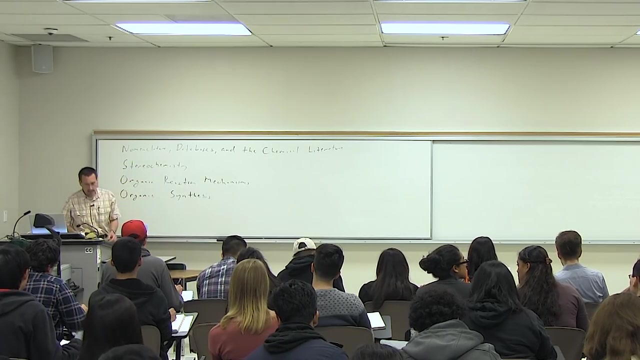 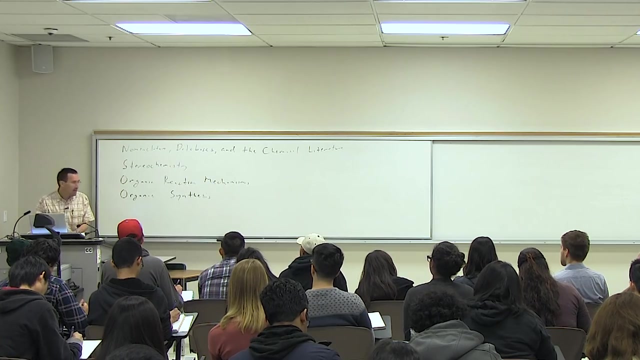 a couple of weeks going deeper. Organic syntheses are going to represent functional groups and their transformations and carbon-carbon bond forming reactions, and again, this is a topic that we have two graduate level courses on. You're going to go a little bit deeper on that and then the last week of class, 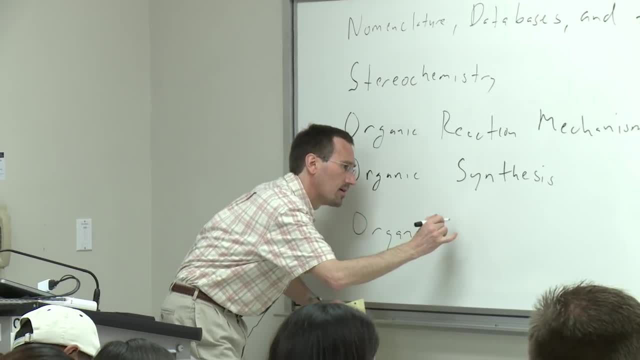 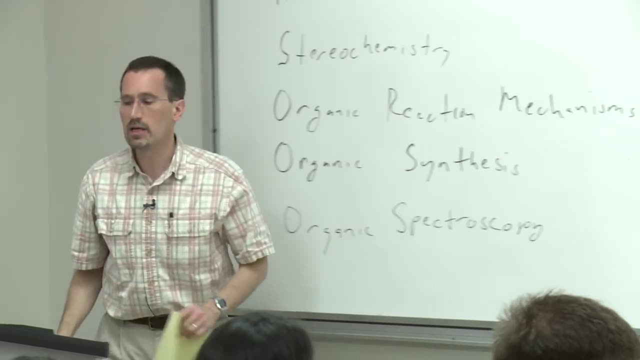 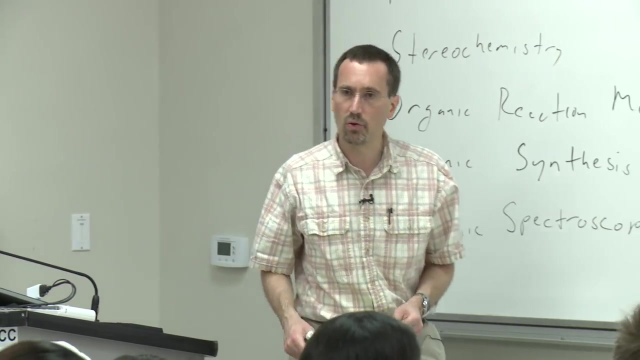 we're going to go into organic spectroscopy, mostly NMR, but maybe a little bit of a review of IR, maybe a hair of mass spec, and again, we have a graduate level course on this topic. All right, so let us dive in to chapter one. 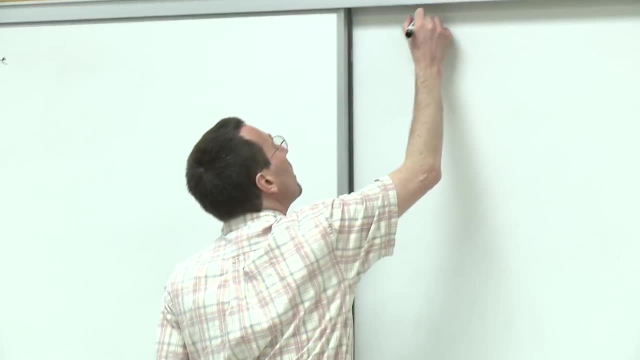 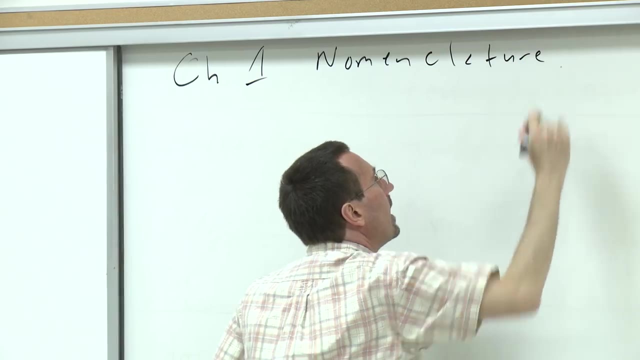 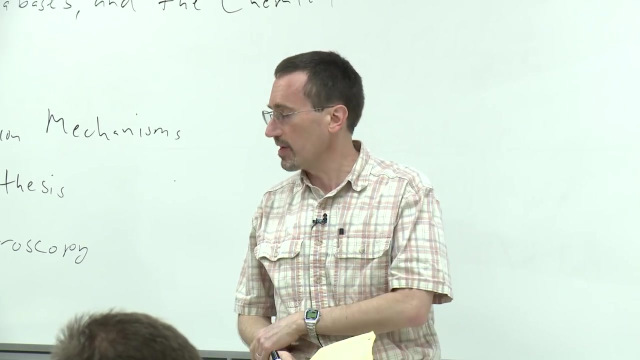 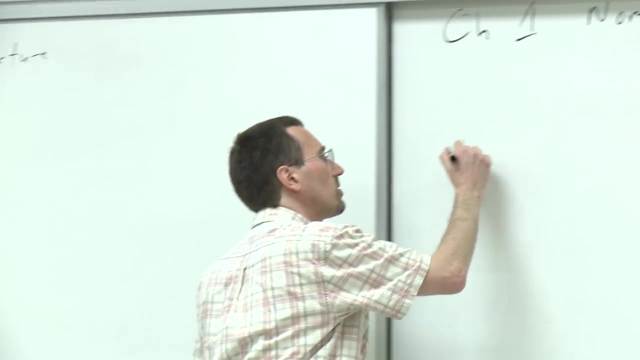 and start talking about it. Let us talk about nomenclature. All right, I am going to take as a given that you have, if not right at your fingertips right now, certainly the ability to refresh your memory on some basic nomenclature. 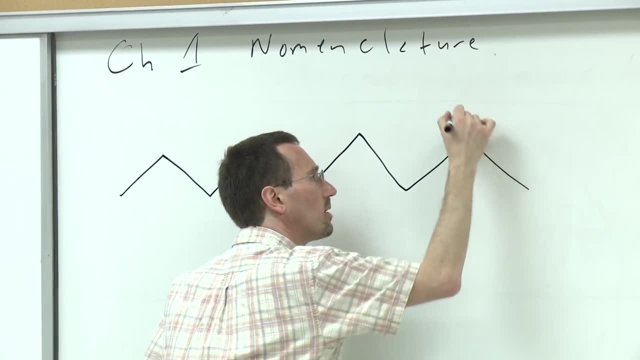 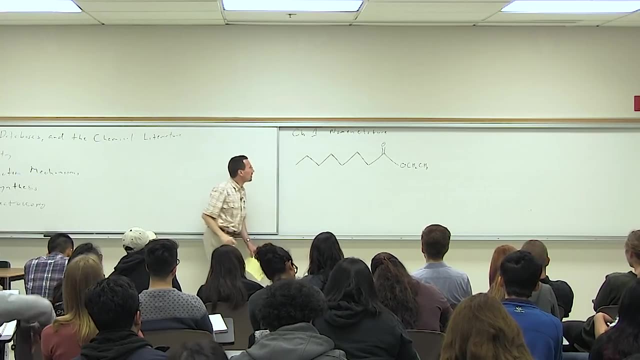 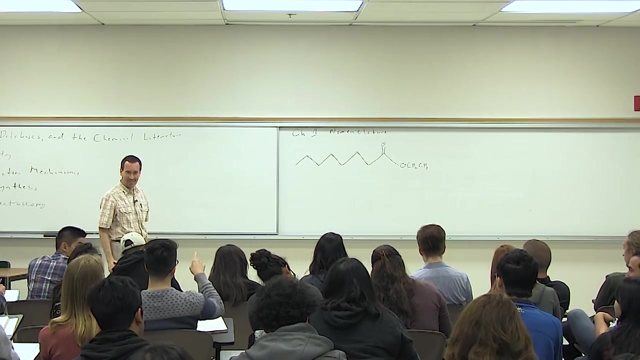 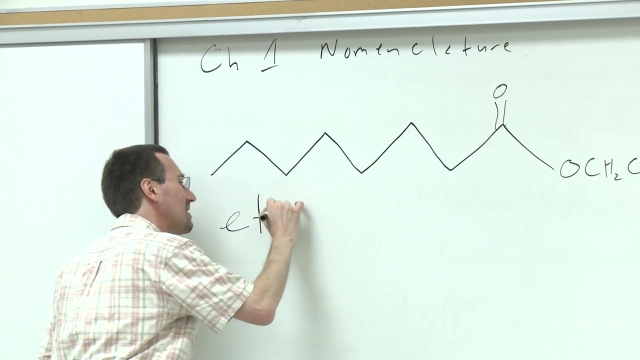 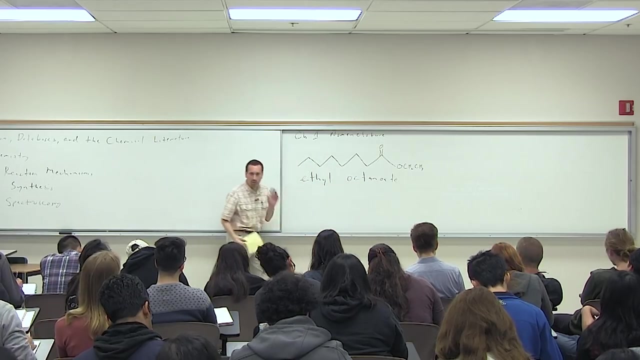 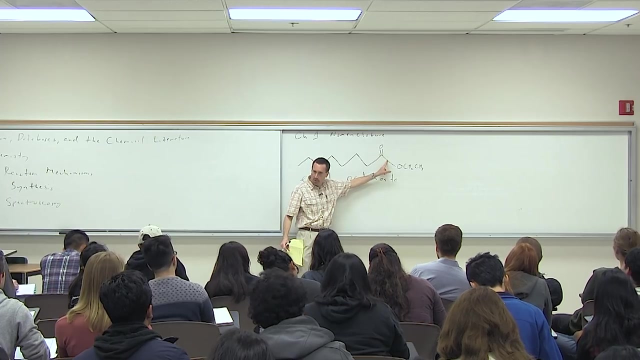 So if I draw the following compound, who can give me a name for that? Octanoate, great, fantastic. I am not mistaken here. In other words, you looked at this compound, you recognized that the most important thing and functional group in it was an ester group. 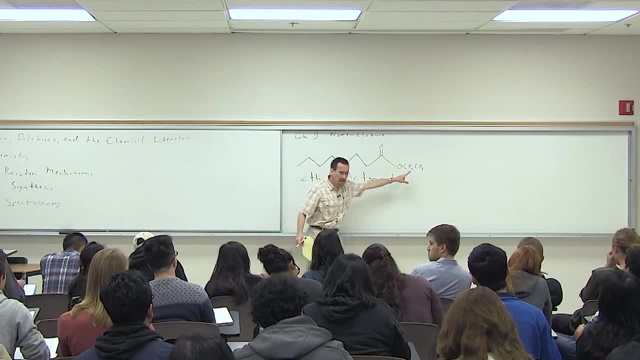 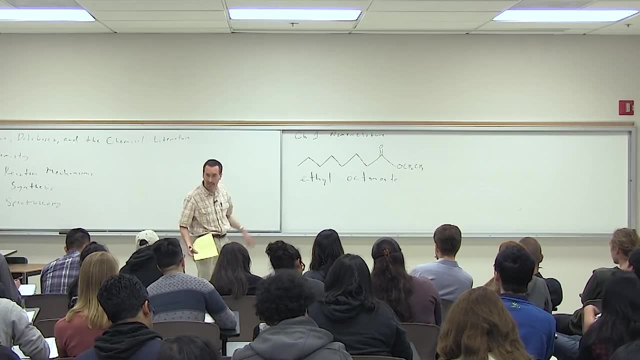 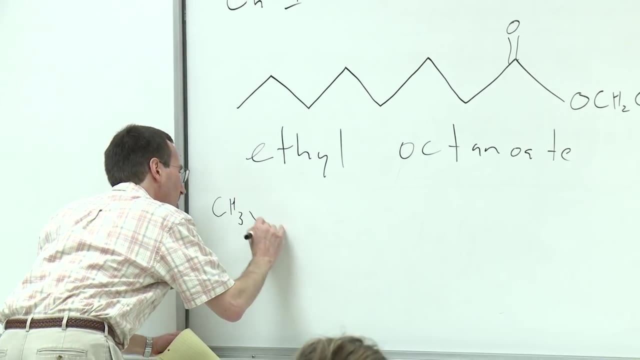 It's an ester of octanoic acid, It is the ethyl ester. and we name an ester, first name the alcohol part, ethyl, last name the octanoate part, And if we go ahead and play with that theme, 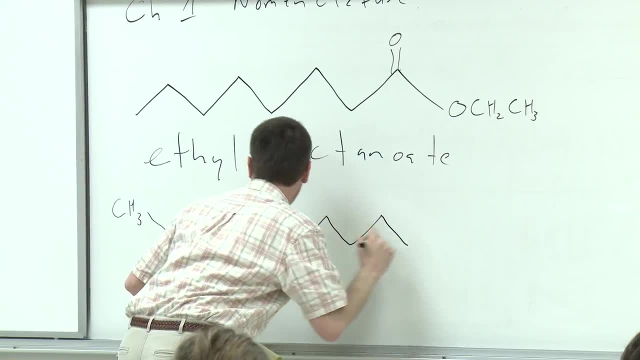 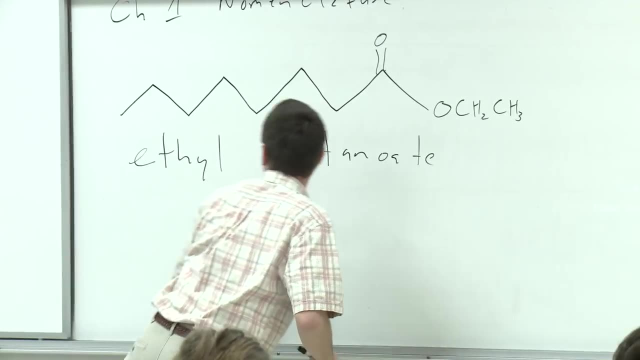 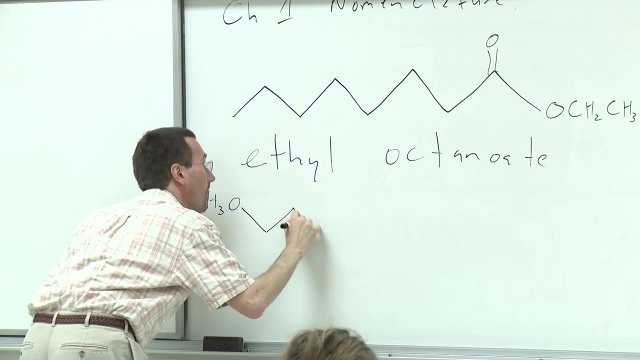 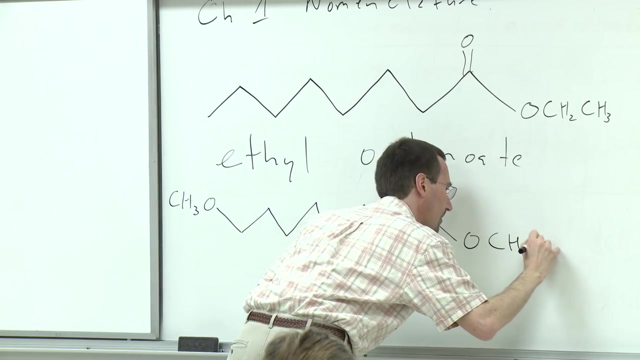 we know about substitution. Oops, I'm going to draw this. Okay, so we're going to draw a little bit of a picture. Let's see, Let's draw this in such a way that it aligns here. All right, so playing with that theme. 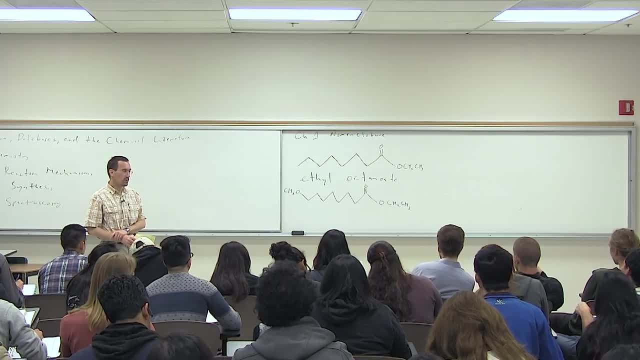 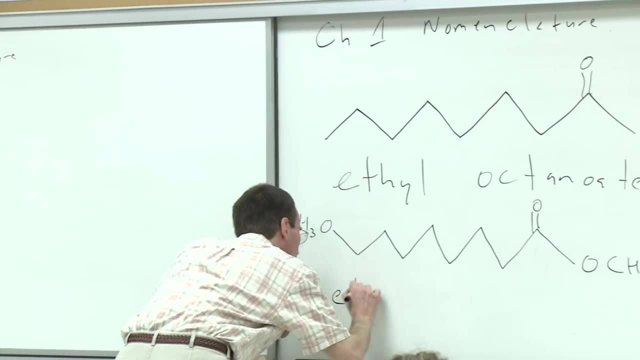 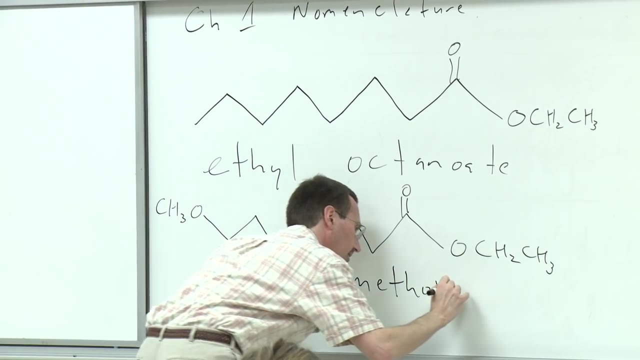 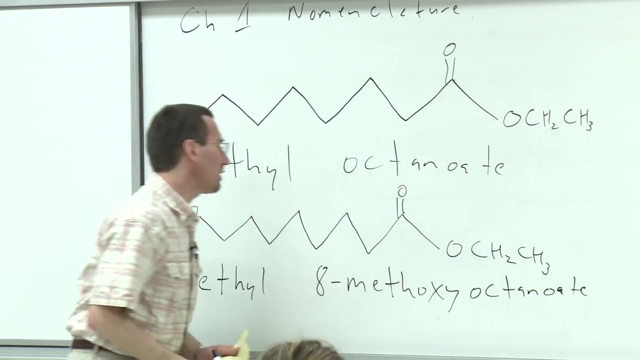 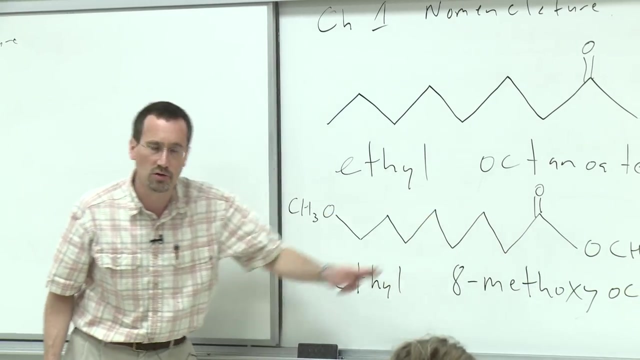 who else can give me a name for this molecule? Perfect Ethyl-8-methoxy-octanoate, all one word. In other words, you have looked at the molecule, recognized that the highest priority functional group is still the carboxylic acid functional group. 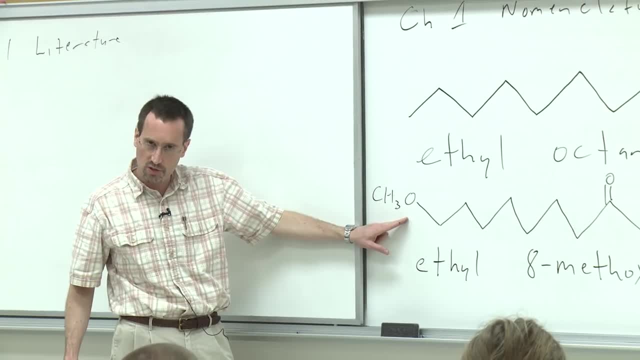 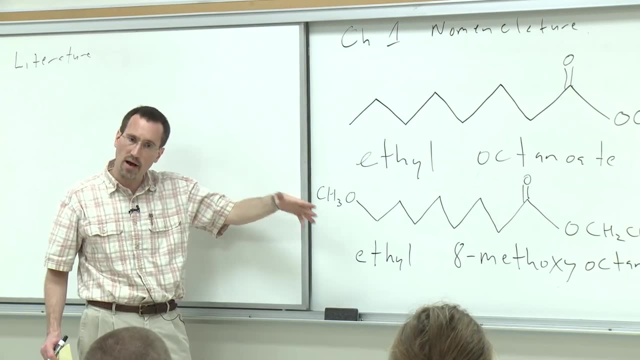 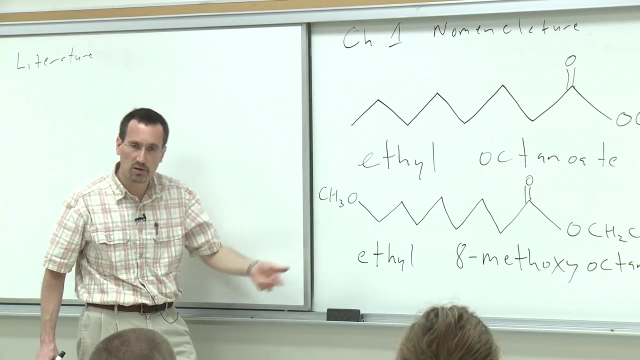 Even though you see that you have an ether functional group, you know it's lower in priority. In general the priority goes with oxidation state. so alcohols and ethers are lower oxidation state and priority than aldehydes and ketones, which are lower priority and oxidation state than esters. 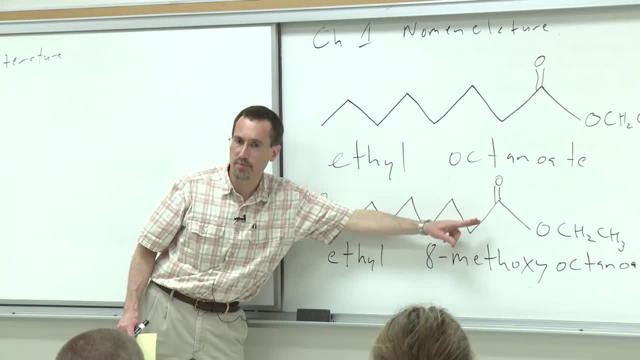 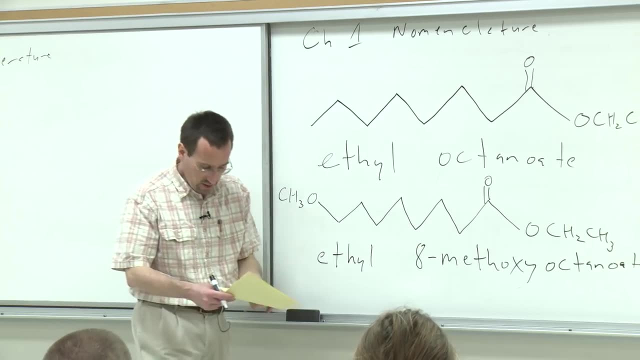 So you named it as a substituent and you remembered that you number your chain from putting the functional group at the lowest number: 1,, 2,, 3,, 4,, 5,, 6,, 7,, 8, and so forth. 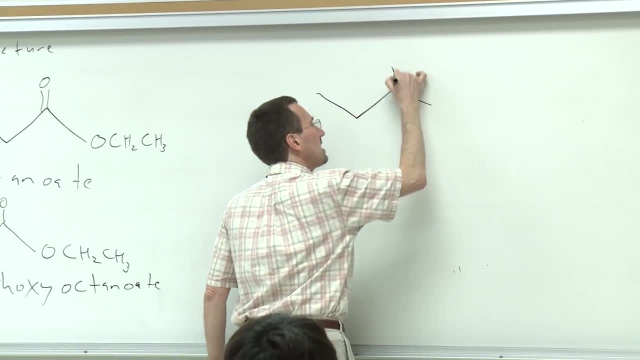 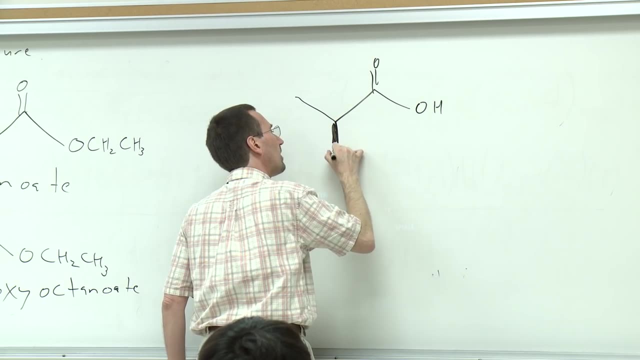 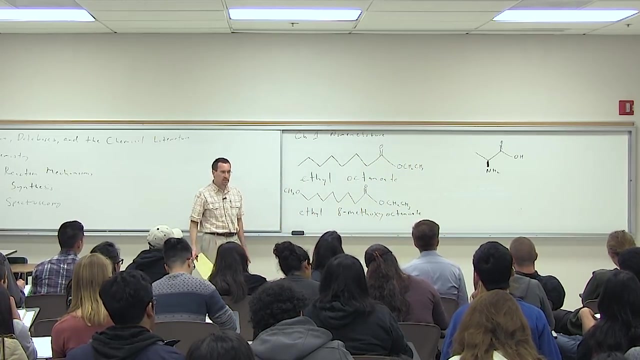 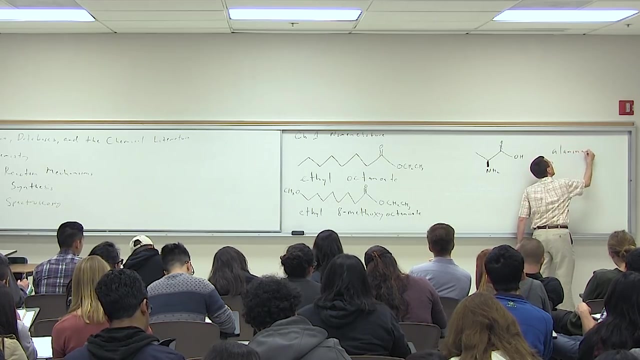 The other one that I'm going to take as a given, maybe with a little bit of dusting off, is that you can remember your Conning-Gold-Prelog stereochemistry. So this molecule's casual name is alanine. It's an amino acid. 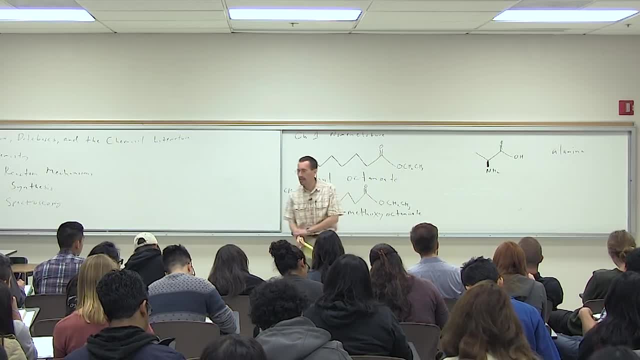 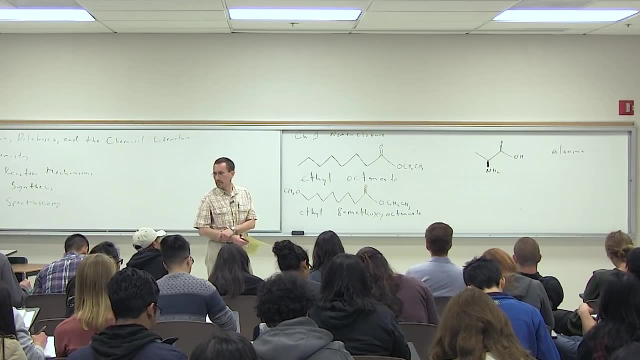 You can also call it L-alanine. It's the simplest amino acid with stereochemistry, But if we want to come to an IUPAC name for it in the same principle with a stereochemical designator, how do we name this molecule? 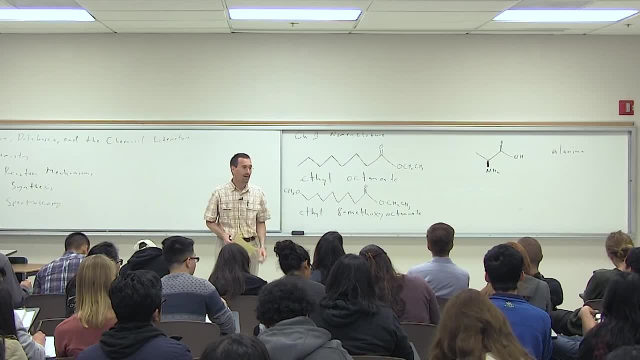 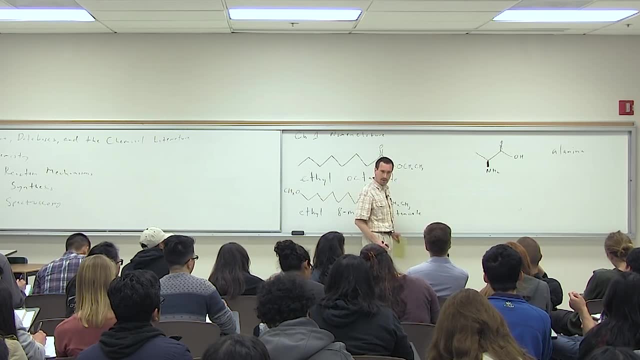 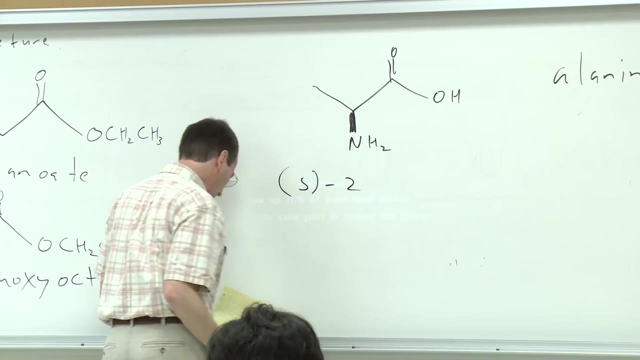 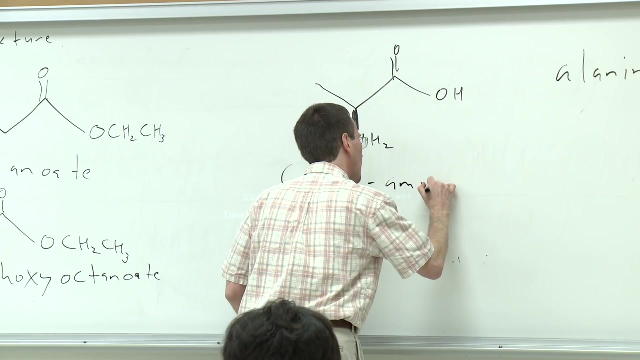 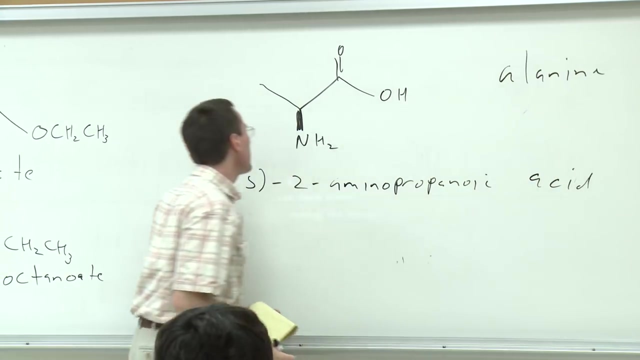 Someone else? Okay, Pretty much. yeah, S, we can put the designator. I think it can go in either place. I think it can go 2S or S2-aminopropanoic acid And, honestly, the biggest principle I want us to take away on this, 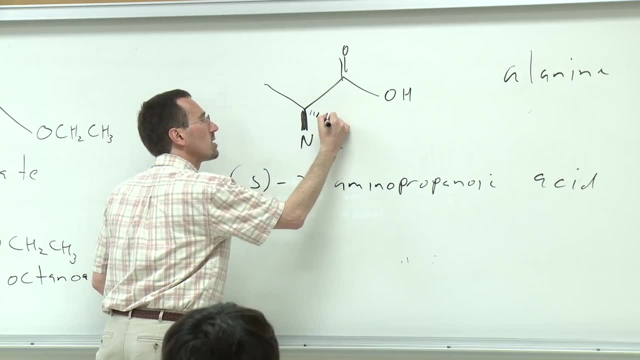 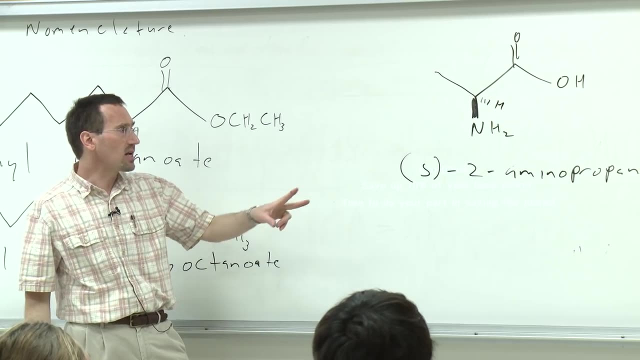 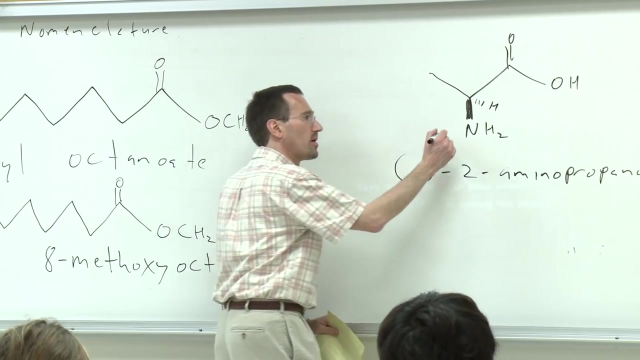 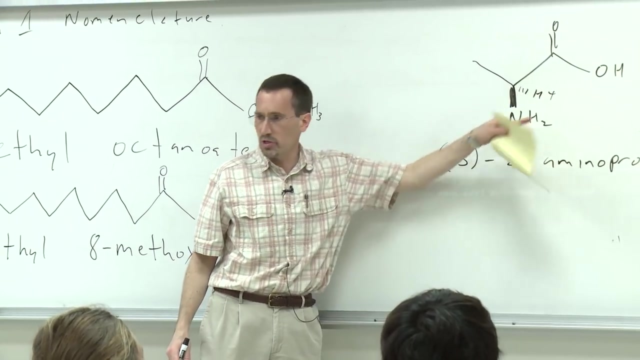 and again by way of review, is you're giving assigning authority, you're assigning priority to the atoms based on atomic number and then substituents attached to it and their atomic number, and citing down the bond to the lowest priority. So the stereocenter, here, the hydrogen, is the lowest atomic number. 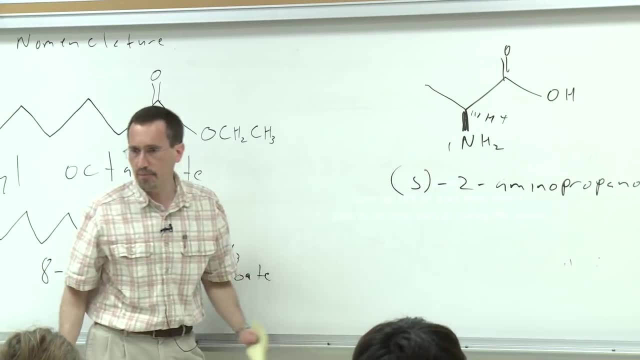 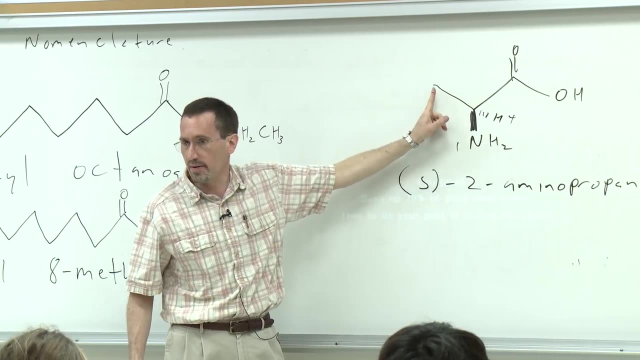 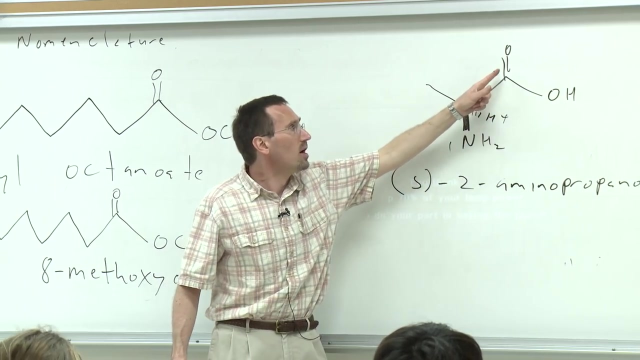 the lowest priority, The nitrogen is top priority of the two carbons. the carbon bearing number, The carbon bearing the oxygens, is higher priority than the carbon bearing the hydrogens. And if you want to get really into the nuances which you may at some point have to, 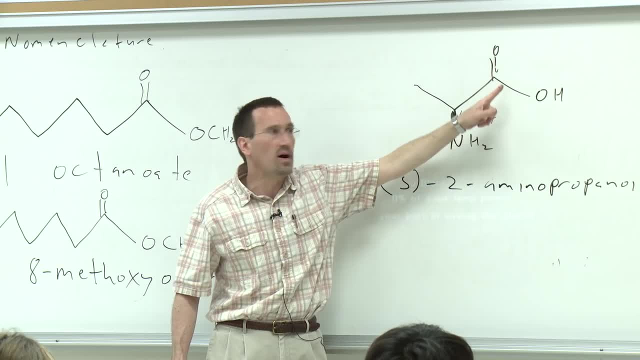 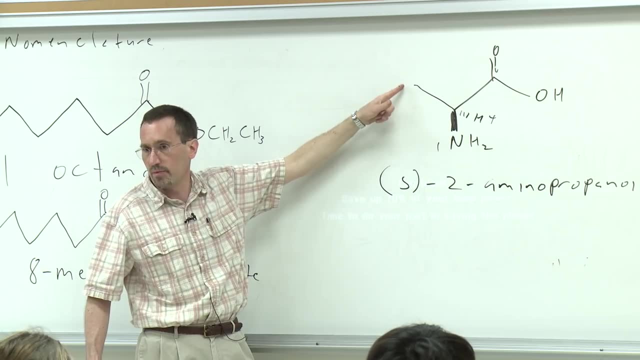 we count this oxygen as two oxygens with a double bond. So this is equivalent to a carbon with three oxygens bound to it. If we say, had an aldehyde here, it would be carbon 2 hydrogens, two oxygens bound to it. 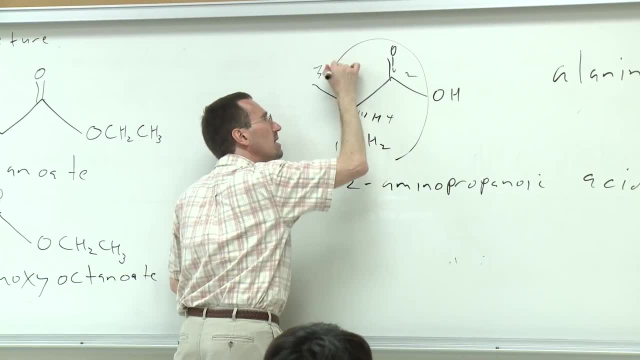 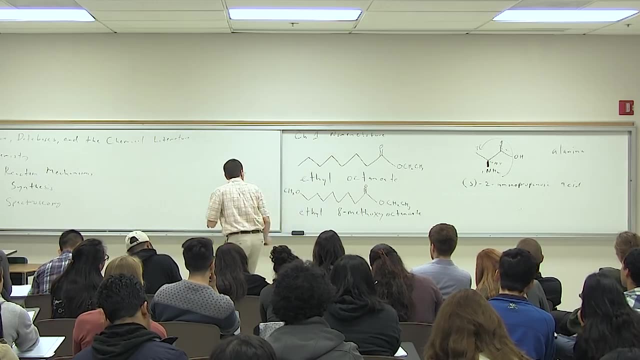 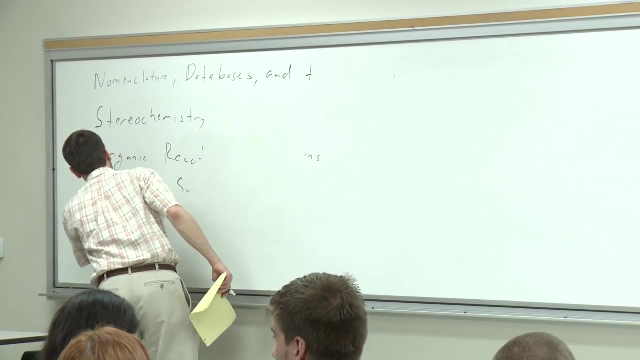 And so our priority goes 1,, 2,, 3.. You cite down the bond. It's counterclockwise, And so you can assign it as S stereochemistry. All right, OK, All of that is sort of taken as a given for where our textbook begins. 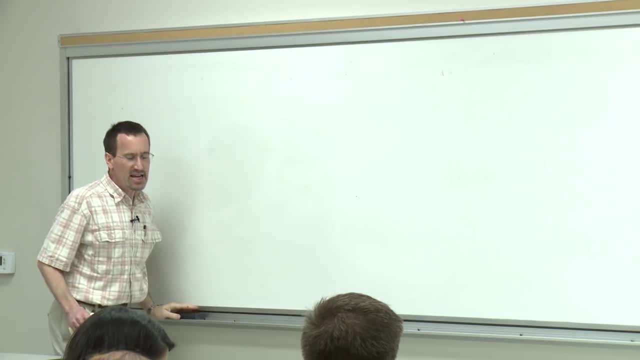 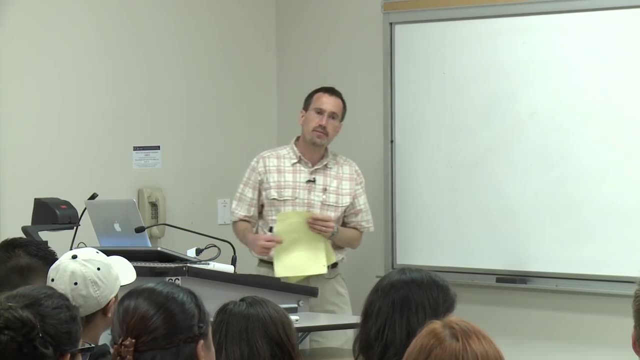 And I picked, by the way, on the homework I tried to pick, I think, about eight problems that I thought really catch the essence of the chapter. I don't expect this. This is a meaty chapter. Chapter 1 is meaty. 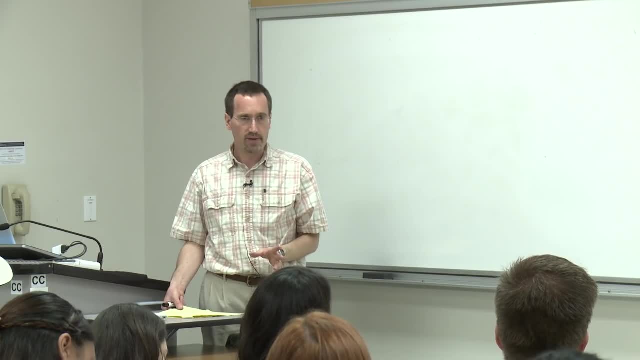 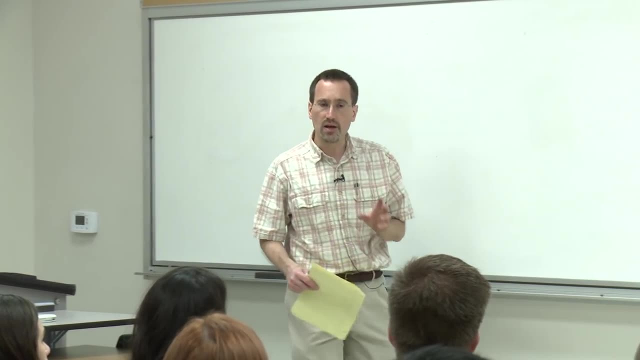 I don't expect us to have 100% mastery of organic nomenclature. Don't get scared. What I want is for us to come away with a flavor of what all this nomenclature means. And I have a confession to make. 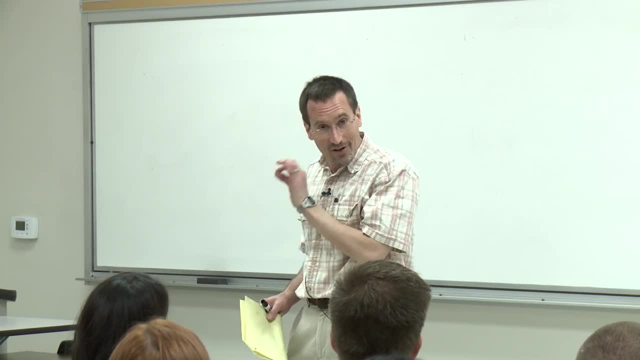 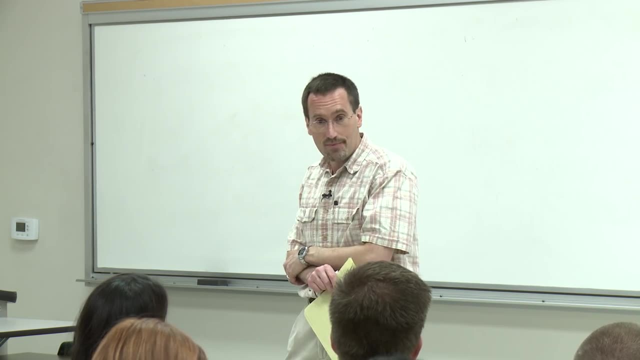 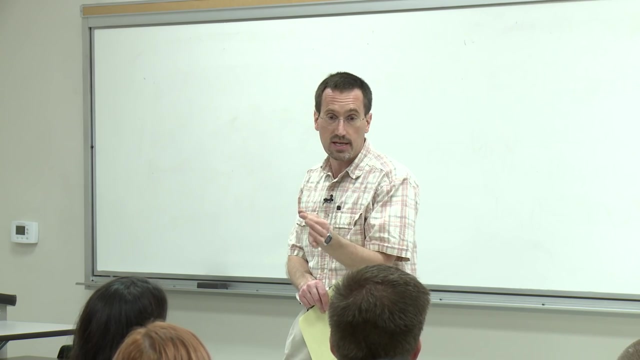 In all of my graduate courses I never had one time that really went through this And I saw a lot of these names And, honestly, the first time I picked up this chapter 1 and just looked at it, basically it's like so much of the stuff that I had been seeing for years. 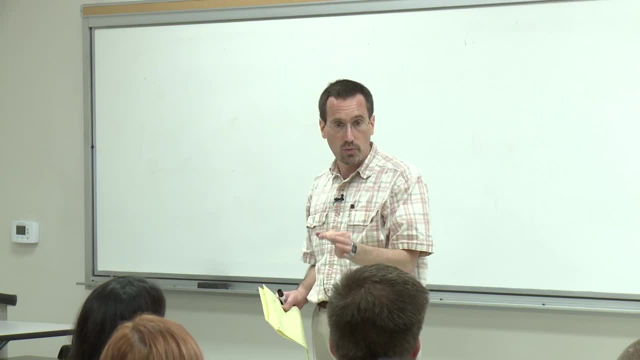 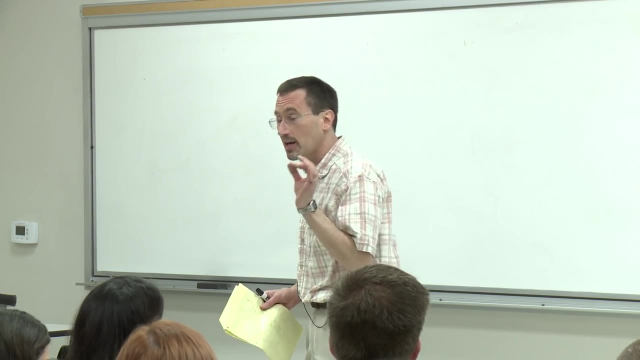 made sense for the first time, not because I was a master and could do it all perfectly with my eyes closed or the book closed, but because, having seen it once, it's like, OK, all this makes sense. Some of the stuff you just pick up along the way. 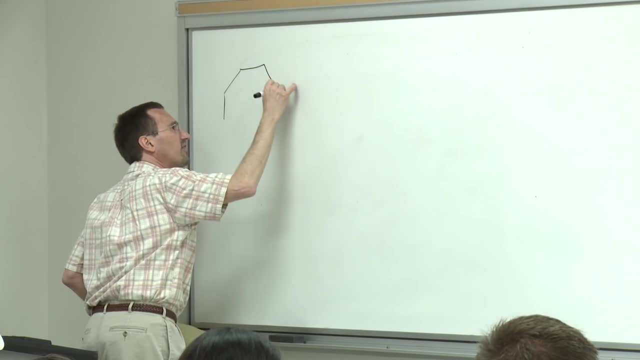 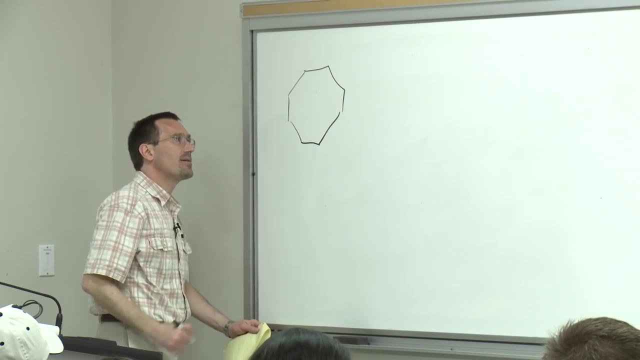 and we're just going to you know which I had done, but then some of the stuff like the benzo B, you know, quinoline or something. actually it's like: OK, now that makes sense. OK, so this is a cycloalkane. 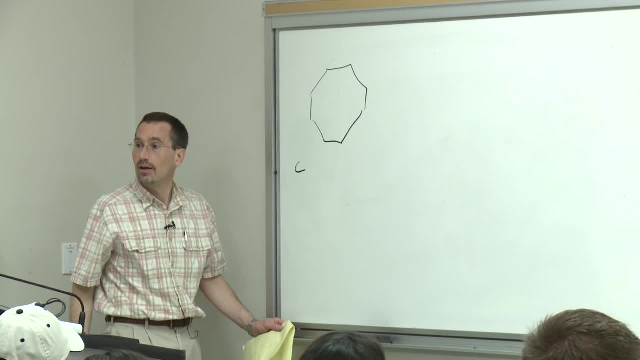 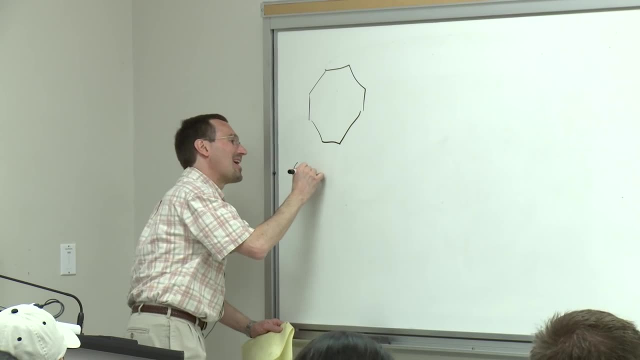 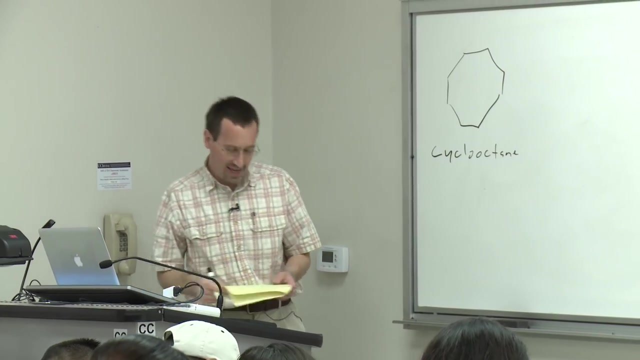 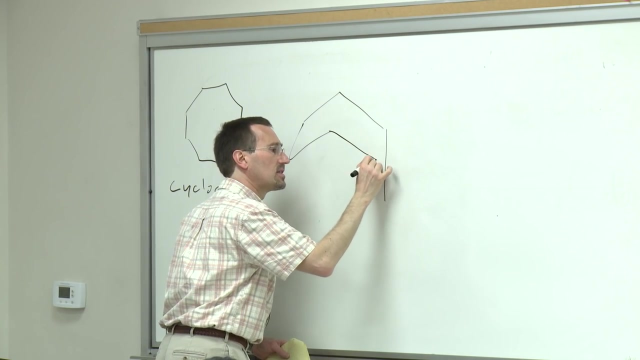 Anyone know the name of this molecule? Say it Cyclooctane. Cyclooctane- great, No breaks in it. Two O's up against each other. No hurt, no foul, All right, So where your textbook is sort of beginning. 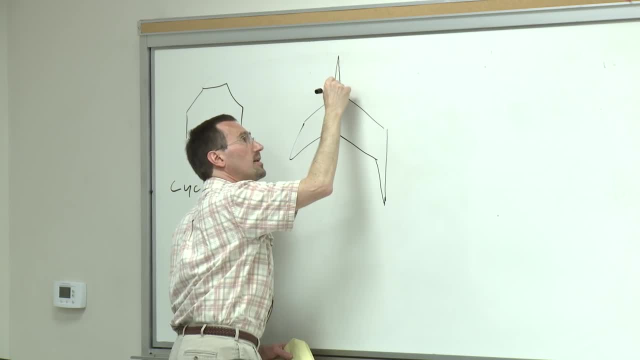 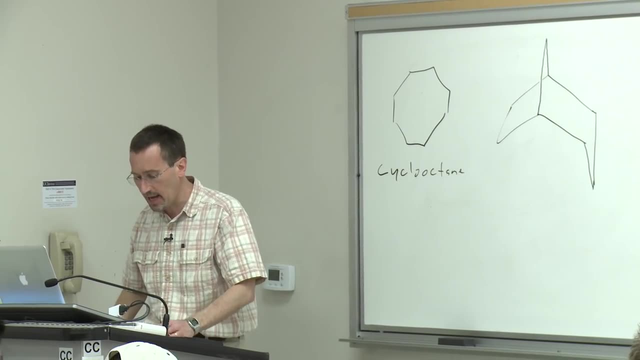 and I think it's a nice place to begin- is with bicyclic, or at least one of the places it begins is with bicyclic molecules. So there's a bicyclic molecule, one that you might not have seen in sophomore organic chemistry. 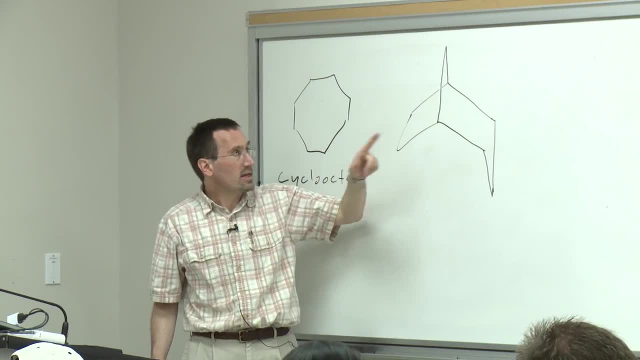 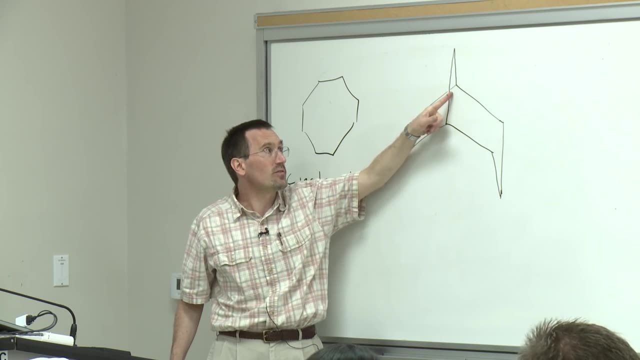 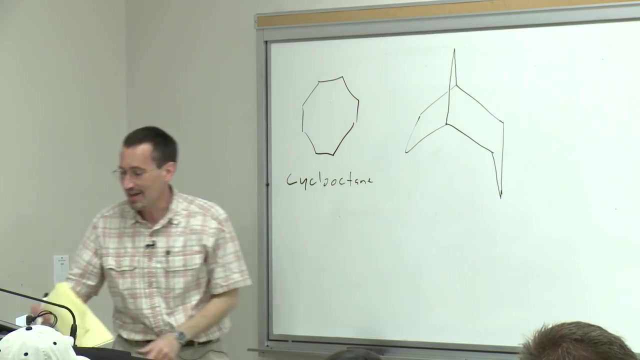 In other words bicyclic two rings. We have this bridge. If you want to get fancy- and usually I'm a slob in writing structures- if you want to get fancy, you put a little break in that line in back to show that you've got this line in front of this. 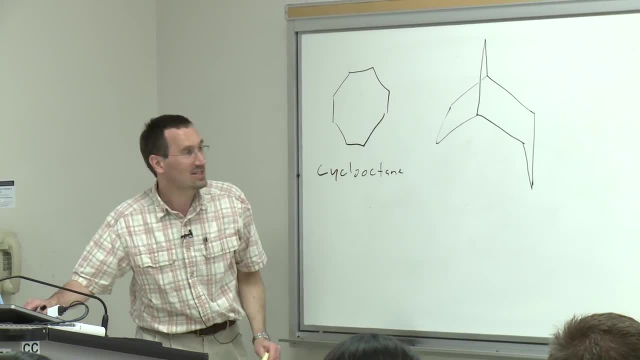 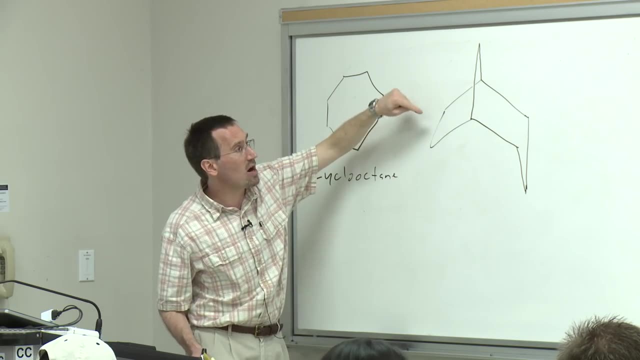 I'm going to help you make sense of this structure in just a second. All right, So this compound gets named as a bicyclo. It still has eight carbons in it: One, two, three, four, five, six, seven, eight. 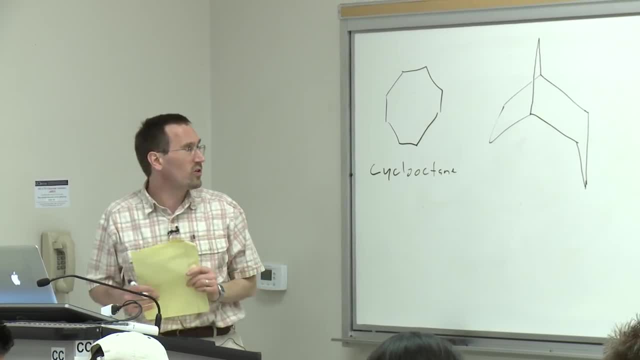 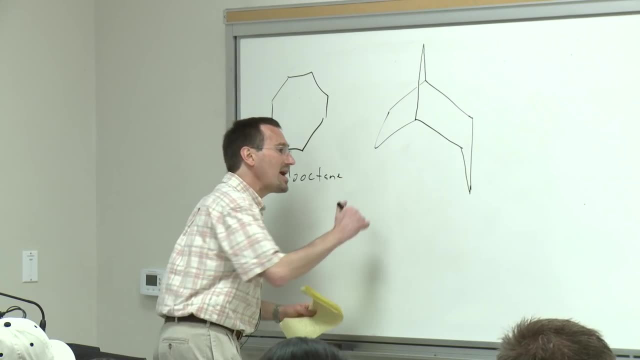 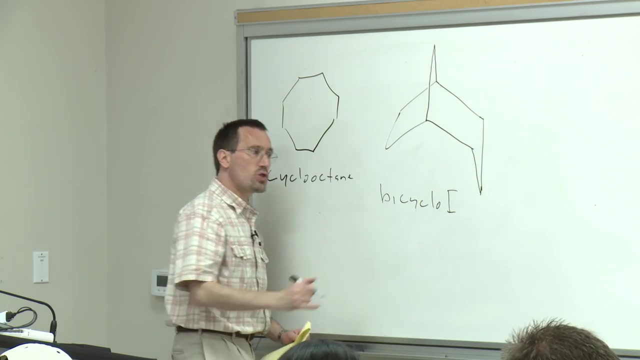 So it gets named as a bicyclo-octane. We have two fewer hydrogens than cyclo-octane because we have one more ring And we call it bicyclo. and then we open a bracket and we say three, period two, period one. 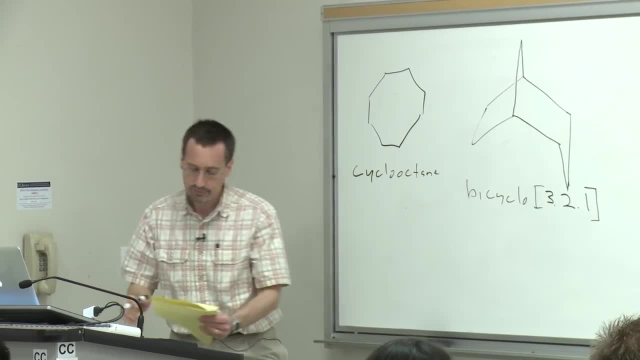 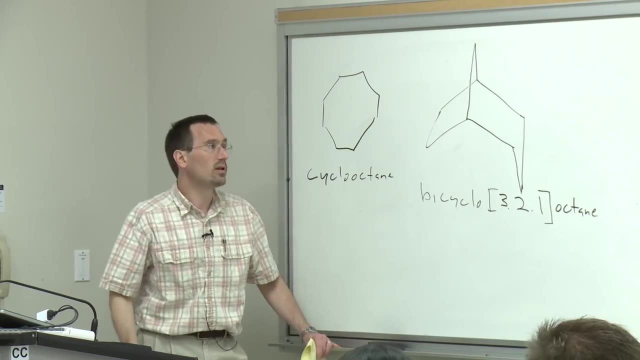 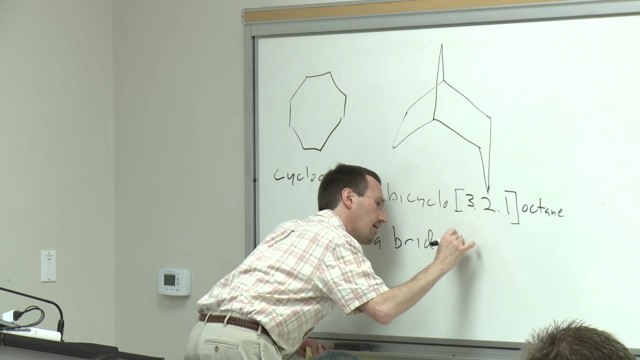 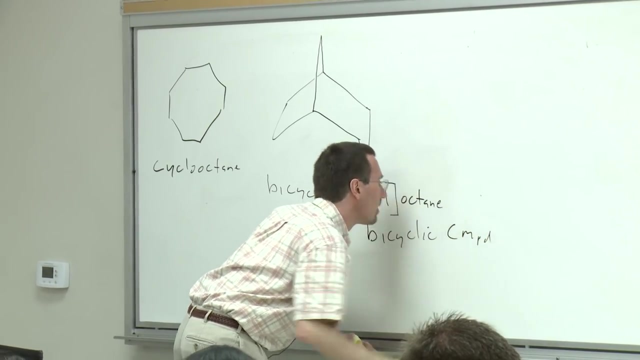 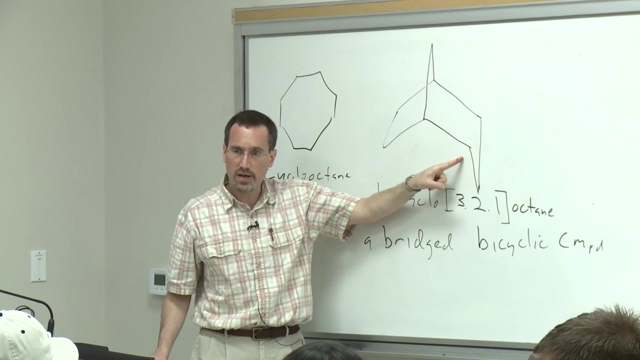 Close our bracket. All run together Octane, And it's sort of a cool example of what we call a bridged bicyclic compound. Now it has a three-carbon bridge, Which is where the three comes from, A two-carbon bridge. 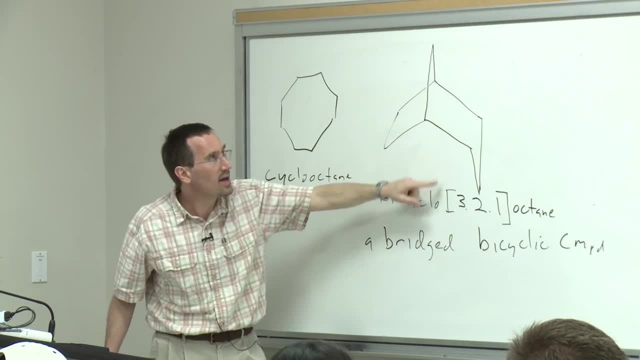 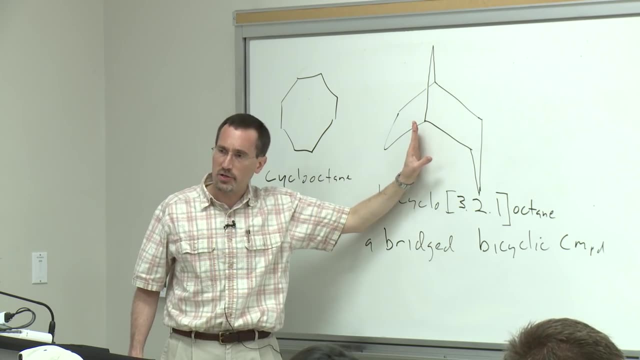 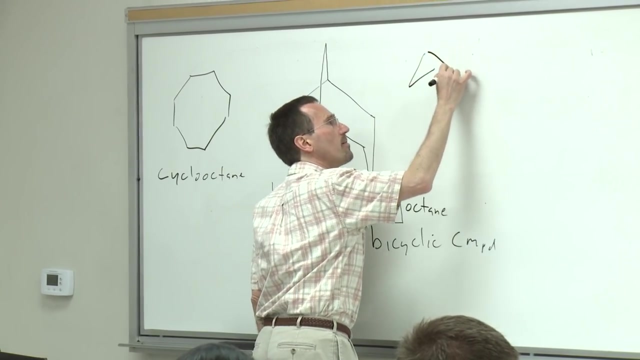 One, two, Which is where the two comes from, And a one-carbon bridge, Which is where the one comes from. This drawing very much like your drawings of cyclohexane Right. Everyone probably remembers this structure And hopefully everyone remembers. 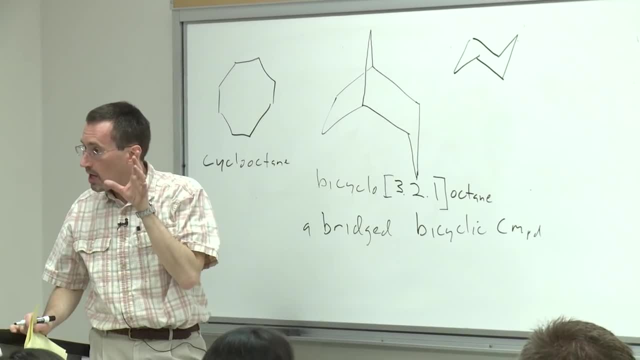 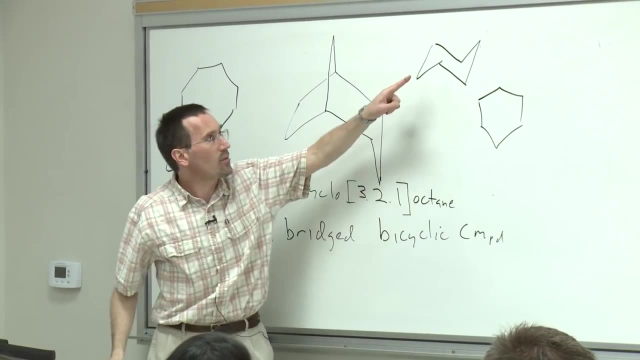 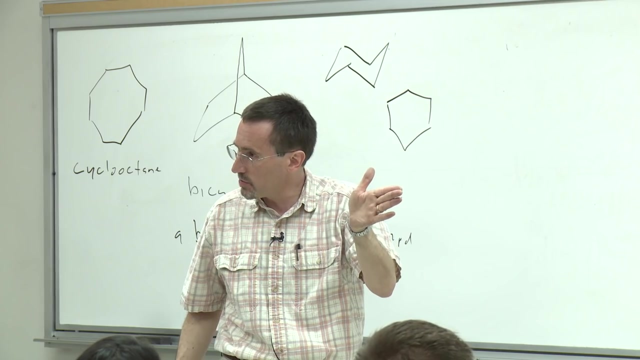 that the reason a chair cyclohexane is drawn that way, or can be drawn that way rather than just this way, is that when you put cyclohexane in a realistic conformation and look at it side on, that's what you see. 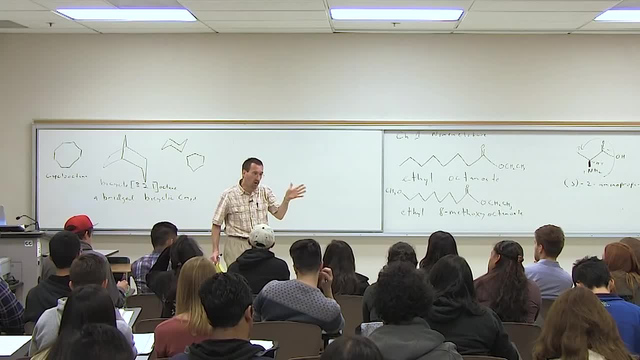 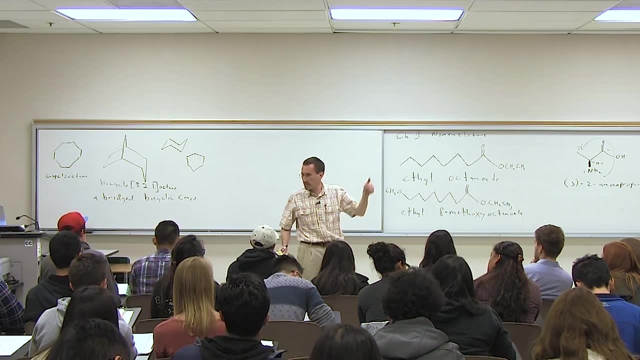 That is a projection of the structure. One of the things I like to do in my sophomore organic chemistry class is: take cyclohexane in a chair conformation, hold it on a big stick in front of the projection, with the projector on white. 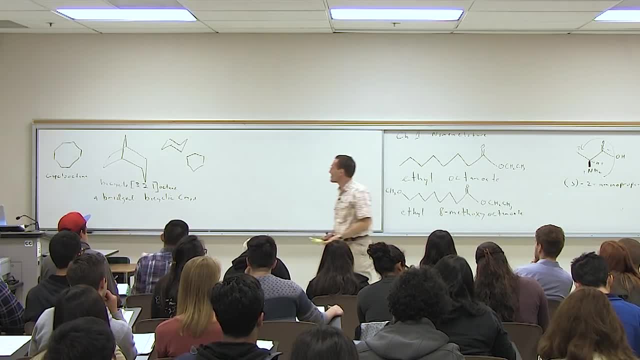 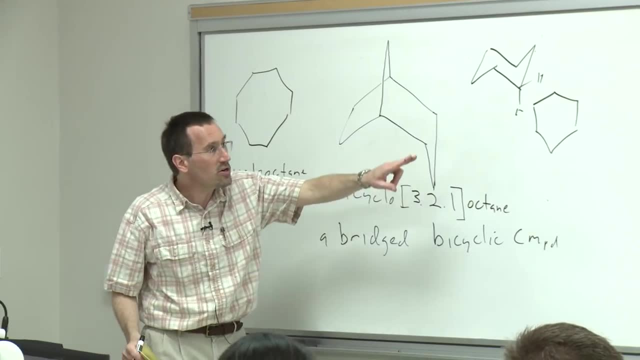 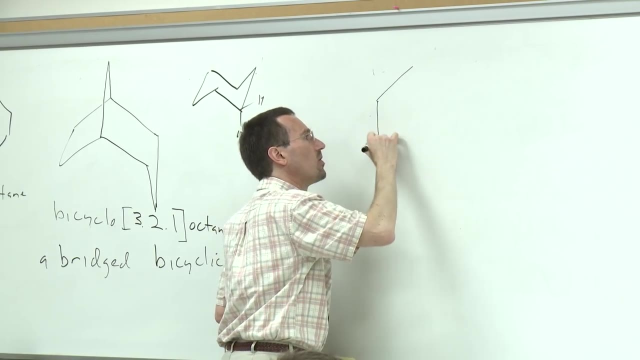 and you will see on the screen exactly that structure projected with the axial hydrogens and the equatorial hydrogens and so on and so forth, And you can also draw cyclohexane this way And similarly. we can go ahead and we can also draw our bridged. 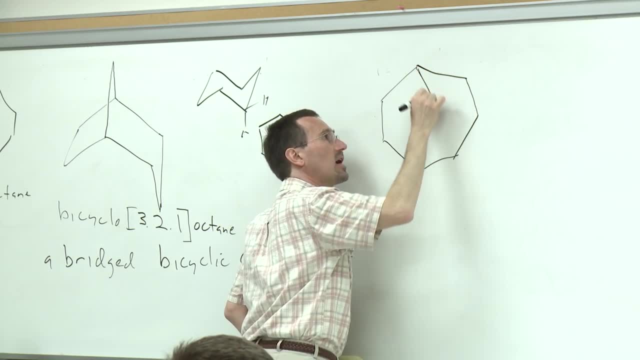 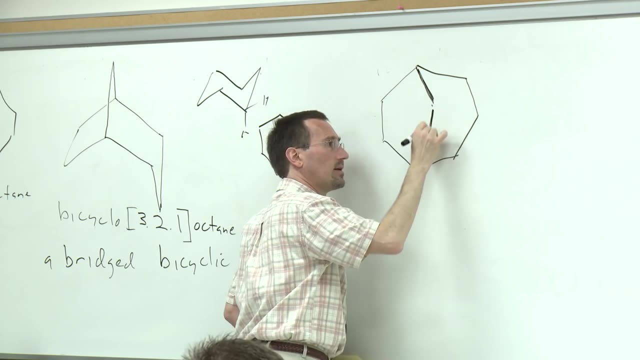 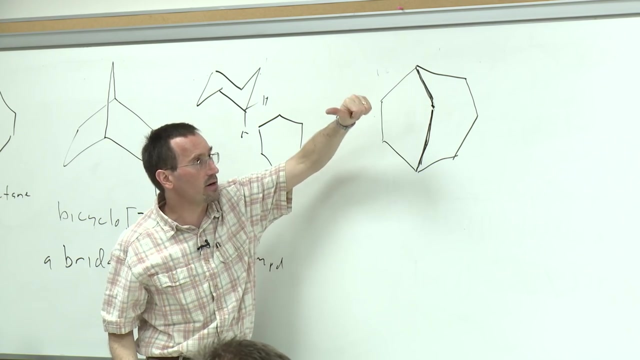 bicyclic compound in various other ways. So, for example, I can go ahead and draw it like so And I'm just showing that it's a wedge, which means basically our bridge is coming up here out of the plane of the page. 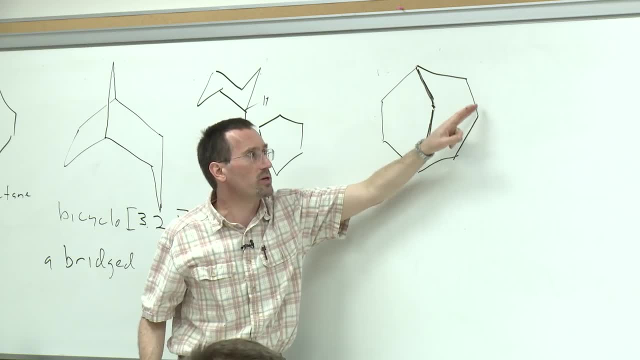 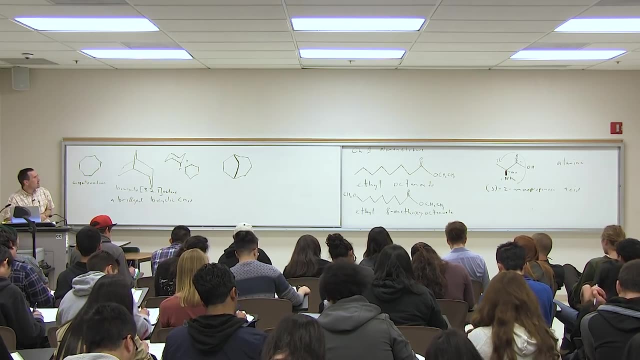 out of the plane of the blackboard. So there's our one carbon bridge, there's our three carbon bridge and there's our two carbon bridge. So I would like to do the same for you that I do with my cyclohexane. 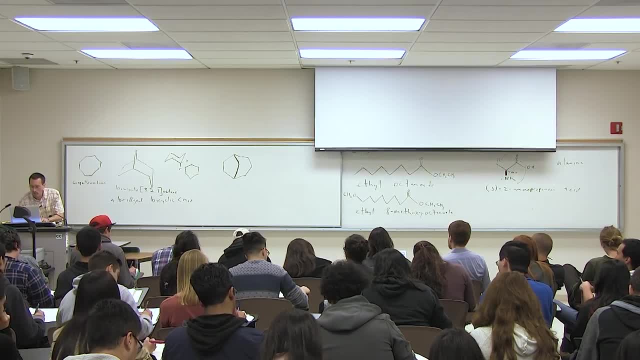 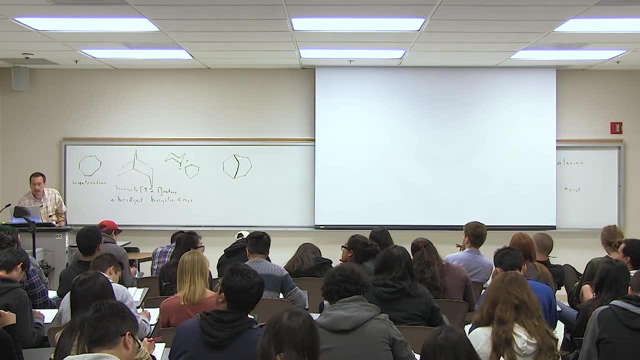 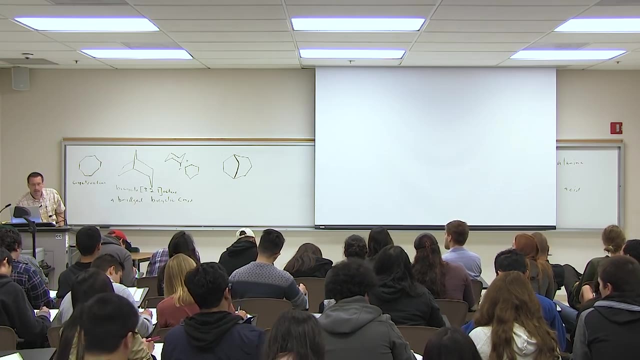 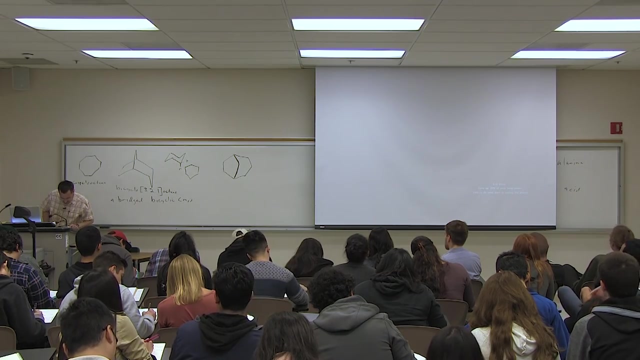 and so I'm going to go over here onto our website And let's see, I'm actually, I think, going to use that version of the website And I try to share my class materials. It helps if I turn on the projector, All right. 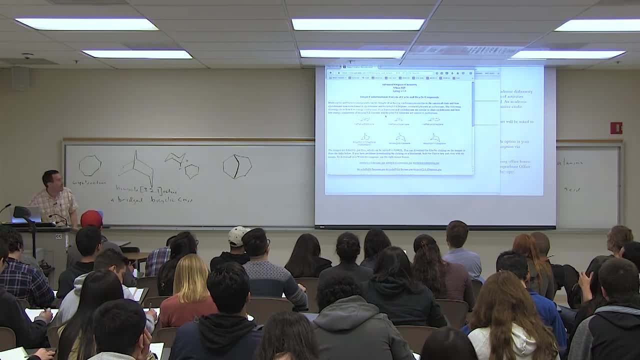 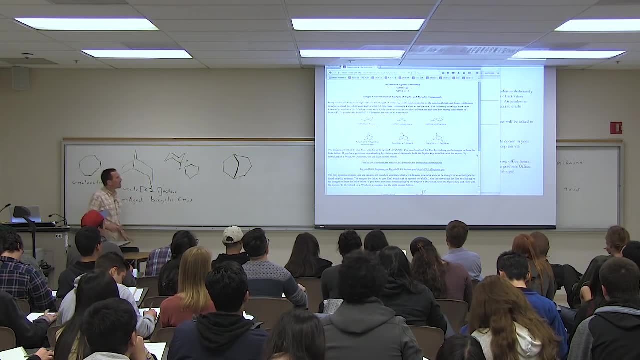 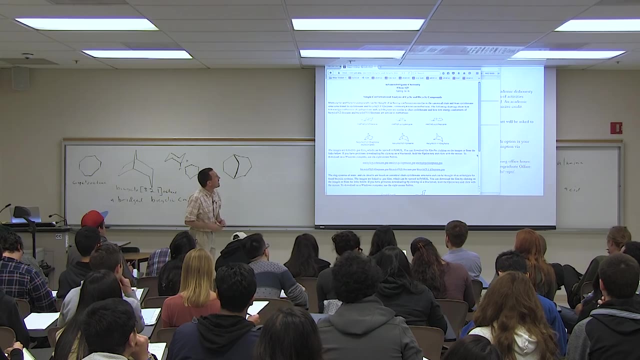 So I try to share with the class the materials that I create, And this is a little little demo I created on bridged bicyclic compounds and just a little bit of drawing to help show their structures. I there's various software where you can view various file formats. 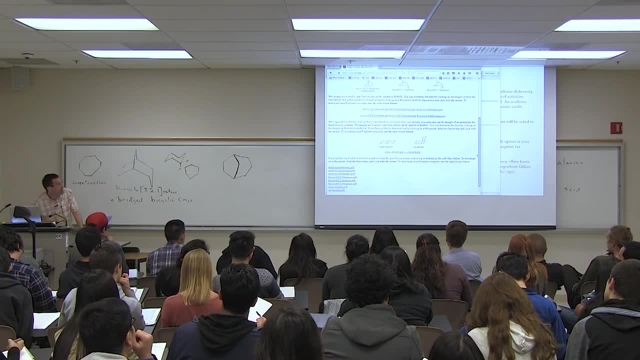 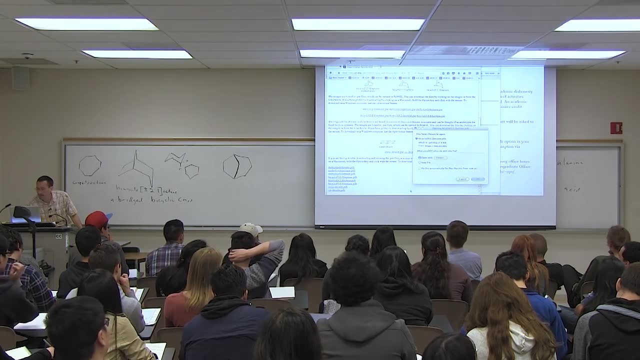 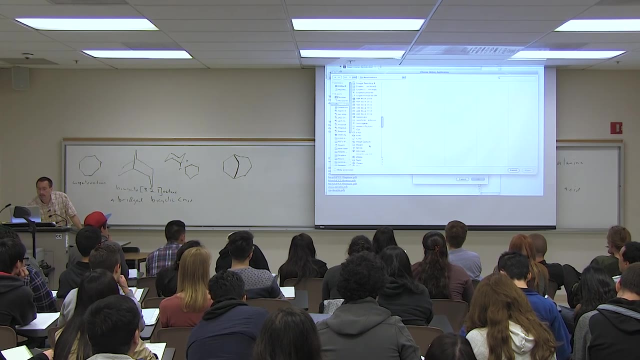 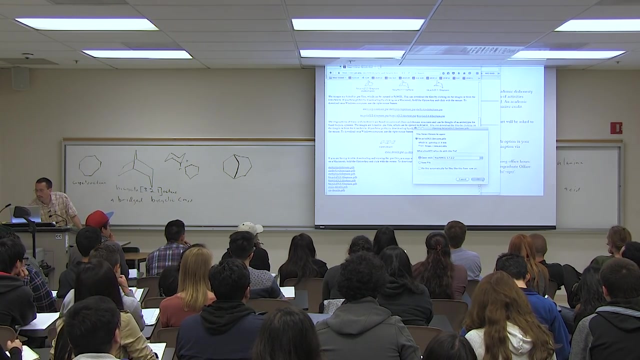 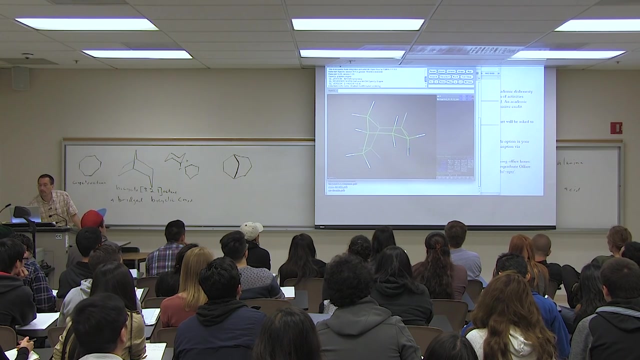 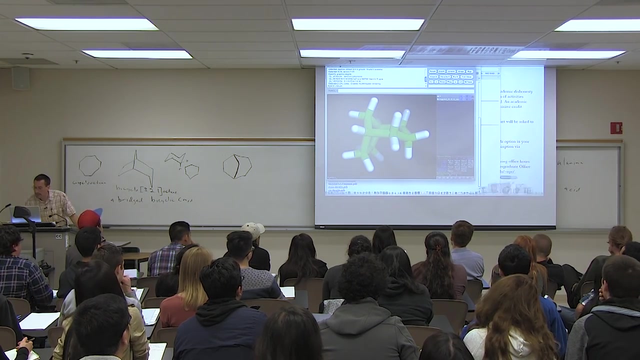 And the file format I like is called a PSE file format, But the one that works a little bit better is the PDB file format. All right, So this is basically, and I'm going to make this a little clearer. So this is basically the. 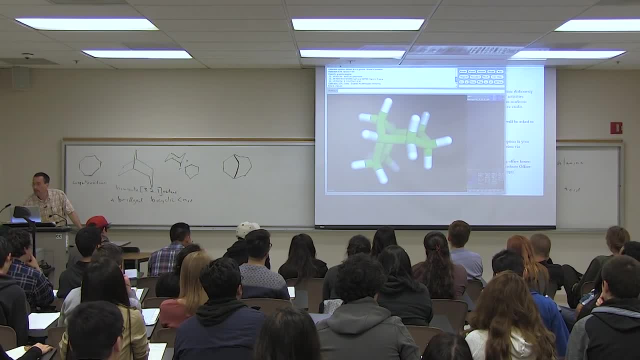 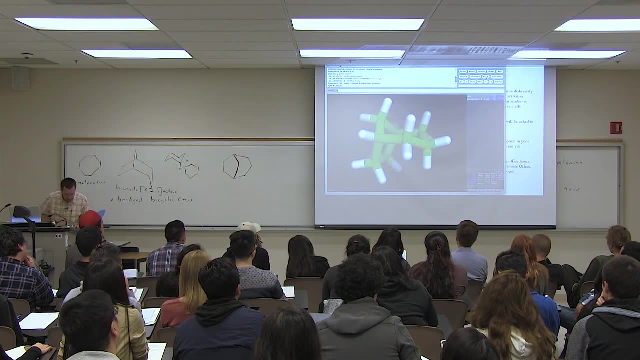 structure we are looking at here. It's what I've drawn And I think you'll get to see the three-dimensional shape of it a little bit better. if I get to move it here, Maybe I'll kill the front light here, So I'll let that rock. 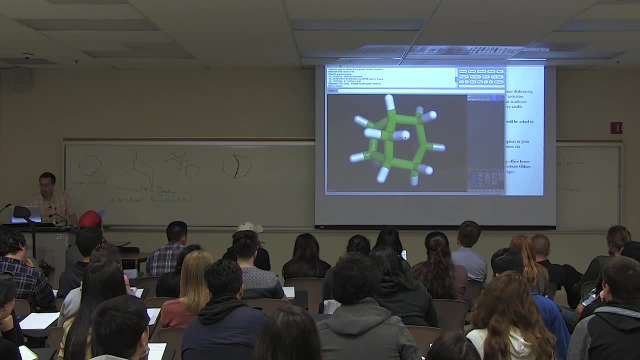 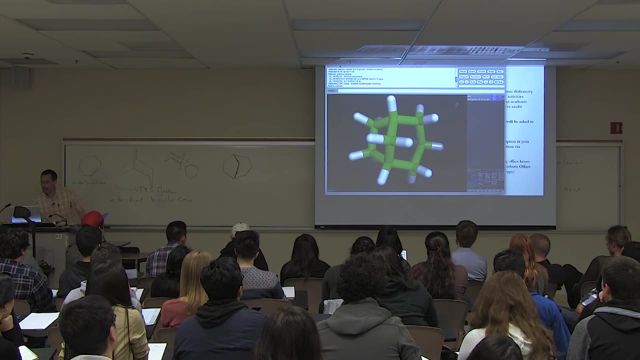 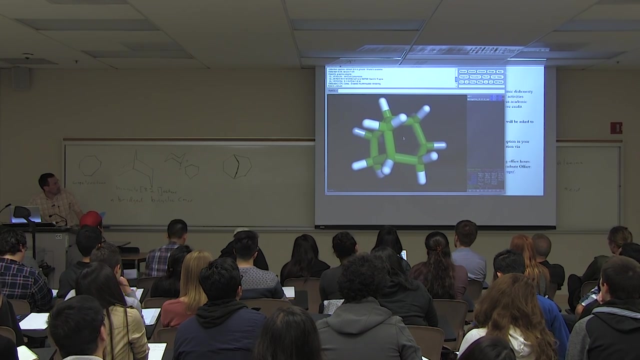 And I want us to be able to relate this structure to the structure I just made on the blackboard over here, The drawing over here, And I think you can go ahead and see how that relates. So, basically, what you're getting inside projection, what you're getting. 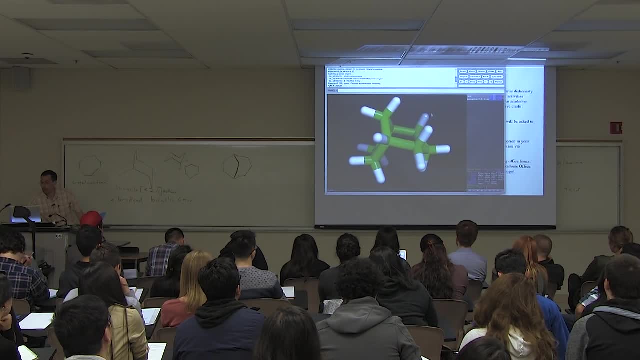 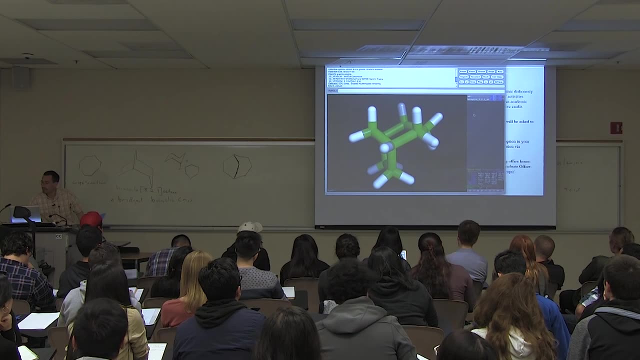 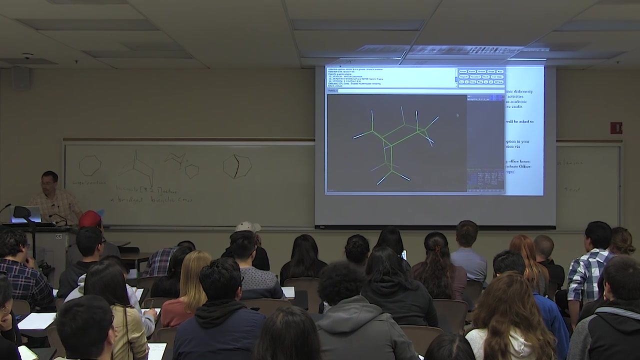 in profile is this structure here Now, the other thing that's sort of cool about this is if you look at this from a different perspective- and maybe I'll go to go to lines here- Okay, if you look at this from a different perspective. 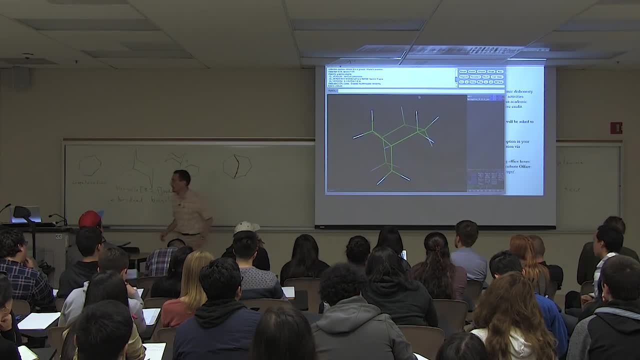 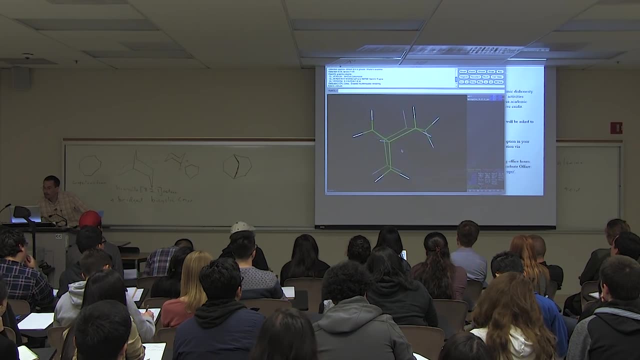 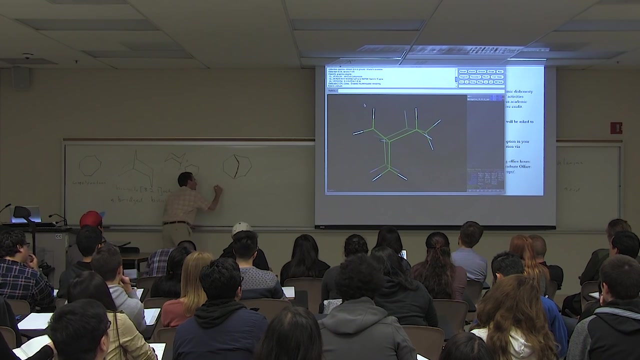 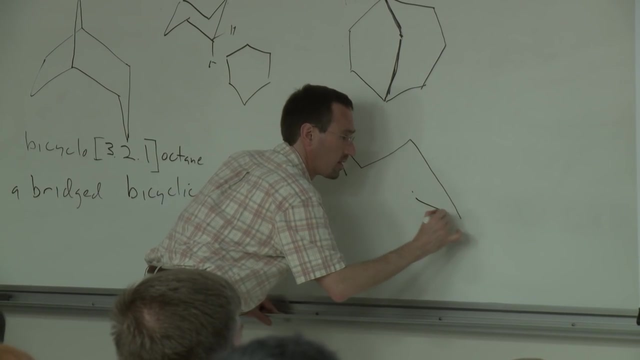 you can also realize: let's see if I can get that, get that good for you. There you go. Okay, you should also be able to recognize that essentially what we have is a chair, cyclohexane with a two-carbon bridge. 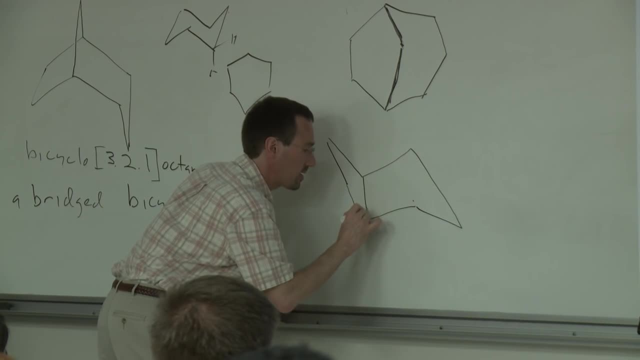 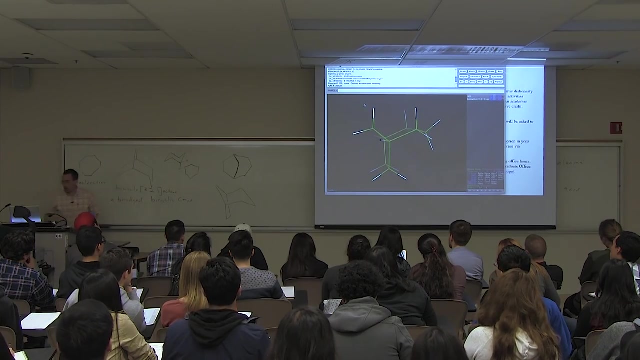 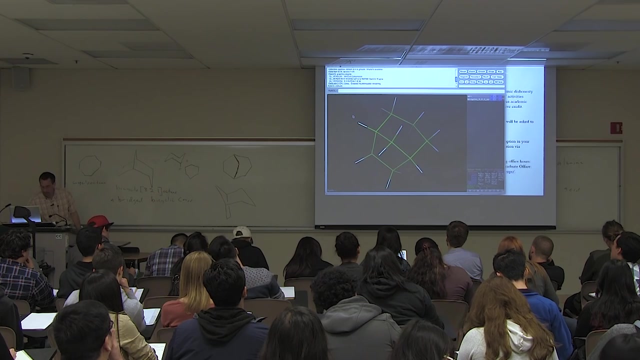 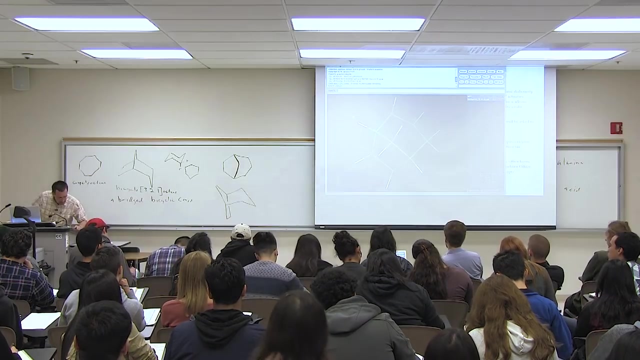 across it like so. Anyway, all of these three-dimensional structures really have much more meaning when you're able to visualize them in your head. I strongly urge you to go ahead and look at these three-dimensional structures and see how they work Also. 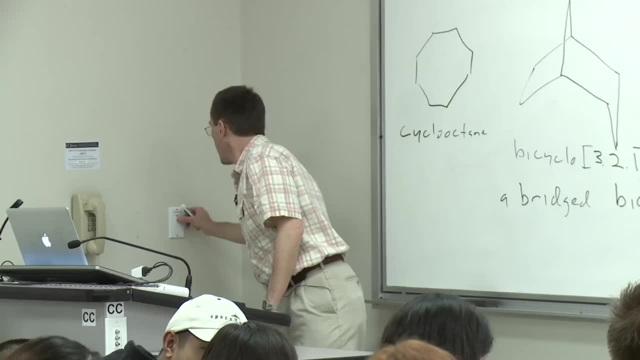 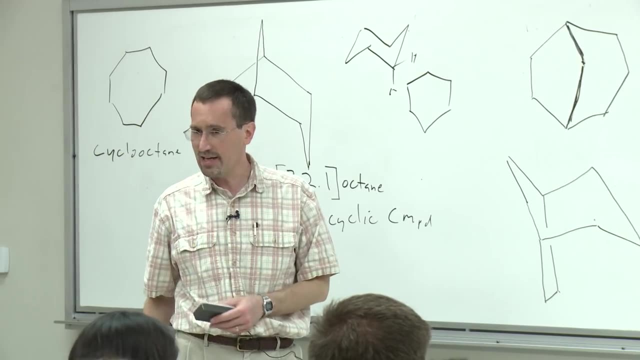 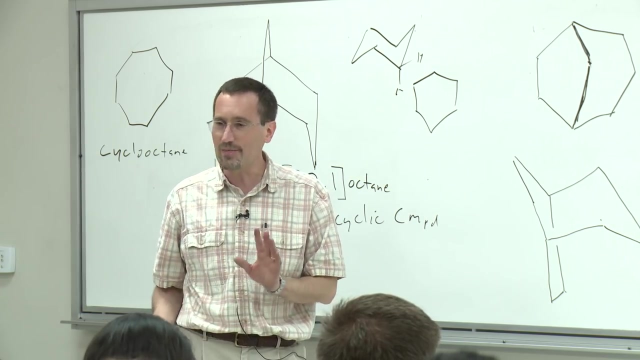 get out your plastic models that you got with your sophomore kit and feel free to play with them. Now the software I got- it's called Pimole, One of the cool things. I paid, I think, 760 bucks for the license for it. 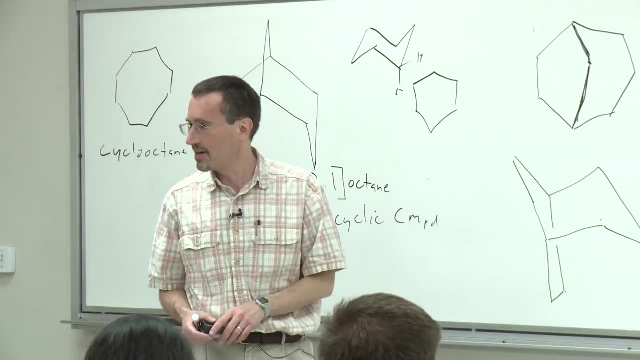 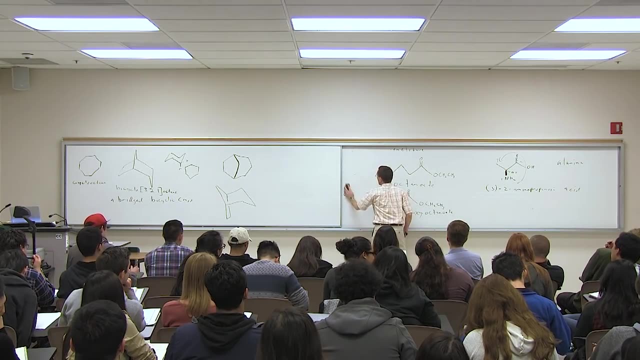 One of the cool things about it is that it allows me to give it to all of my students. so you've got a lot of other things on your plate, But if you want to play with those molecules or even build your own structures, you can. 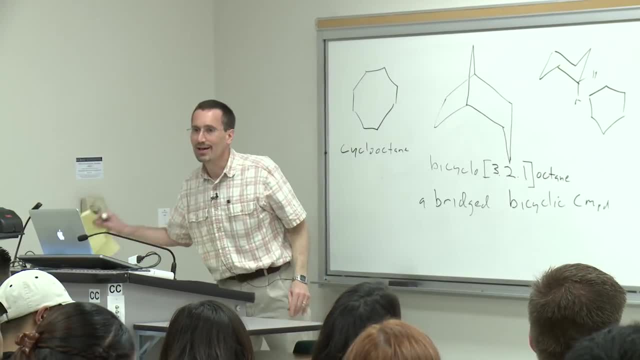 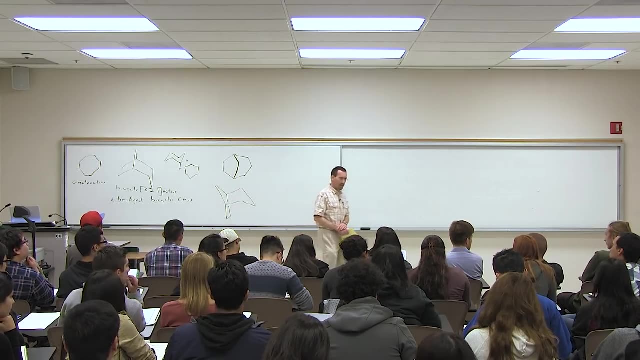 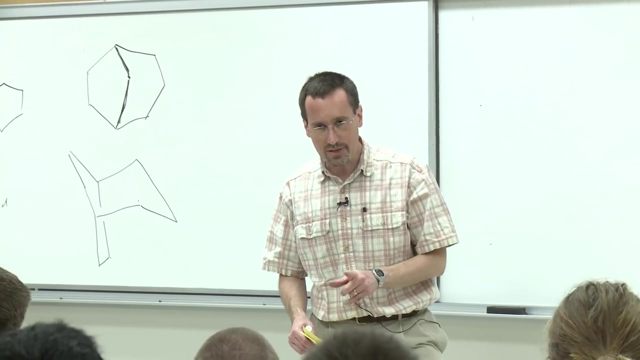 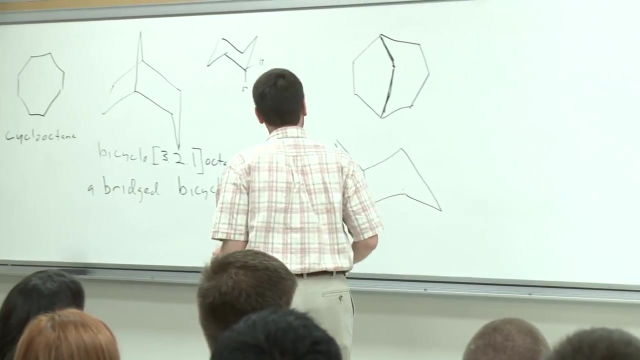 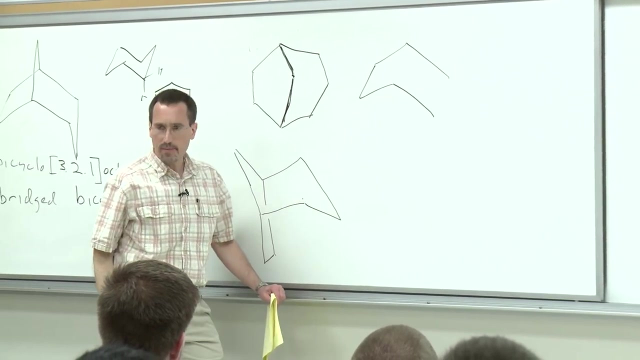 Thoughts or questions at this point. Yeah, I think what you're saying you're asking is: Oh, I understand. Yes, yes, yes, Now I understand what you're asking. When I was setting up to think about how I wanted to teach this to you, 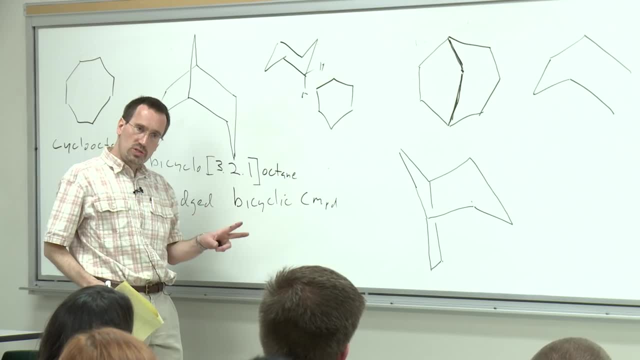 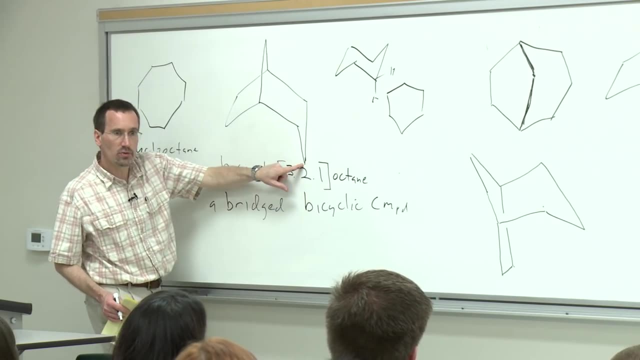 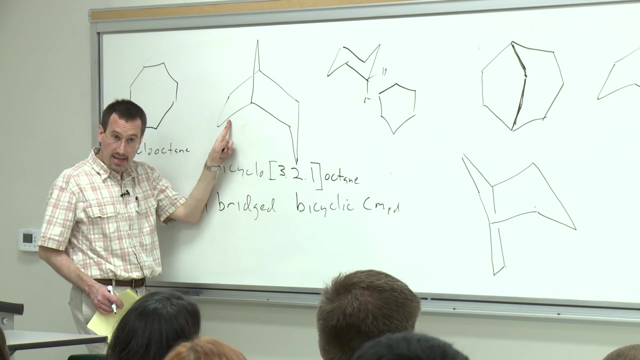 I decided to draw this in the most common realistic confirmation. And so the question you're asking is: you look at this three carbon bridge down here and you look at this bridge and you say it's banging into it And this is a molecule where you are damned if you do. 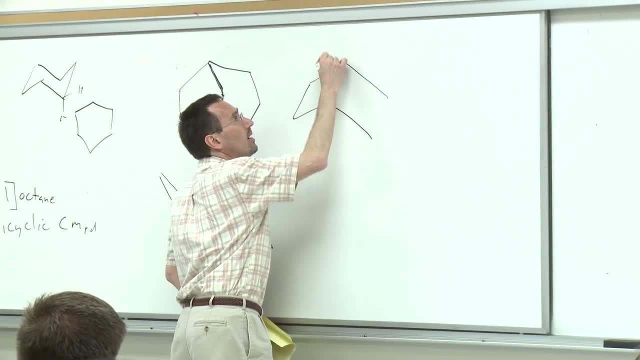 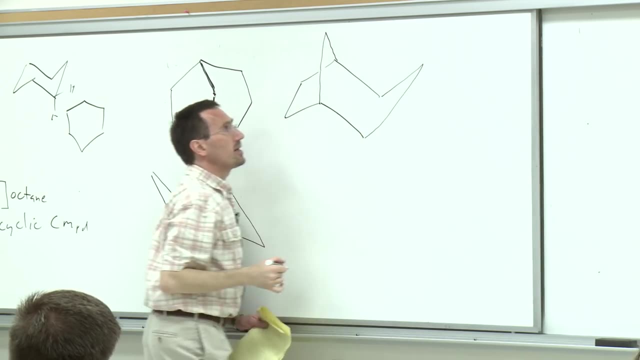 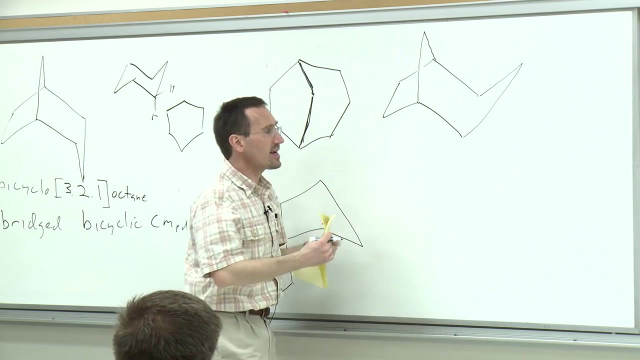 and damned if you don't. And I'll show you exactly what I mean. Okay, so the short answer to your question, which is right on the mark, okay, the short answer is this, is another reasonable confirmation. And they both have problems. Do you recognize? 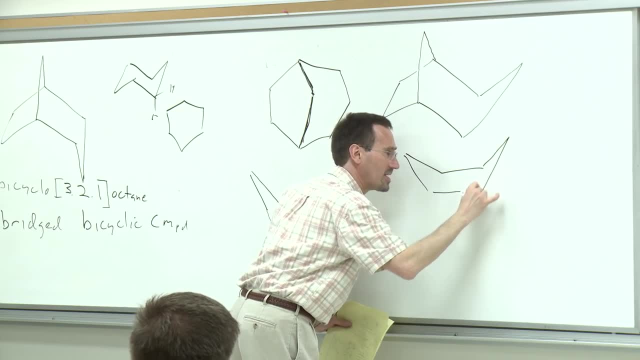 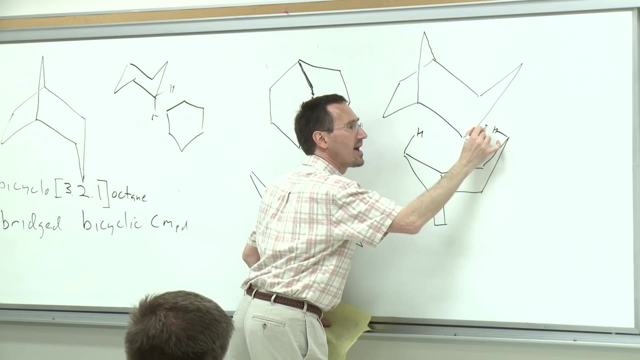 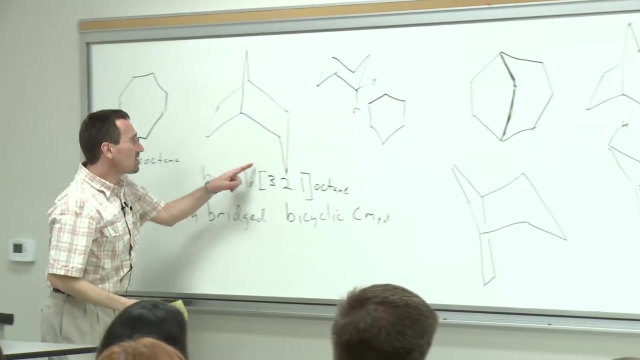 this structure here, Boat, yeah, So this, this is a boat, which is bad because this hydrogen bangs into that hydrogen. There are a lot of other bad interactions as well. This is also bad because this hydrogen here which is now. 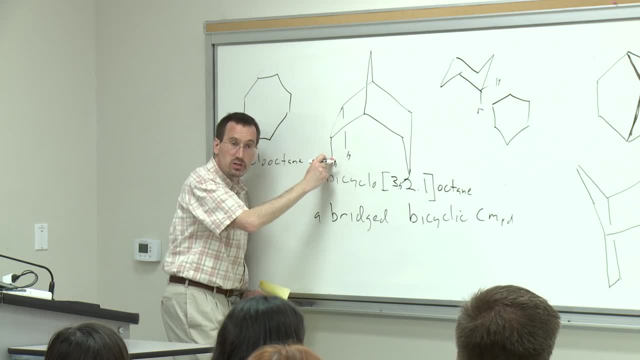 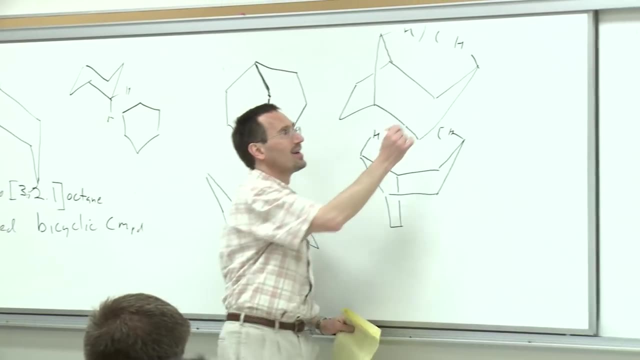 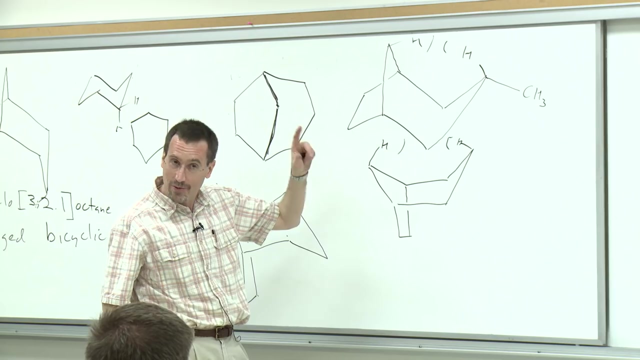 right over the three bangs into these bridging hydrogens, but not quite as badly. But imagine we had a methyl group at this position. Then the lesser of the evils would be to put that methyl group there. So indeed it can flip, And when it's? 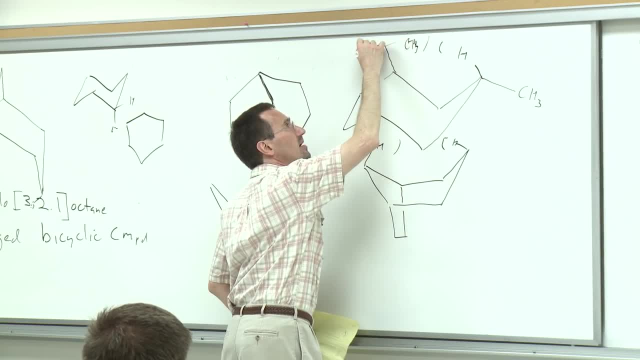 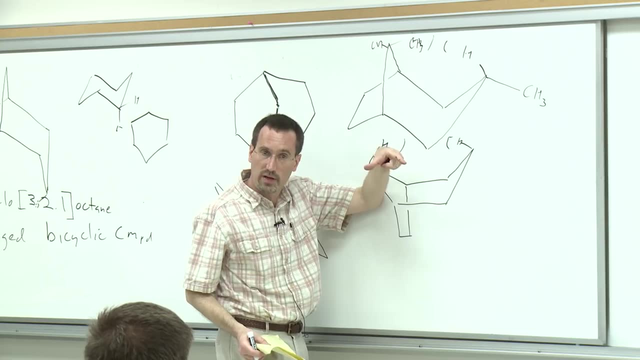 really damned. for example, if you have a methyl group here and a methyl group here, what happens is this ring flattens out a little bit, It gets a little bit more eclipsed, a little bit flatter than a regular cyclohexane. 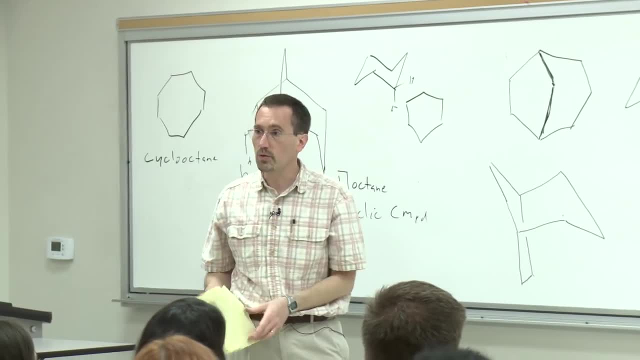 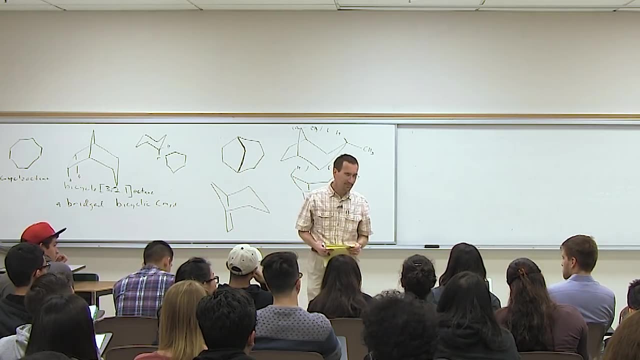 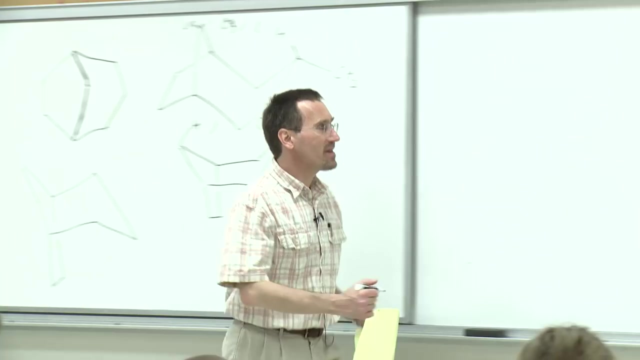 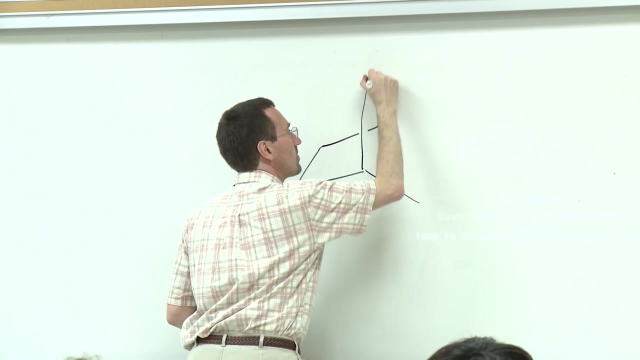 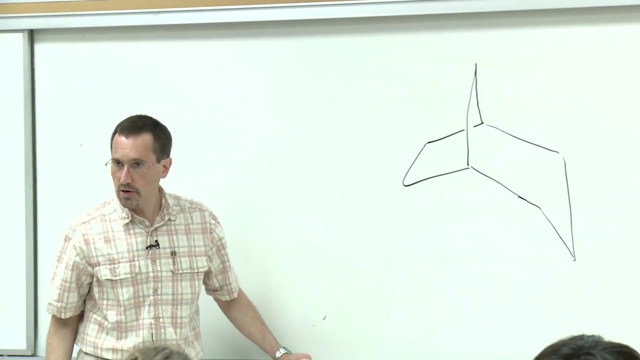 Absolutely insightful question. brilliant question. Other questions: A bridge just means one. okay, so let's talk about the anatomy of the ring. Alright, so it is not a basic review question because you haven't seen this in your sophomore class. Okay, so here's our ring. 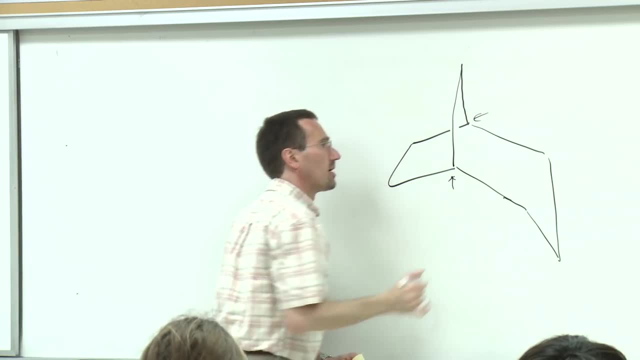 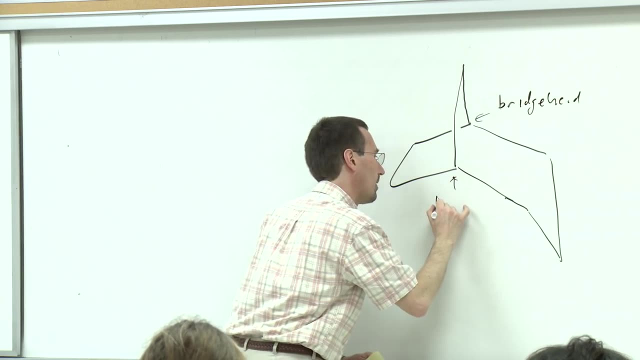 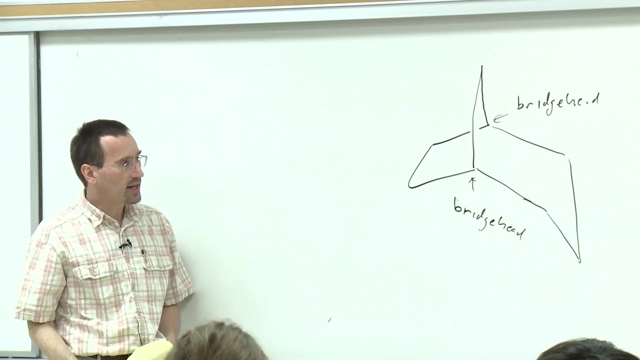 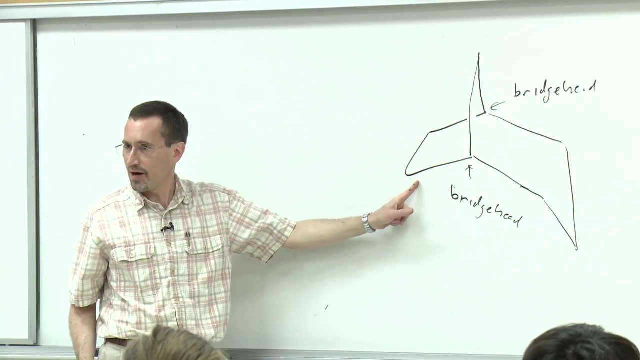 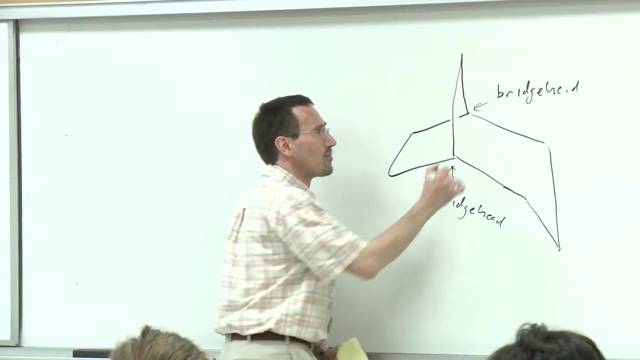 again, We call these joining points bridge heads, And three bridges connect the bridge heads. A three carbon bridge, in this particular example, a two carbon bridge and a one carbon bridge. Now let's get into the details of numbering. So bicyclics. 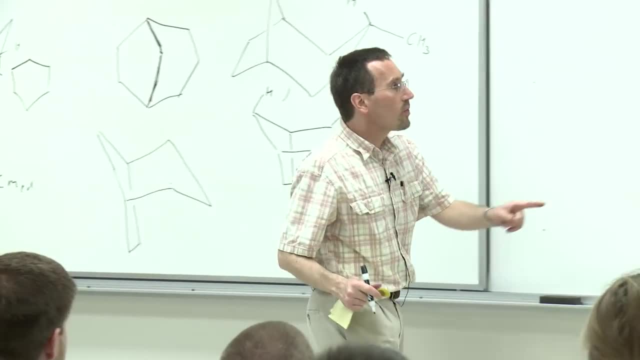 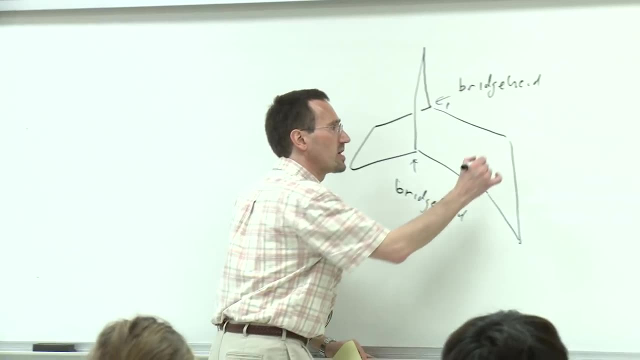 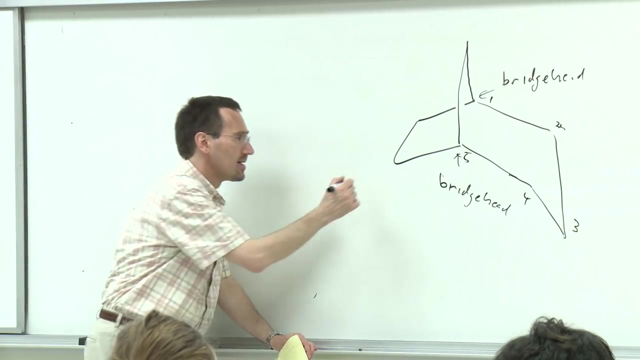 have a curious way of numbering them. We start numbering with the bridge head, Then we number around the longest bridge. So we go one, two, three, four, five back to the bridge head, Six onto the next bridge And finally. 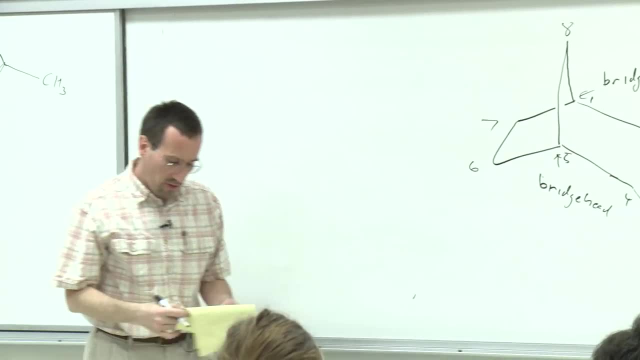 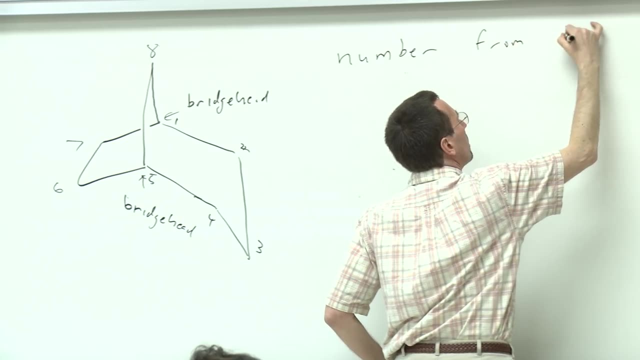 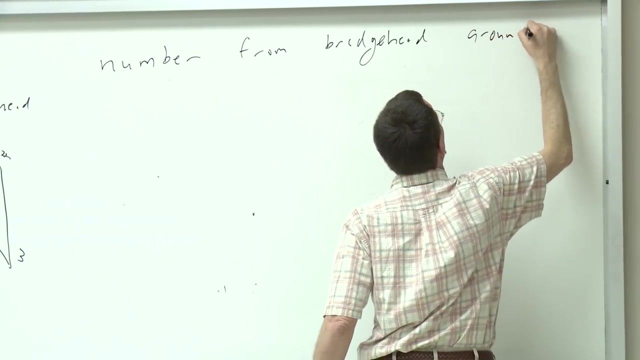 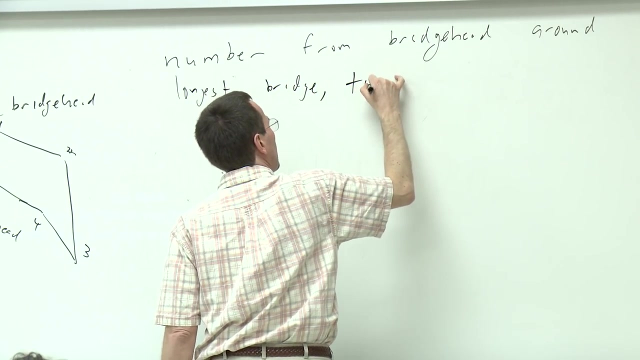 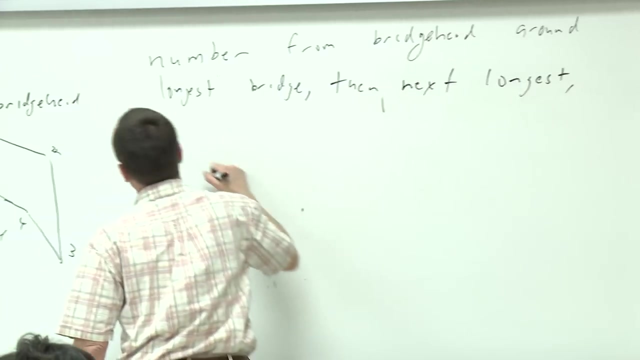 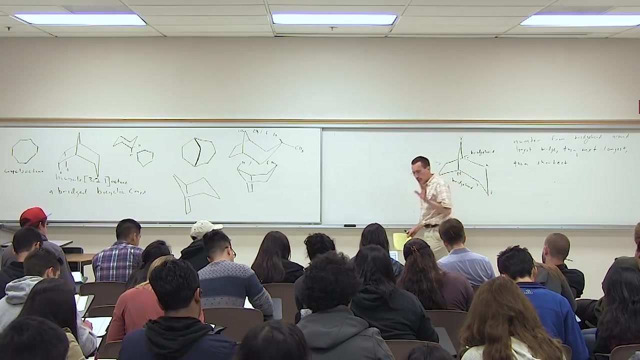 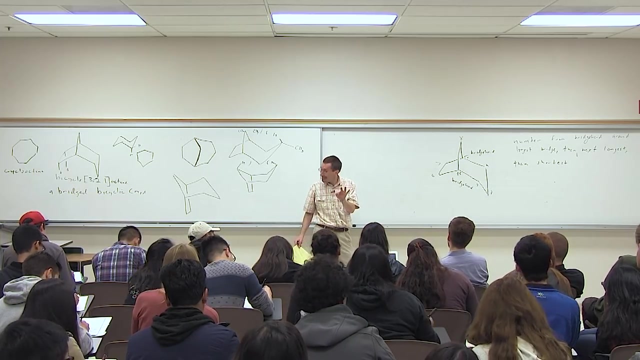 onto the last bridge. So we number from the bridge: head around the longest bridge, then next and then shortest. We're going to see three in the case of molecules. today and next lecture, we'll see three slightly contradictory systems for three classes of molecules. We'll see one set of rules for bridge bicyclics, Bicyclics in general, One for spirocyclics and one for fused aromatics. Don't ask me why. Alright, so now, the smallest bridge defines a face. 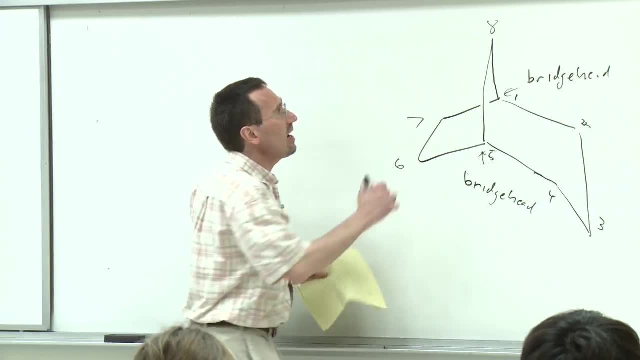 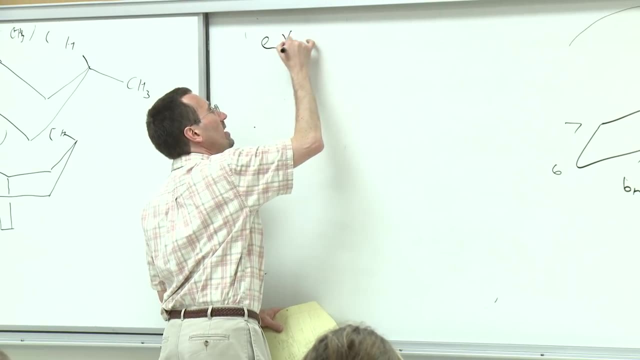 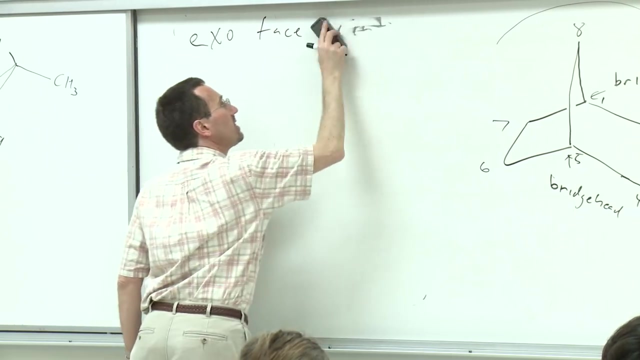 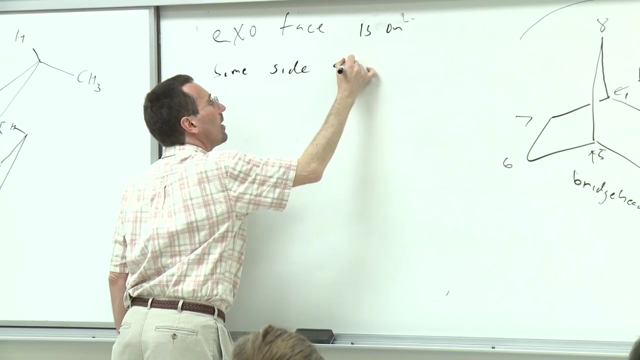 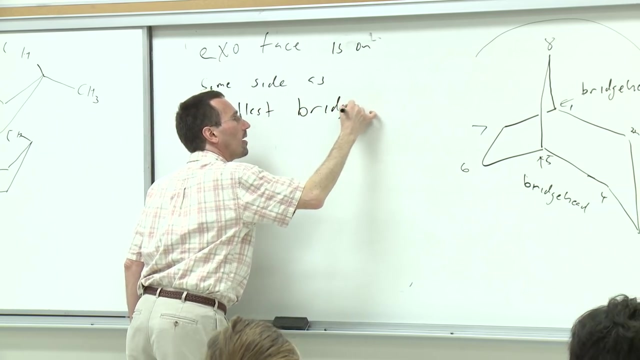 and so basically you've got sort of a convex face with the smallest bridge and we call that face. the exo face, I'll say, is on the same side as the smallest bridge, So this is our exo face. So a hydrogen that's pointing. 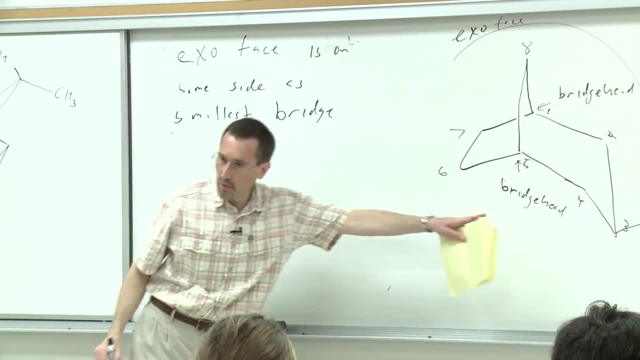 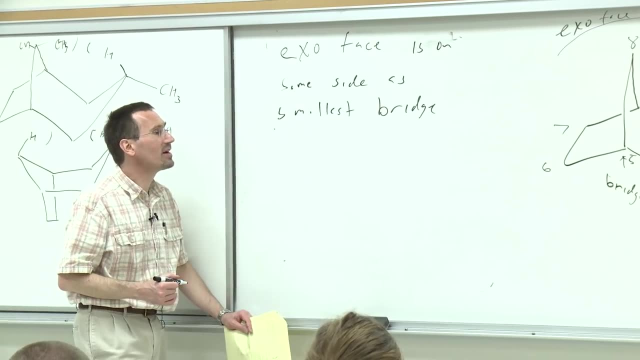 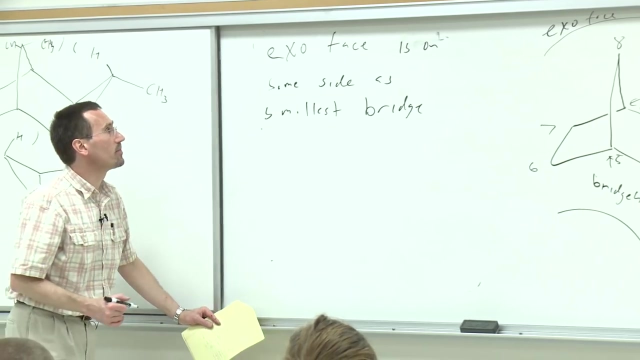 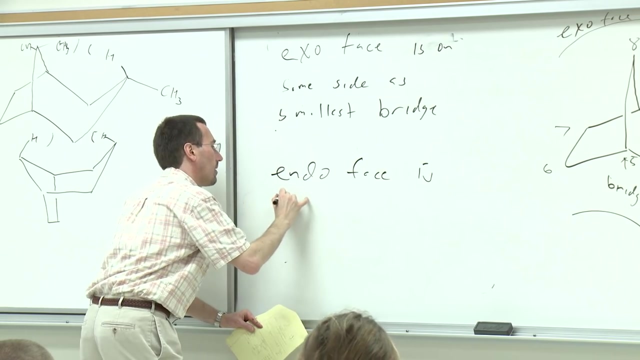 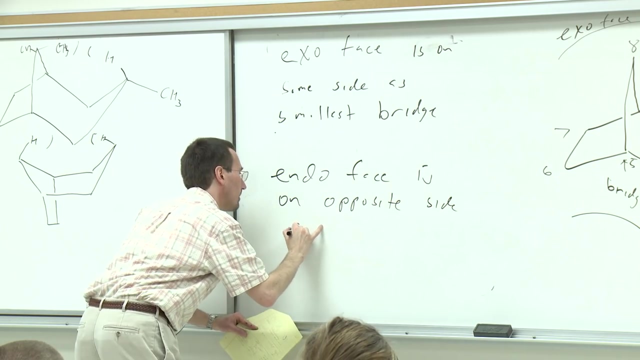 onto that face would be an exo hydrogen, just like you have an axial hydrogen or an equatorial hydrogen. The other face, if you will, sort of the concave face, the face opposite the bridge, is the endo face And I would say 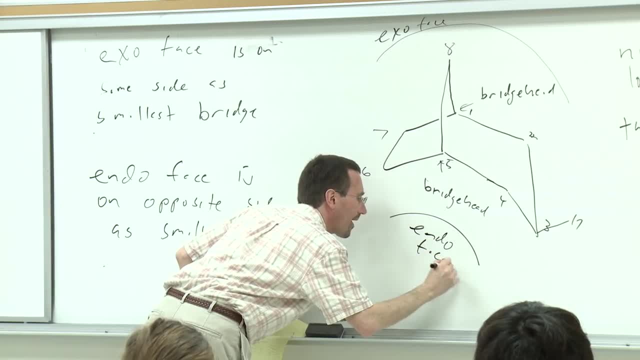 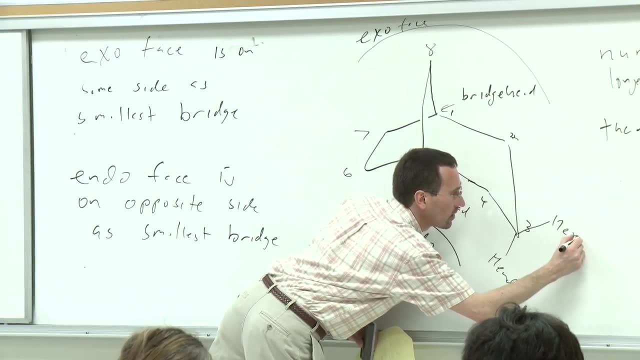 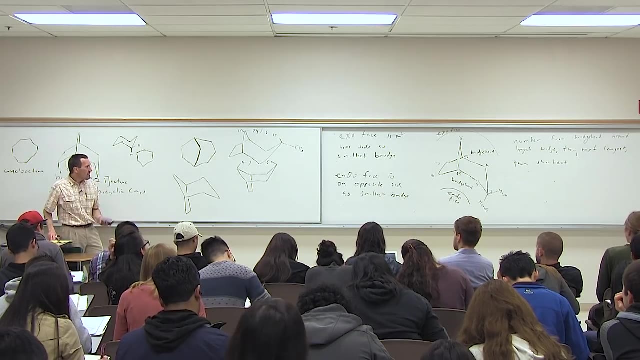 so this hydrogen- here we'll just call it H endo, and this hydrogen- here I'll call it H exo, And I would say, these concepts that I've just laid out here, these are probably what I would call second nature to a practicing organic chemist. 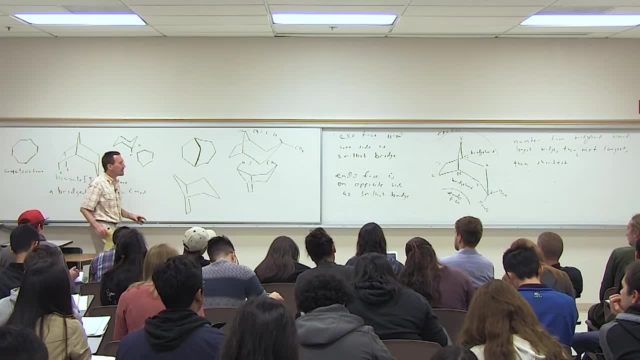 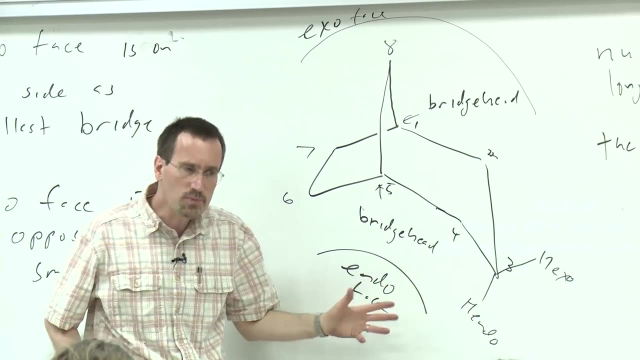 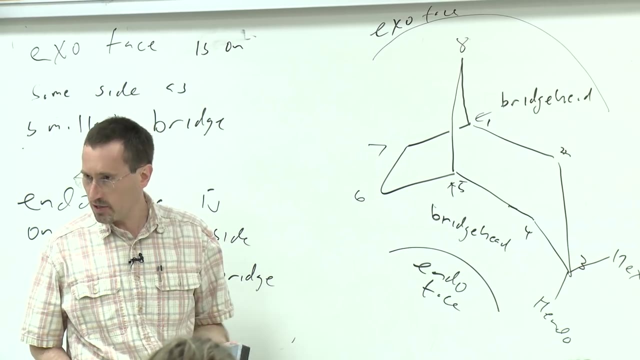 In other words, this level of knowledge. oh yeah, that's a bridge head. that's the smallest bridge. that's the endo face. that's probably second nature. Later on, when we talk about stereochemistry, I'll probably mention Brett's rule. 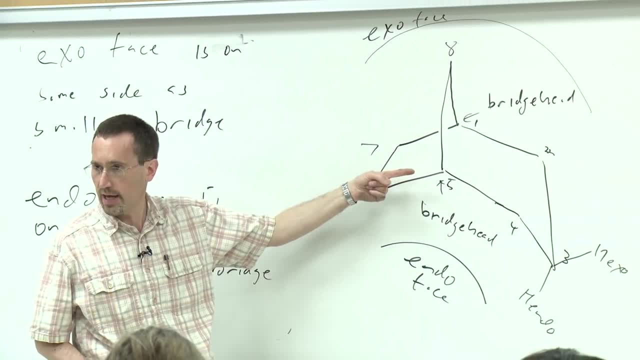 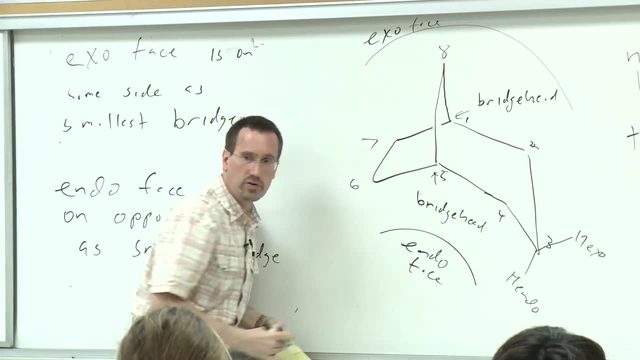 Brett's rule is that in a small bicyclic compound you can't have a bridge head alkene, and we'll talk about geometry and why. In other words, I can't have a double bond, say over here it's too strained. Bridge head alkene is probably 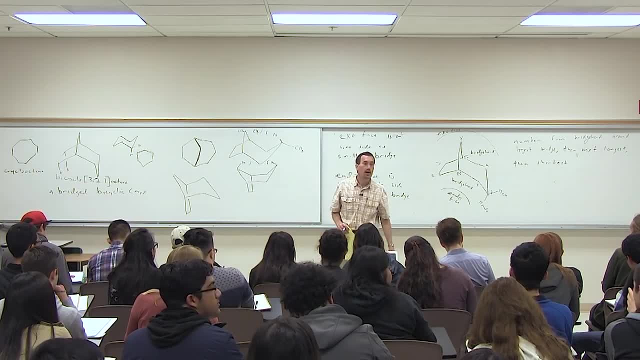 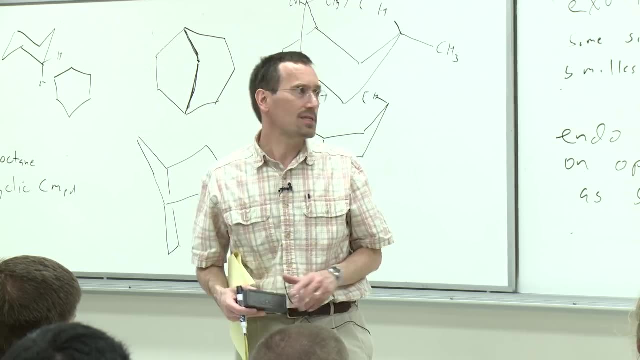 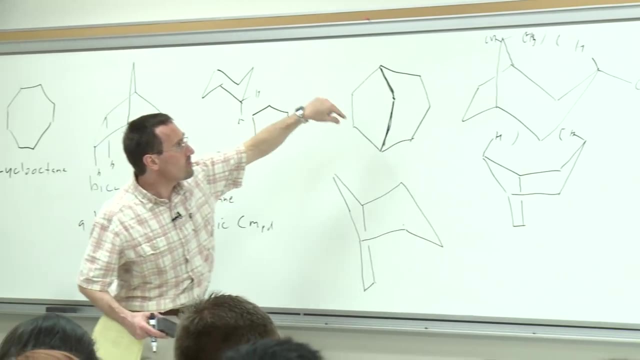 an idea that would roll off most organic chemist heads. I guess you can say: okay, again, let's think anatomy and let's come back to this drawing over here. So the biggest ring in the molecule is a seven membered ring. So imagine now we're defining 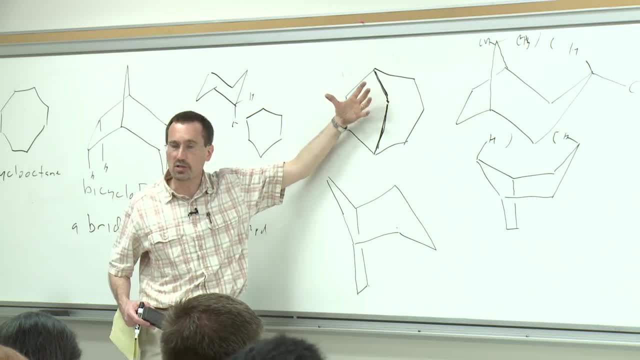 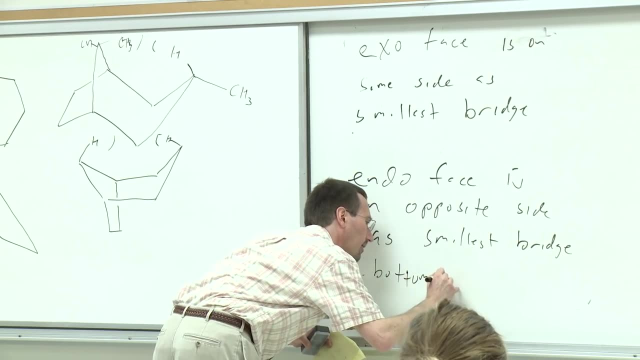 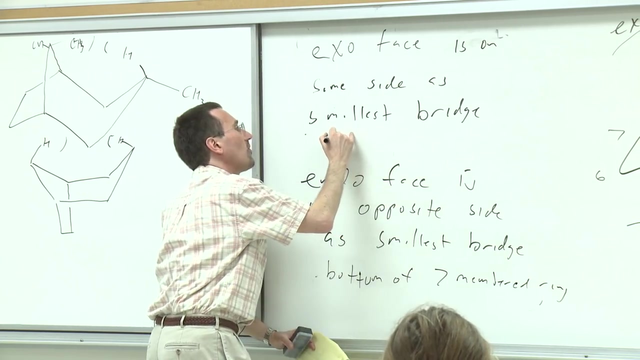 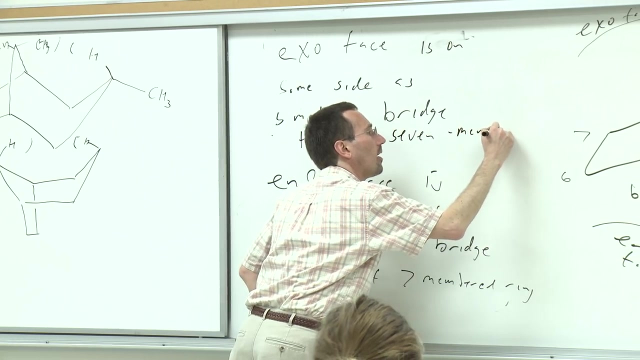 the top and the bottom of the seven membered ring. So basically, the endo face is the bottom of the seven membered ring And the exo face is the top of the seven membered ring. So yeah, there really are two faces. 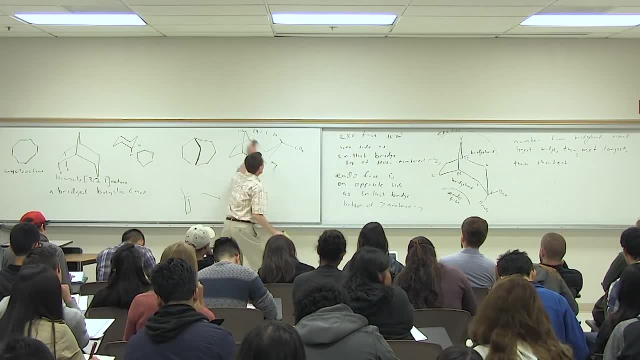 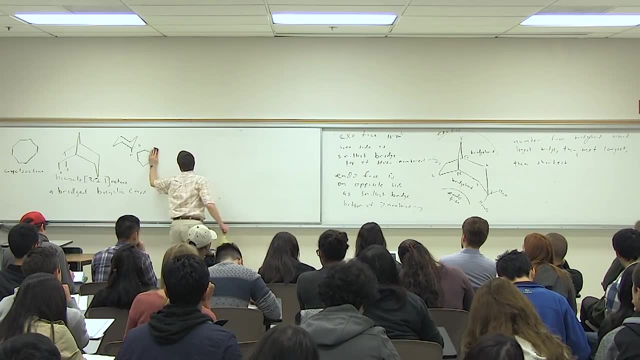 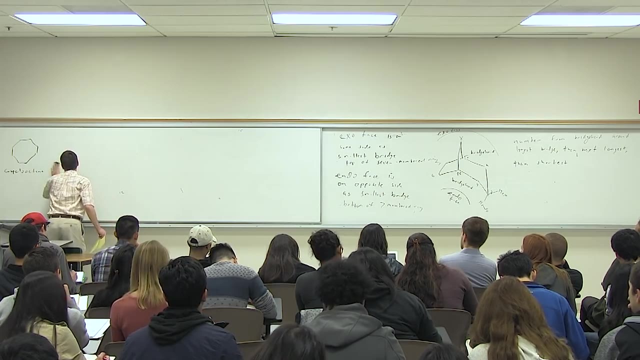 Now your textbook gets beyond this. Your textbook gets into trying to figure out how to use bicyclics and so forth, And I guess my feeling at this point is for us spending only a couple of lectures on it. read it, let it pass over your eyes. 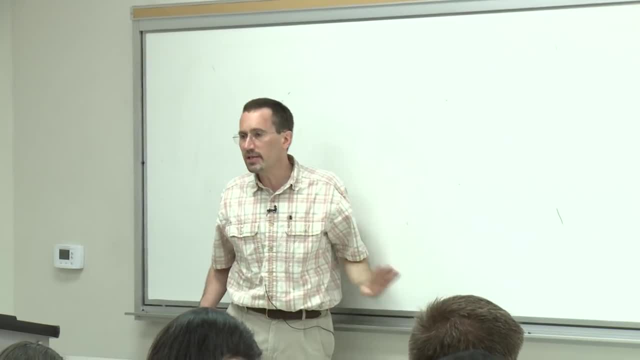 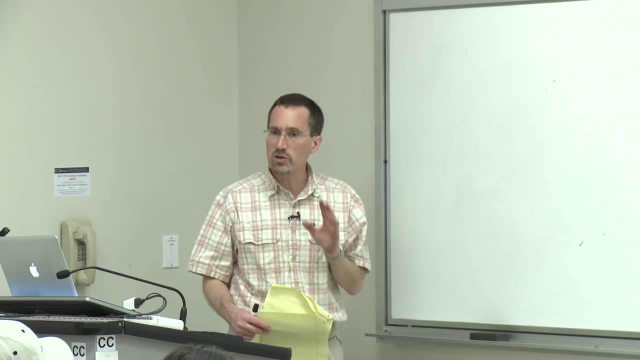 see if you can make sense of the examples. But honestly, if you can get bicyclics down at this point, I'm really happy with that level of mastery. You'll be able to flip back to that and say, oh, wait a second. 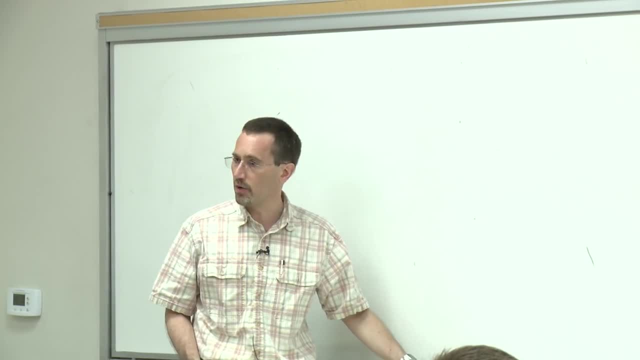 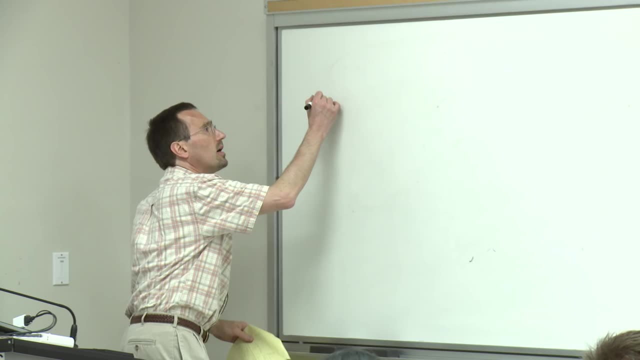 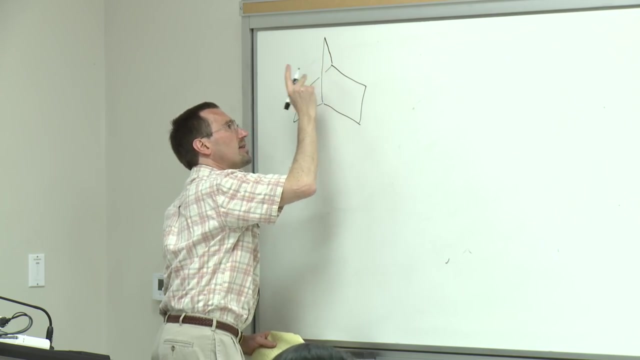 I saw tricyclics once. I saw how you deal with additional features in the molecule. Alright, I want to come back to some substituents here And I'll give us a different molecule. Have a little bit of fun. 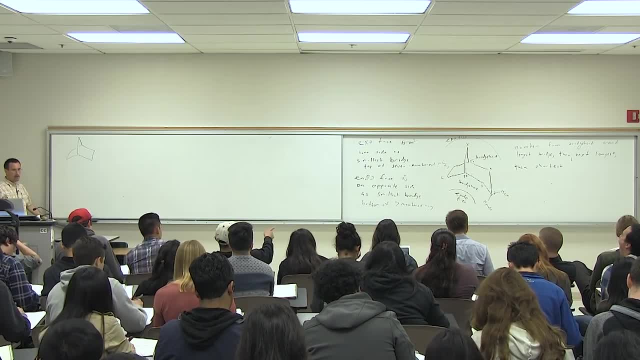 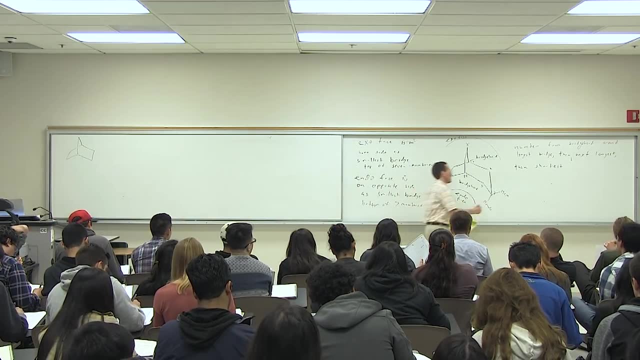 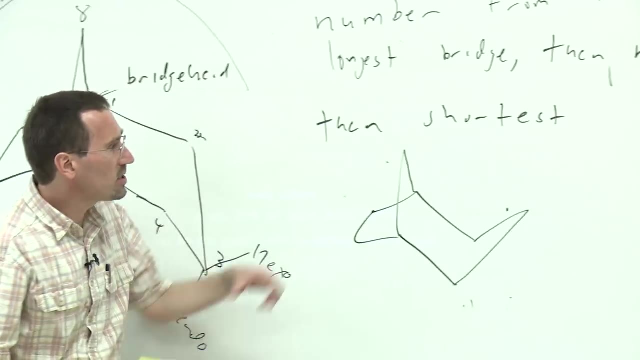 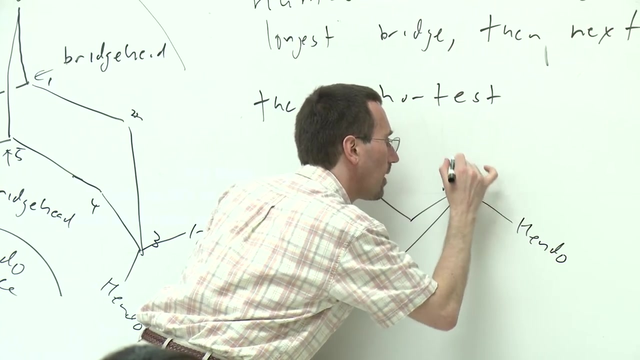 Yeah, Are you only able to determine through that chair conformation, Regardless, even if it's flipped up, even if it's flipped up because it's because we're defining face opposite the bridge, this is still. that's still the endohydrogen. 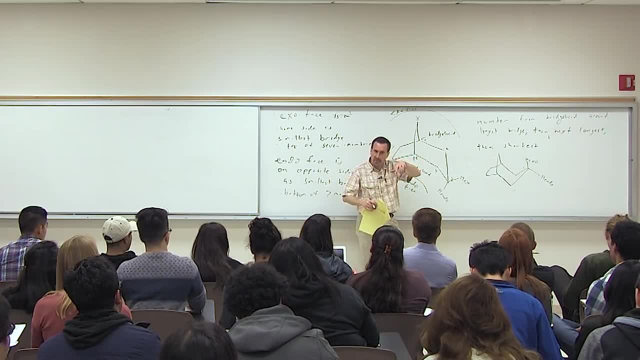 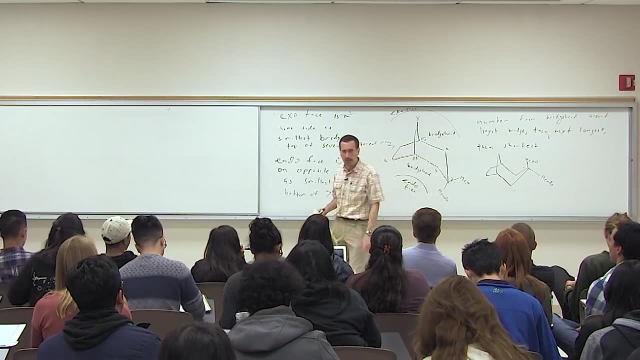 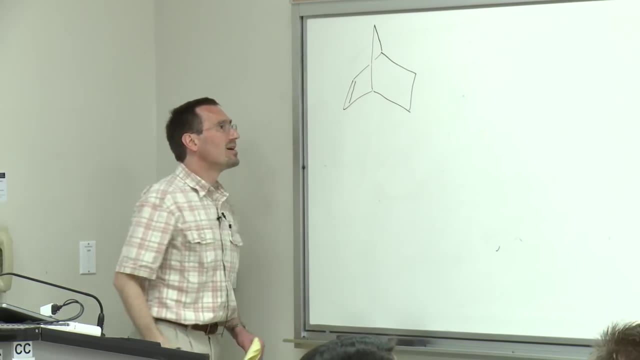 Even if the whole face isn't perfectly concave, it's the bottom face, Opposite the bridge, bridgehead, And that's basically what's meant. You're welcome, Alright, So somebody, based on what we've learned so far, 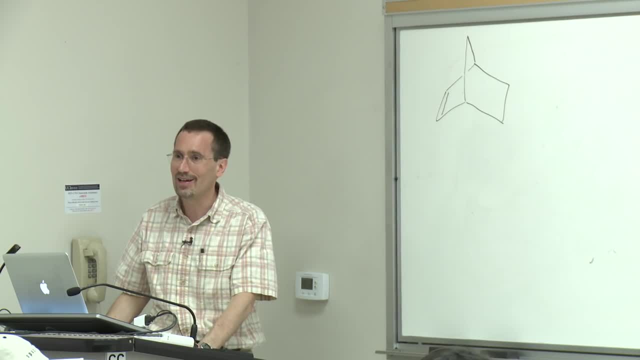 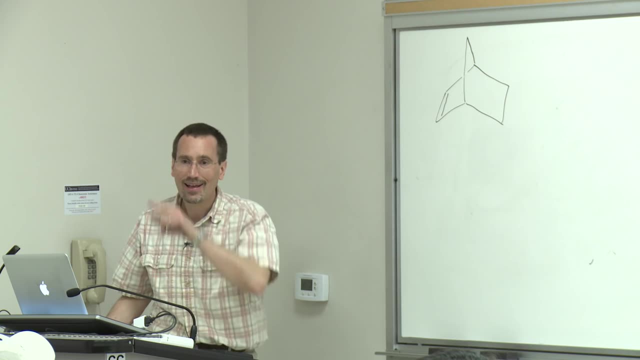 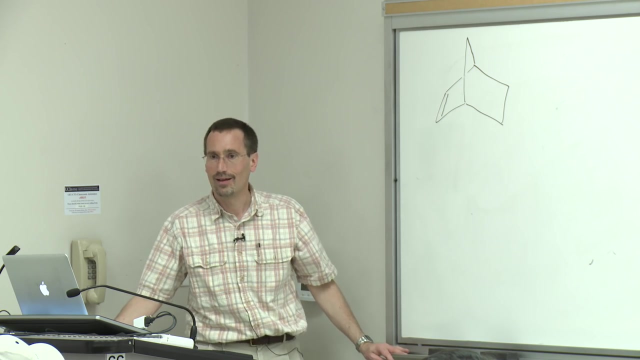 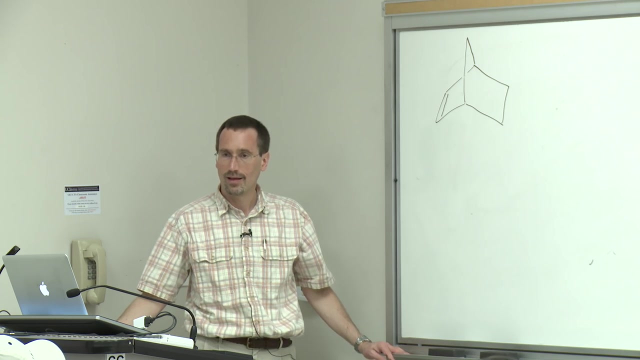 take a stab at this structure. What would we call it? 3, 2,, 1, 6, uh, uh, the bicyclo 3, 2,, 1, 6, 2, 2? 2, 2, yep. 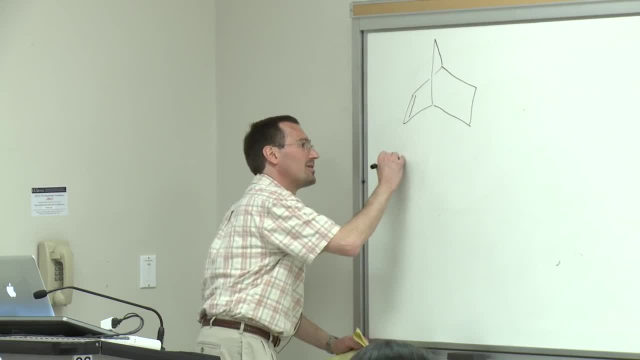 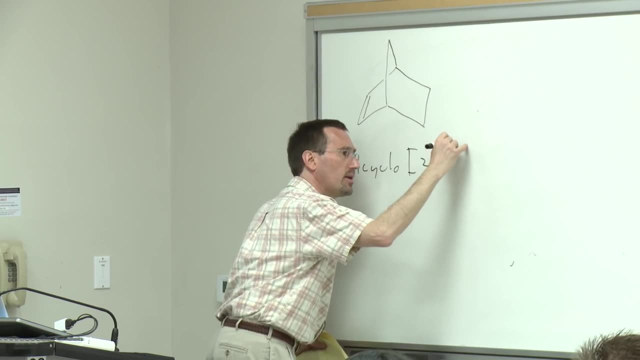 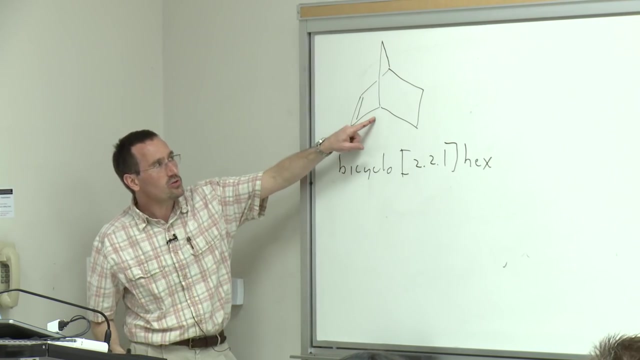 So bicyclo. so it's 7 atoms: bicyclo 2, 2, 1, hex. alright, And now we get to the numbering. So we've got two choices. Remember I said number the biggest bridge. 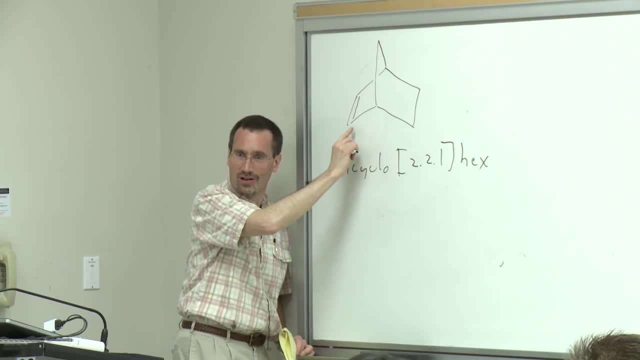 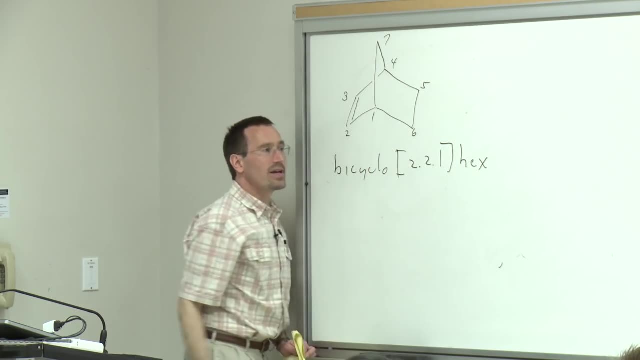 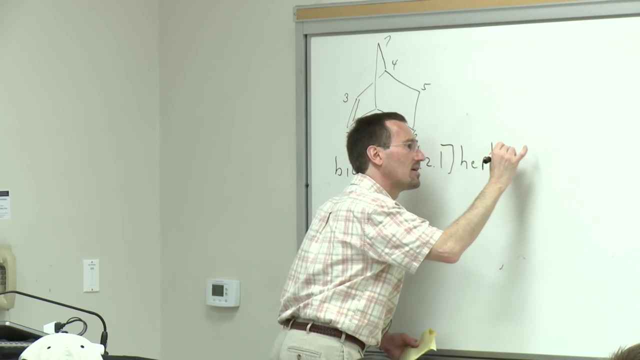 Well, we've got two choices. When all else is equal, we're going to give higher priority here, So it becomes bicyclo 2, 2, 1, hept- oops, did I say hex hept? 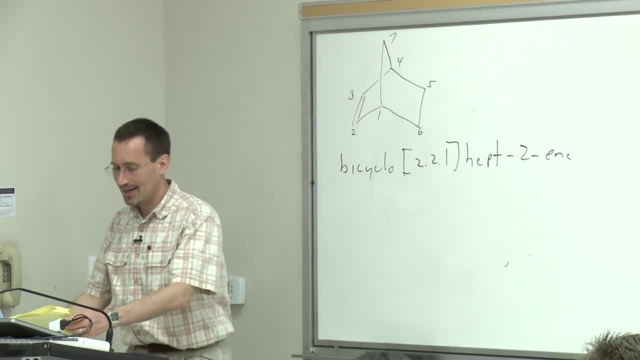 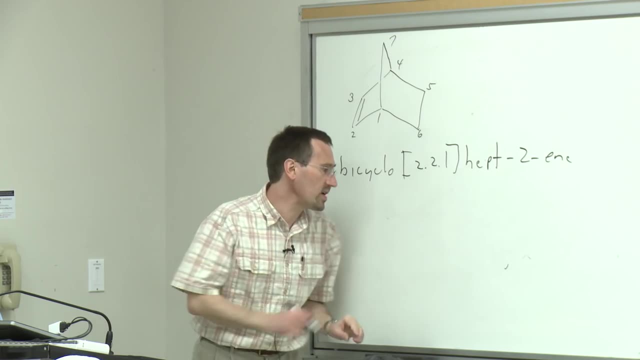 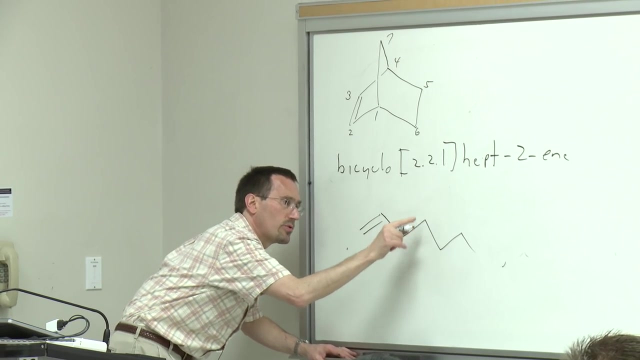 2-ene, Just like heptene, like when we say um this molecule, we can call this 1,, 2,, 3,, 4,, 5,, 6,, 7, we can call it hept-. 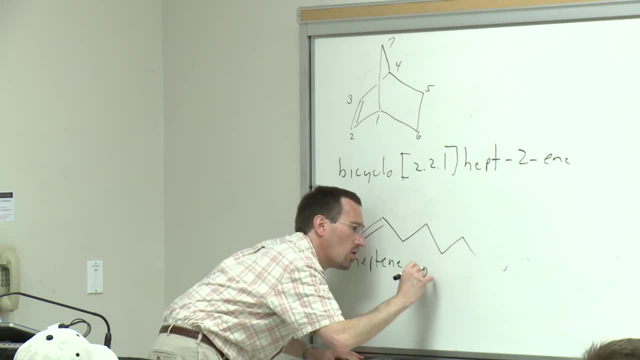 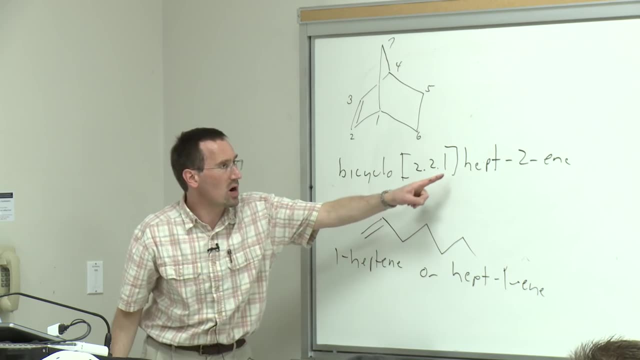 ene. we can call it either 1-heptene or hept- 1- ene, And I don't think it would be wrong to put the 2- here. I think there's enough freedom that you could call it bicyclo 2, 2,. 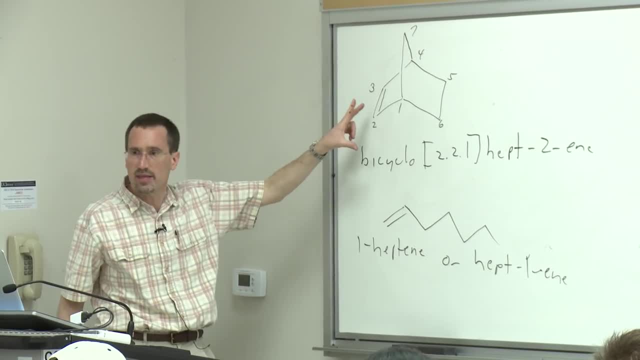 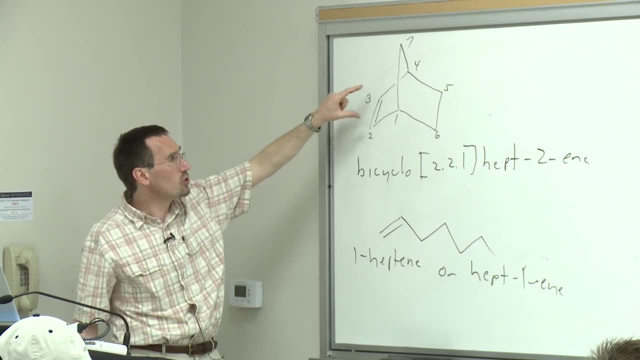 1-2-heptene Anyway, but you got the basic idea of it. It's still a bicyclic system. It's 7 now instead of 6.. 2, 2, 1. Thoughts questions. 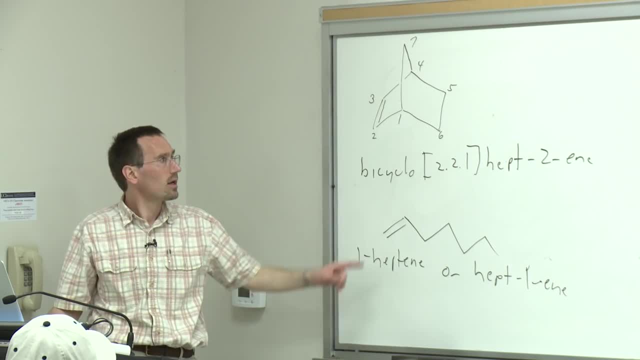 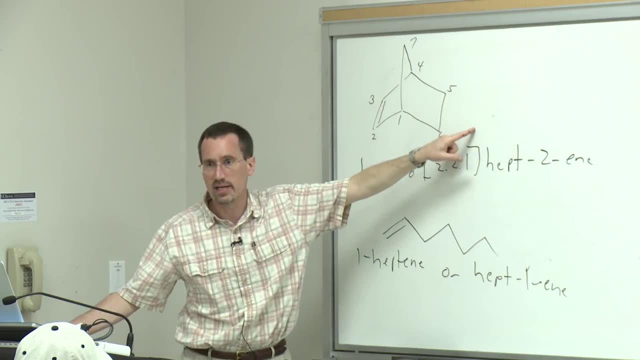 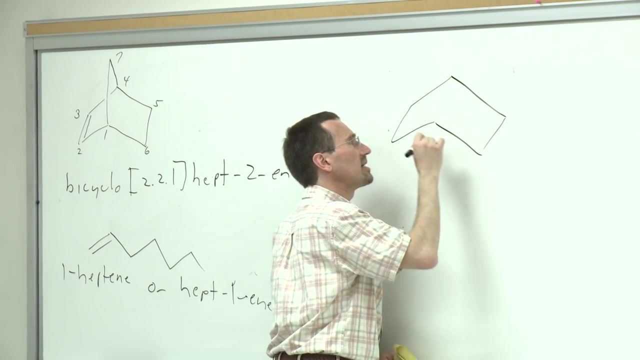 Yeah, Uh-huh. If it had been 3 carbons here, we wouldn't have been able to do it. We would have still had to number around this one. Now I want to show you one more set of variations, And we'll take the exact. 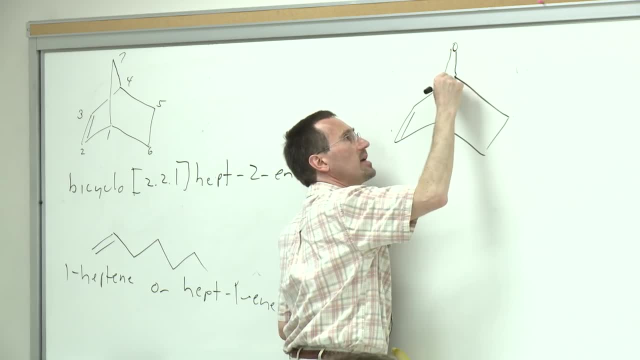 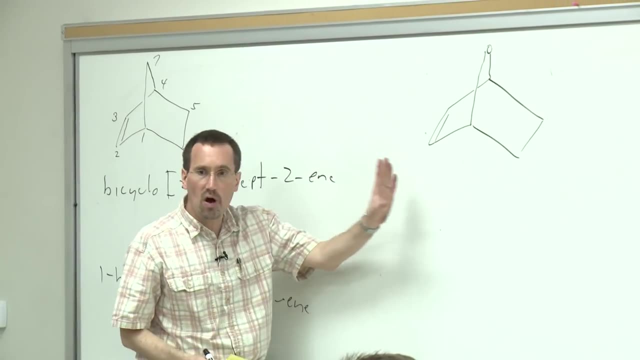 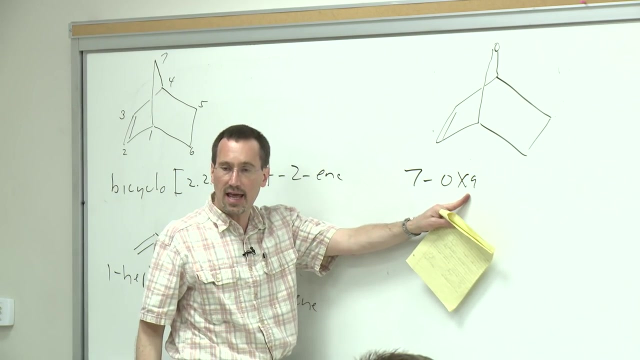 same molecule, except I'm going to put in an oxygen in the smallest bridge, And so now we go ahead. it's all the same principles, except now it is 7-oxa, So we use O-X-A not to be confused with. 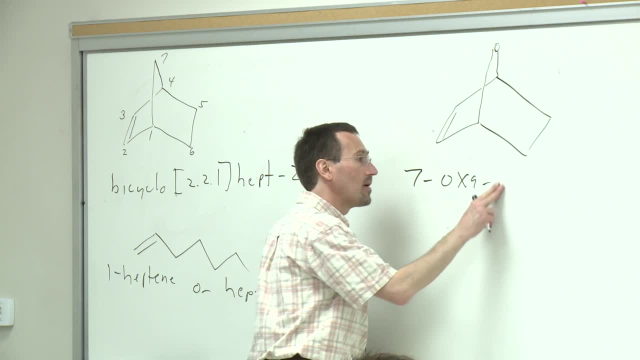 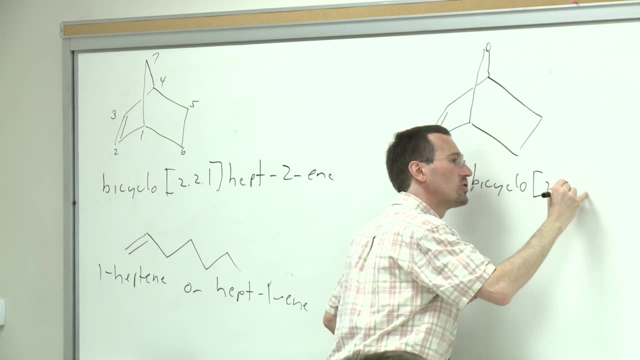 O-X-O and it becomes oops, no hyphen, and it becomes 2-2-1-glo- 2-2-1-hept-2-en, 2-2-1-hept-2-en. 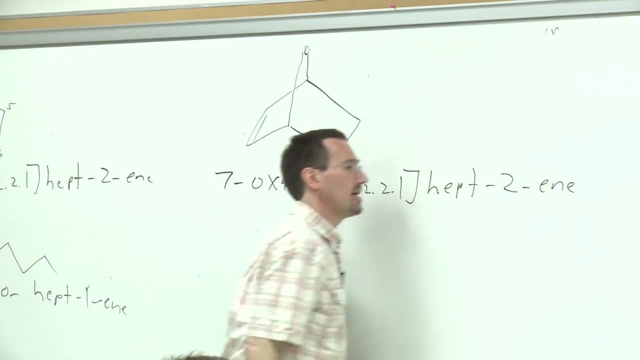 2-2-1-hept-2-en, 2-2-1-hept-2-en, 2-2-1-hept-2-en, 2-2-1-hept-2-en, And so oxygen. 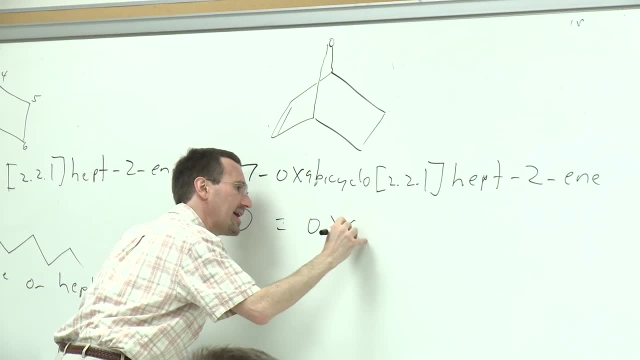 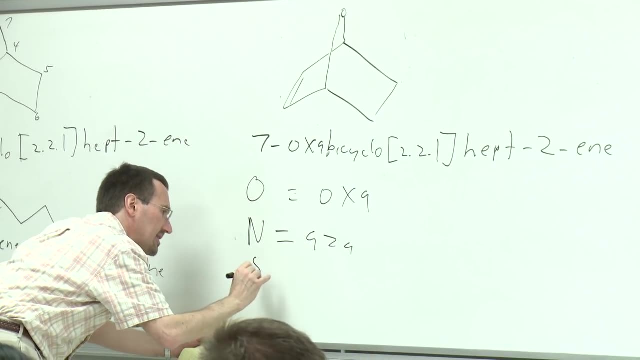 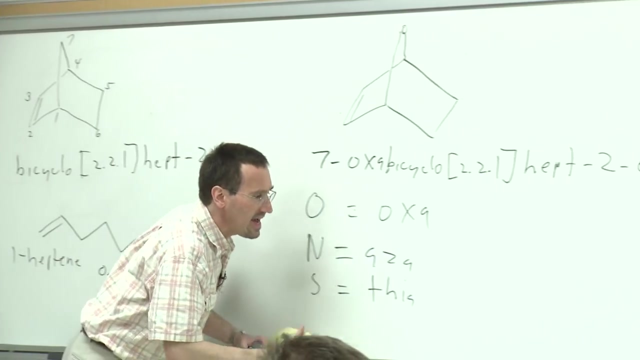 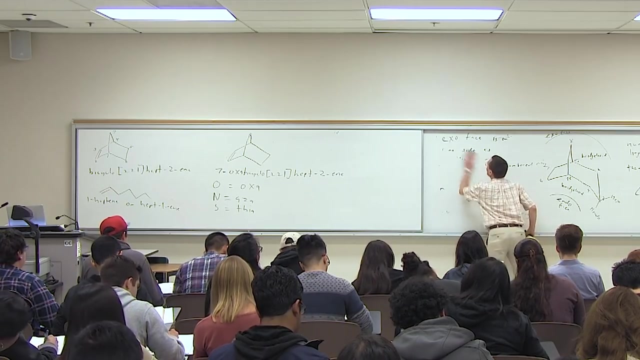 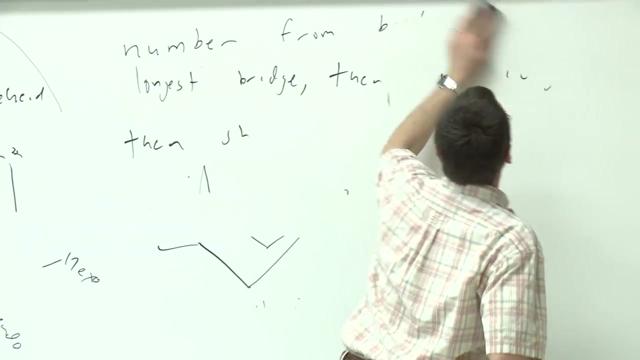 gets oxa, O-X-A, not to be confused with O-X-O, N gets aza and S gets thia. And again, these are terms that probably roll off the practicing organic chemist's tongue. Alright, I want to show you. 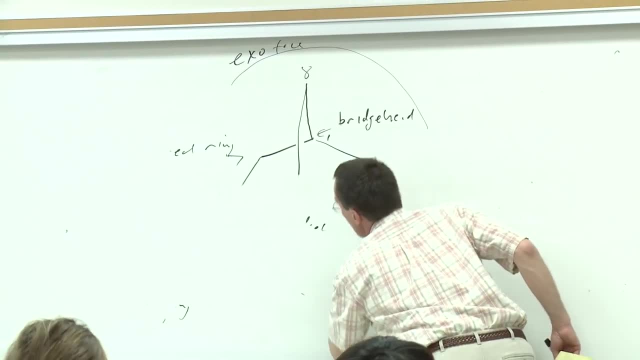 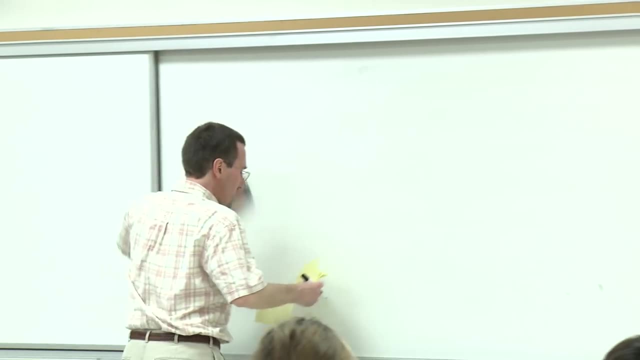 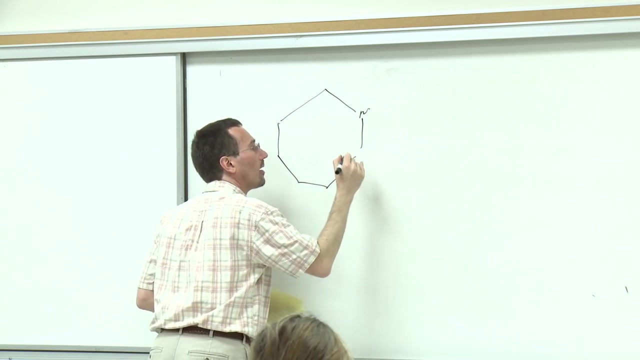 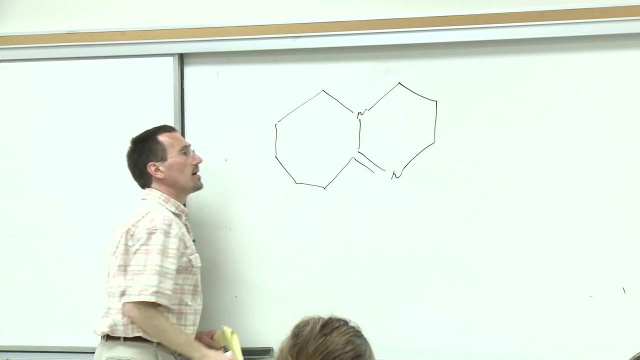 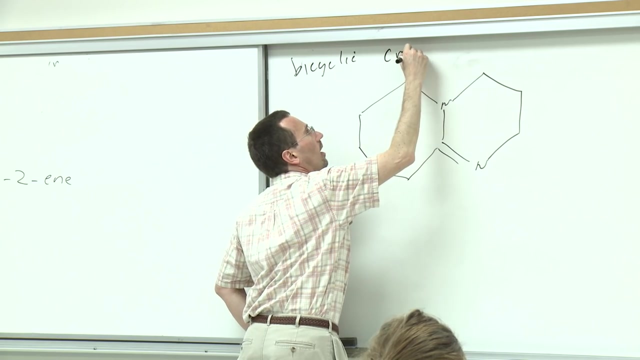 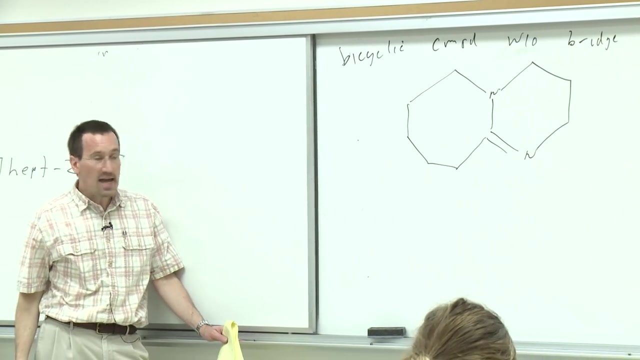 one last example. It's going to be a bicyclic where we have a no-bridge and we'll take all the ideas that we employed, Alright. So this is a bicyclic without a bridge. It's actually a common reagent. 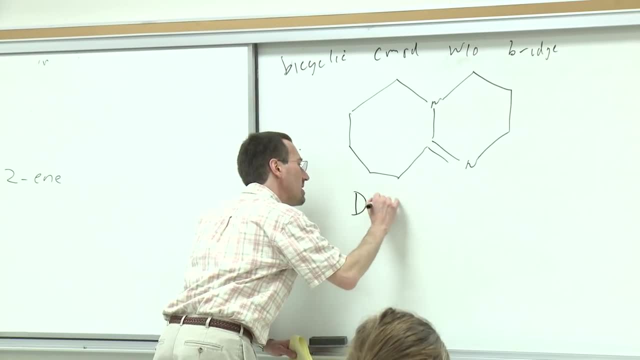 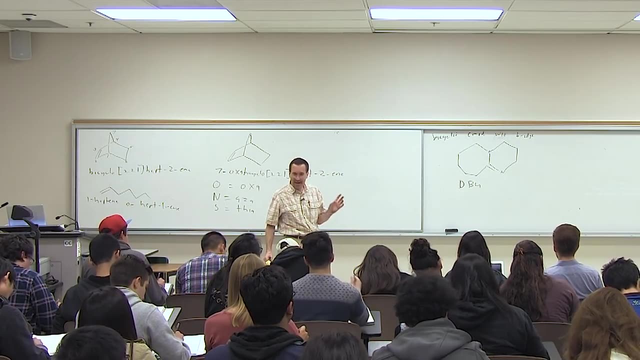 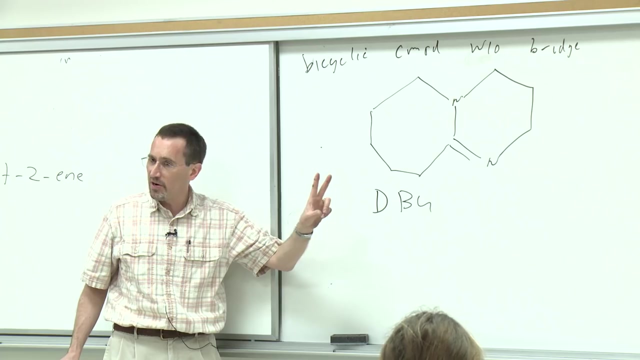 It's called D-B-U. It is an amidine. It is a strong base PK of the conjugate acid 13.5.. Really good for elimination reactions And all the principles we've learned can apply. It's got a five atom bridge. 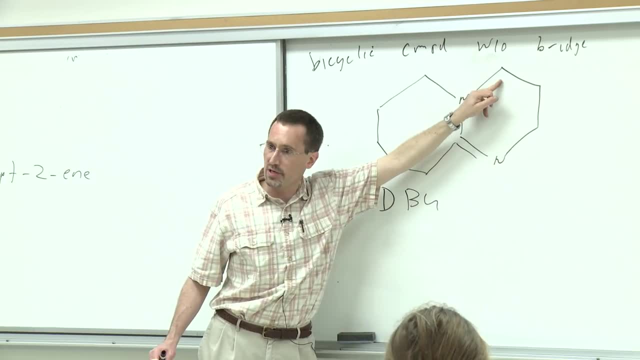 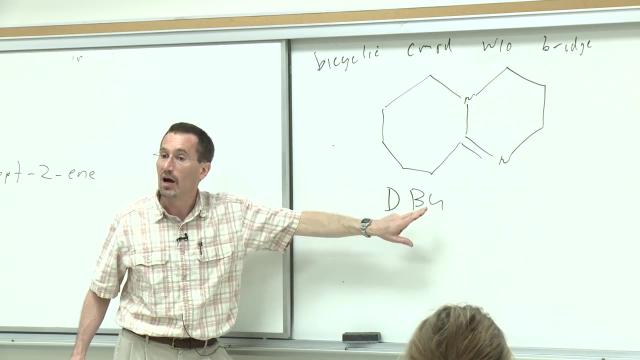 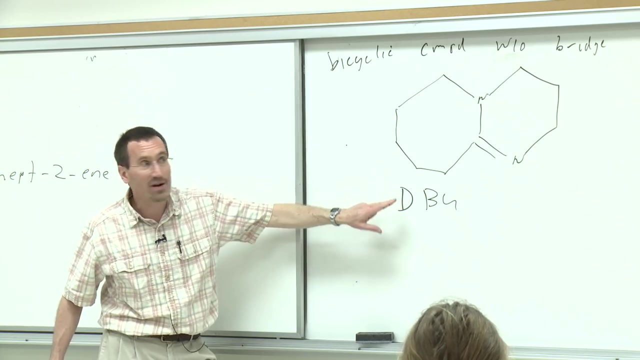 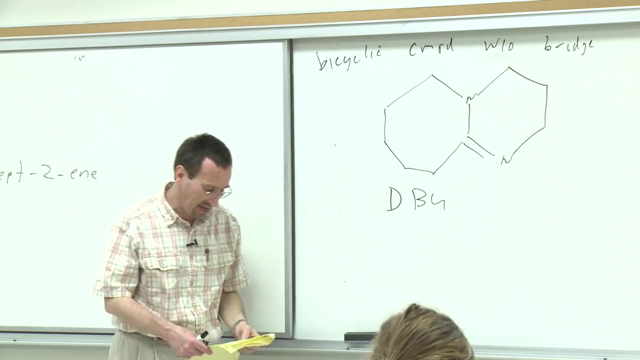 It's got a four atom bridge, It's a total of 11 atoms. The U stands for undecene, because we have a double bond, The D stands for diaza, because we have two nitrogens, And the B stands for bicyclo. 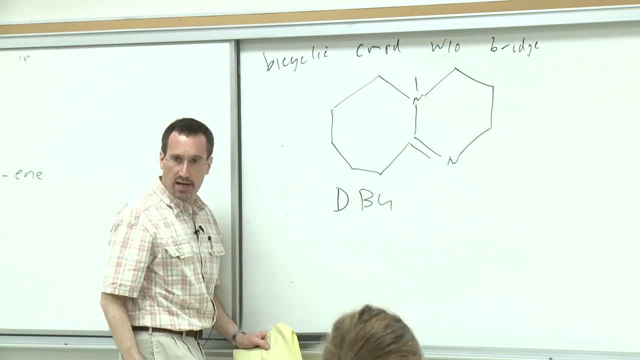 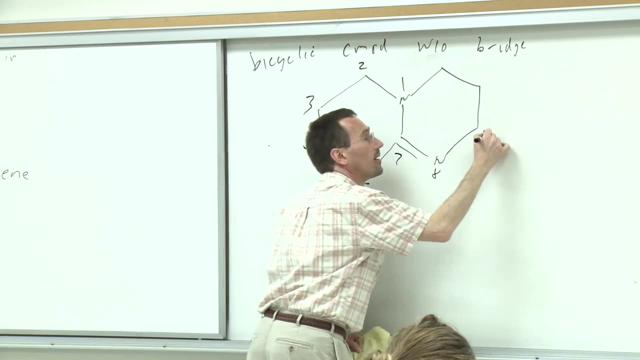 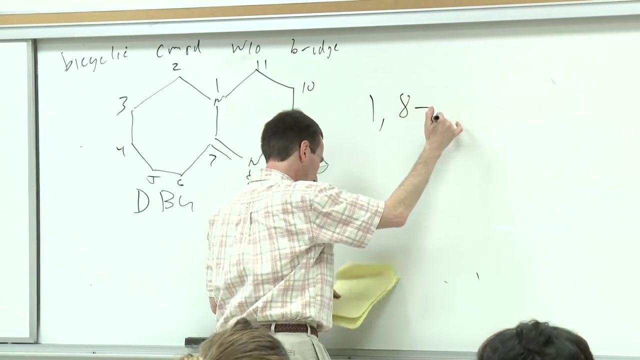 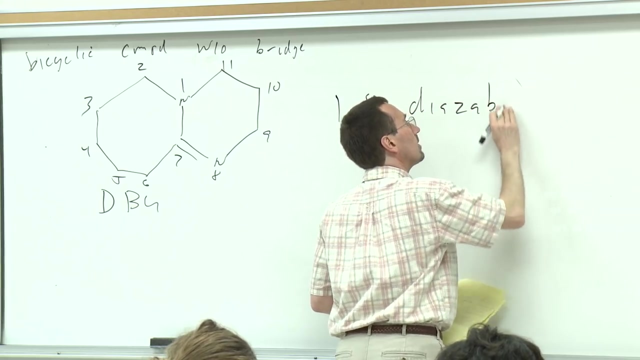 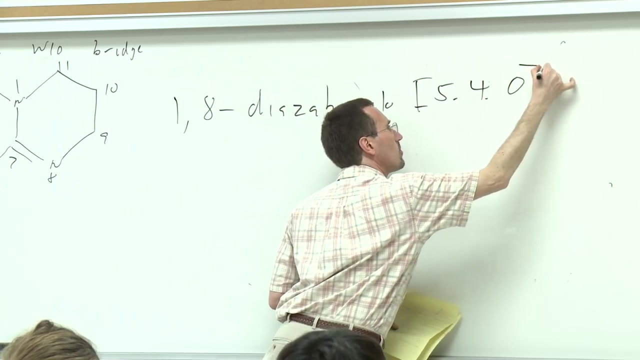 And again all the principles apply. We start with the bridge head number, the biggest ring and and its name becomes 18 diaza bicyclo 5, 4, 0, because we have a zero atom long bridge Undecene 7. 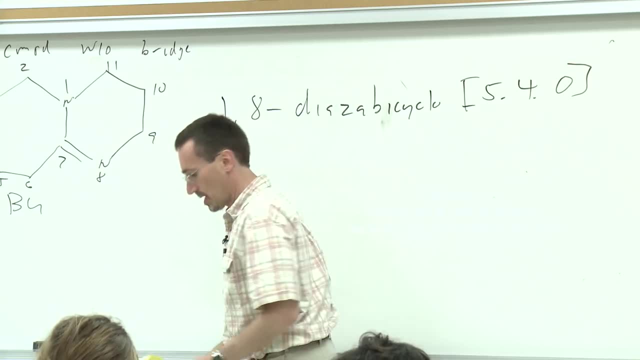 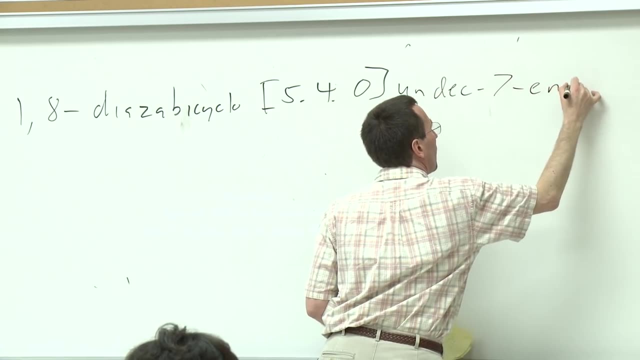 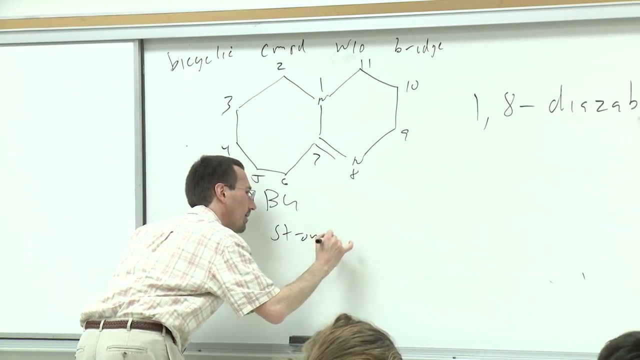 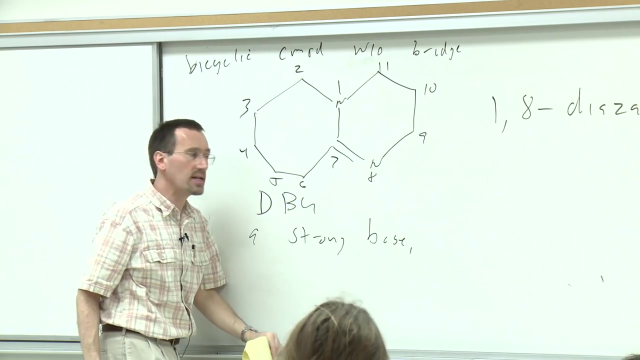 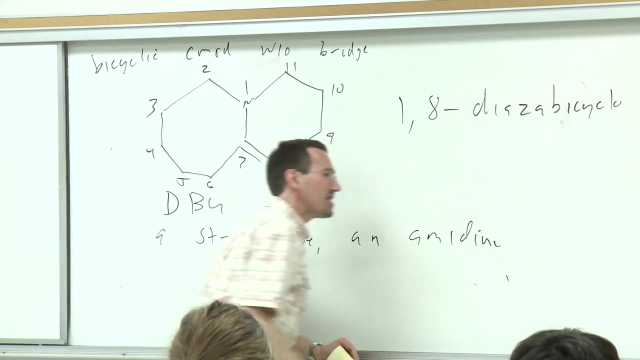 0, because we have a long bridge And the D stands for amine, And so it's a strong base. The class of compounds where you have a nitrogen and another nitrogen together is called an amidine. Alright, This is a very good. 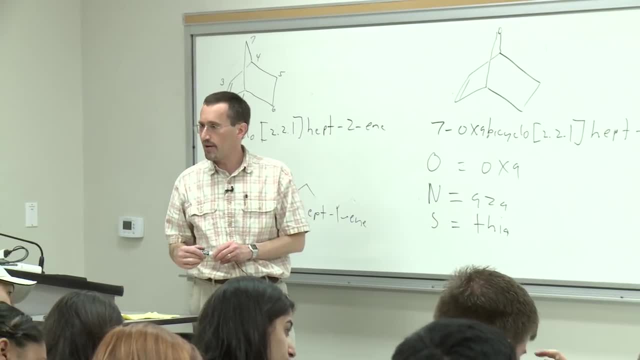 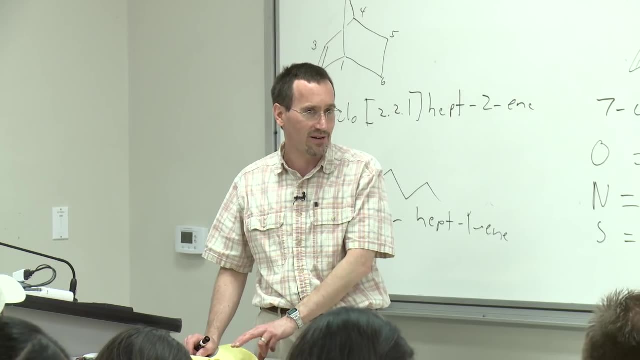 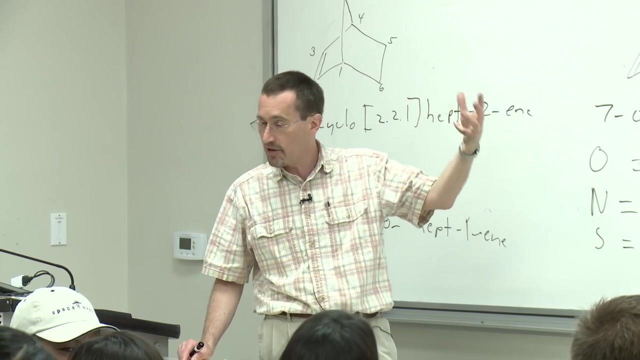 stopping point for today. The sorts of molecules that we're seeing here are the sorts of molecules that get me excited about organic chemistry, because they're pretty, they're complex and they show a whole bunch of ideas about how carbon and other atoms, nitrogen, oxygen and sulfur 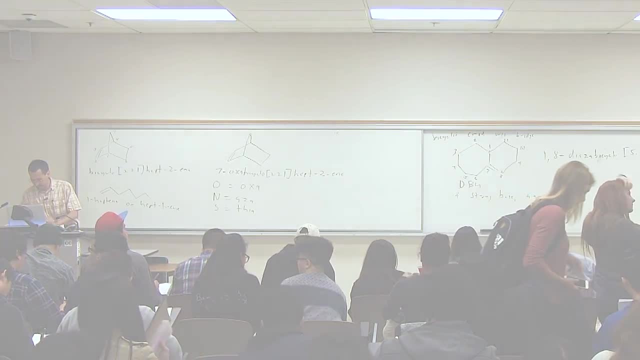 can be put together in myriad ways. See you on Wednesday. Captions by GetTranscribedcom. 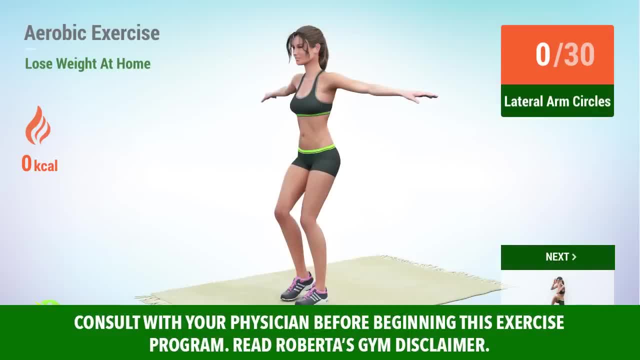 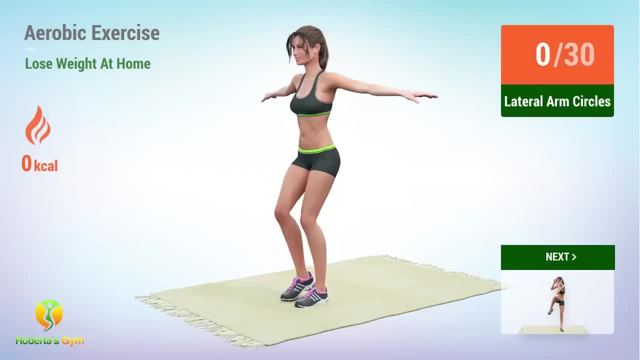 Up next lateral arm circles in 5,, 4,, 3,, 2,, 1, go 1,, 2,, 3,, 4,, 5,, 6,, 7,, 8,, 9,, 10,, 11,, 12,, 13,, 14,, 15,, 16,. 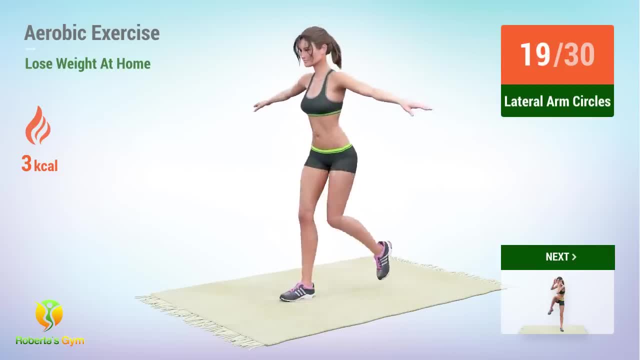 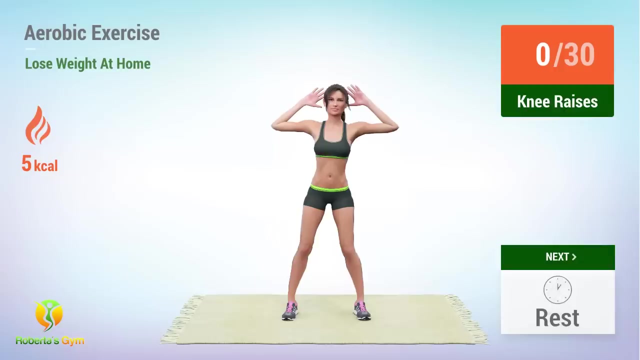 17,, 18,, 19,, 20,, 21,, 22,, 23,, 24,, 25,, 26,, 27,, 28,, 29,, 30.. Up next knee raises in 5,, 4,, 3,, 2,, 1, go. 1, 2, 3.. 1, 2,, 3,, 4,, 5,, 6,, 7,, 8,, 9,, 10,, 11,, 12,, 13,, 14,, 15,, 16,, 17,, 18,, 19,, 20,, 21,, 22,, 23,, 24,, 25,, 26,, 27,, 28,, 29,, 30. 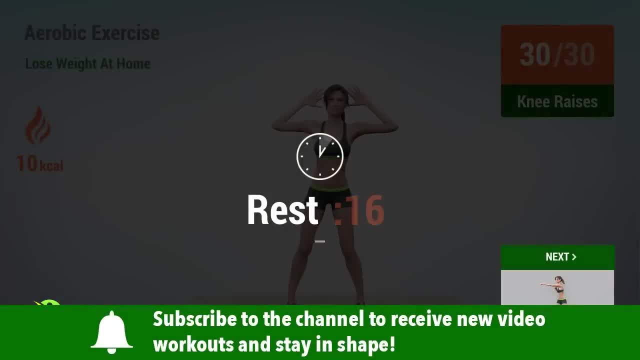 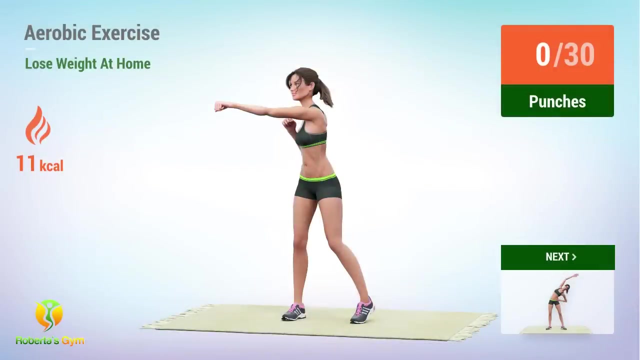 Rest time. Up next budgeteehands on knee families. Up next grab the wristband stand. 1,, 2,, 3,, 4,, 5,, 6,, 7,, 8,, 9,, 10,, 11,, 12,, 13,, 19,, 20,, 21,, 22,, 23,, 23,, 24,, 25,, 26,, 27,, 28,, 39,, 31,, 32,, 33,, 34,, 35,, 36,ut festival night.